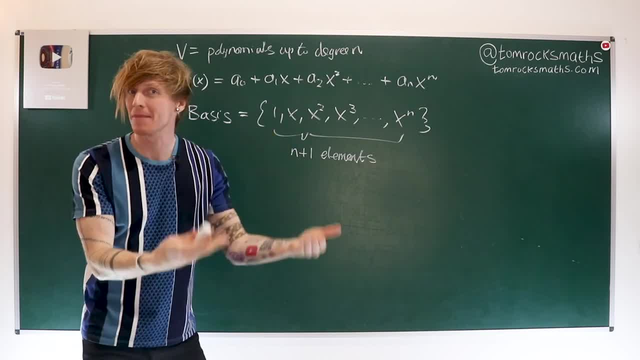 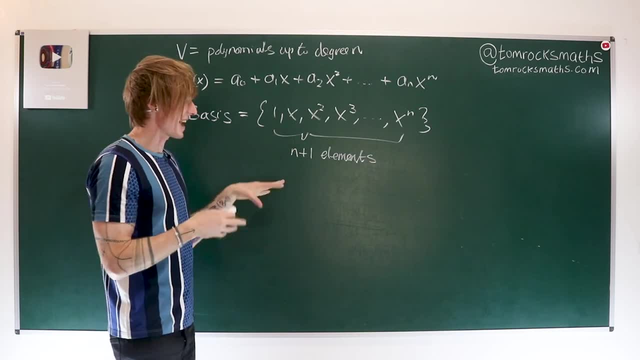 and therefore, according to our definition of dimension, which I just told you, is simply the number of elements in the basis. So if we look at our definition of dimension, which I just told you is simply the number of elements in the basis, Then we can say the dimension. 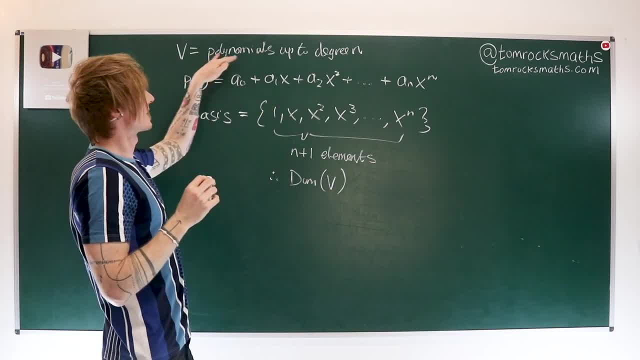 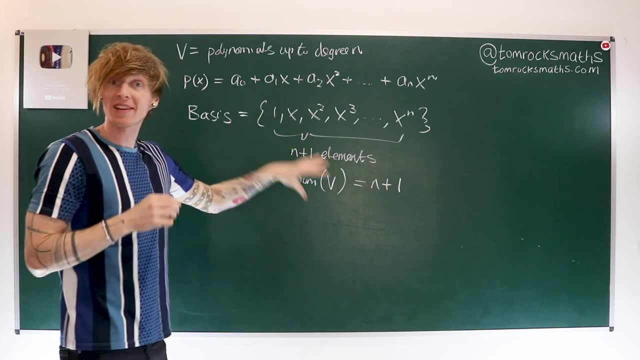 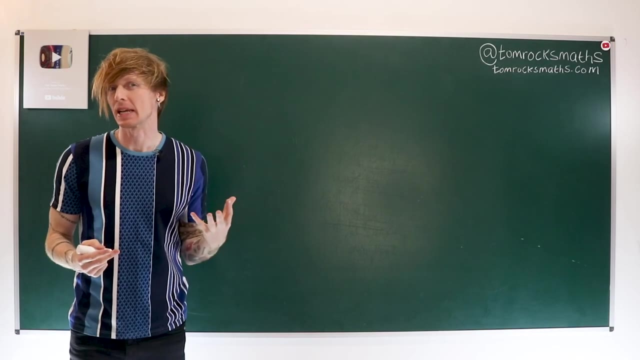 dimension of v. where v is the vector space of polynomials up to degree n, dimension of this space is n plus 1.. Again, because there are exactly n plus 1 elements in the basis. Now how about something a little more explicit? So let's take our vector space v to be r4. 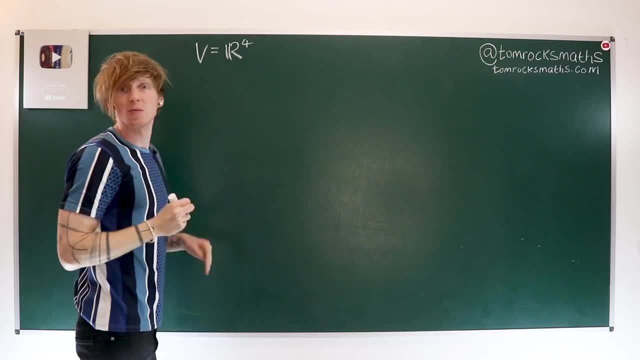 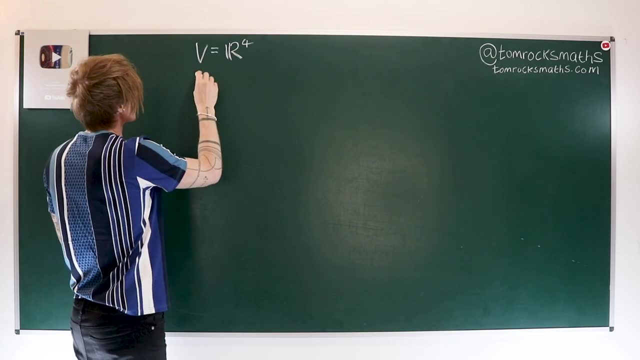 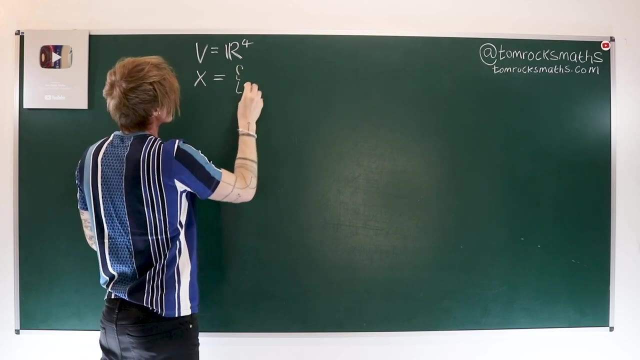 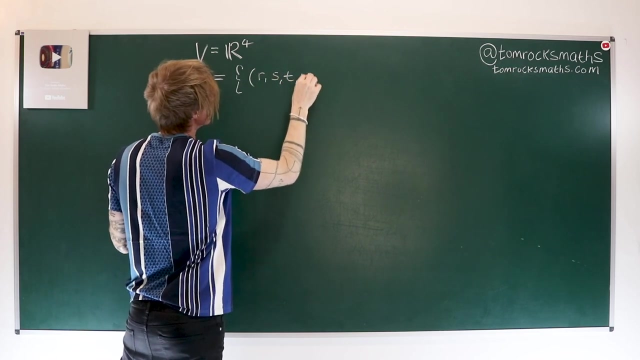 so this is all vectors with four entries, or four dimensional space, if you prefer to think of it that way. And let's suppose we have a subspace x, where x again consists of four vectors. So we could say: x is the set of, let's call these: r, s, t and u are our four entries. but in order to be in this subspace x, 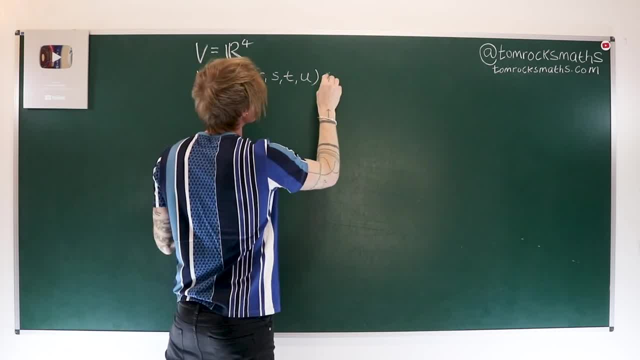 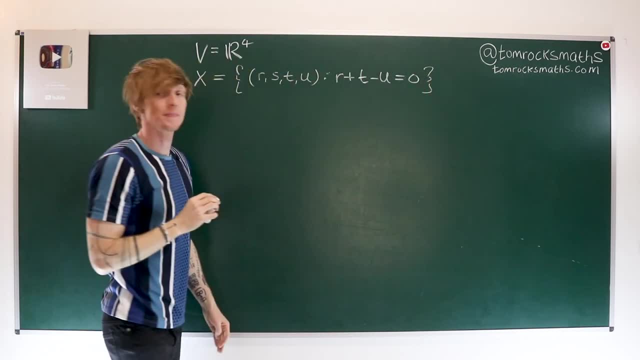 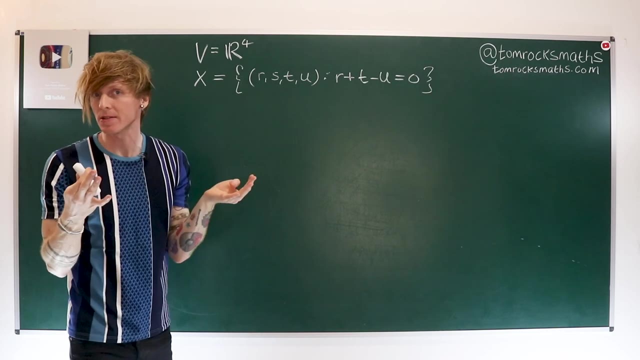 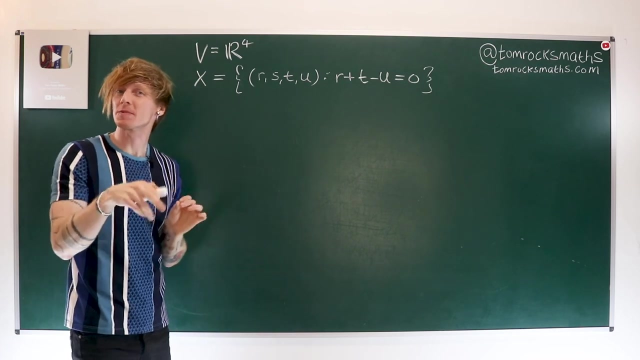 we're going to require that r plus t minus u is equal to 0.. So our larger space v is all of four dimensional space, four d vectors or vectors with four entries, and our subspace x, and of course you can check this is a subspace using the subspace test discussed in an earlier video in the Oxford. 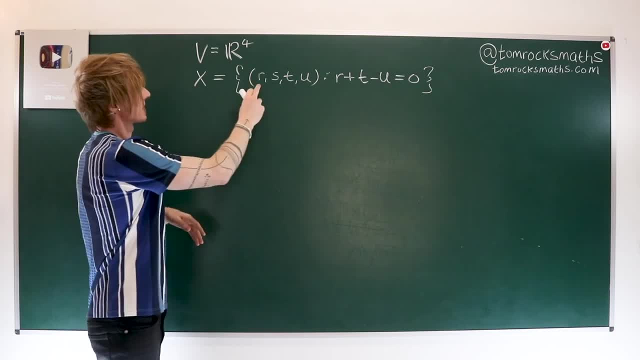 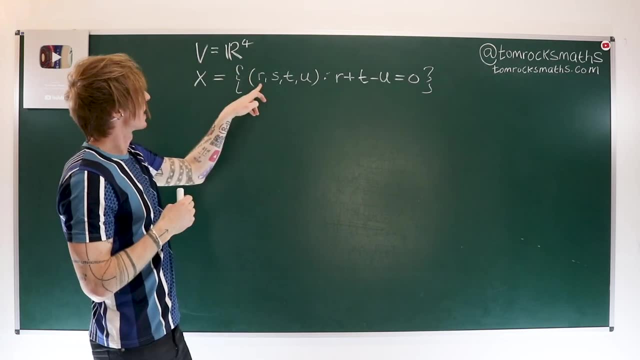 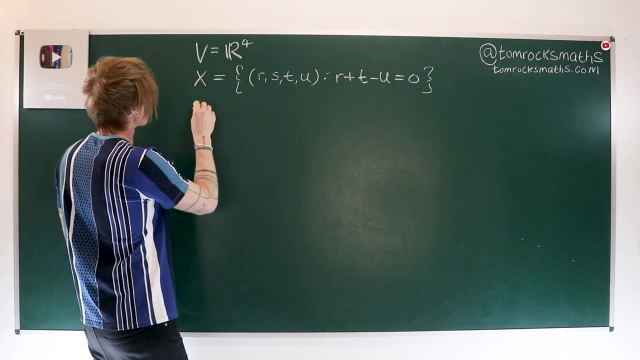 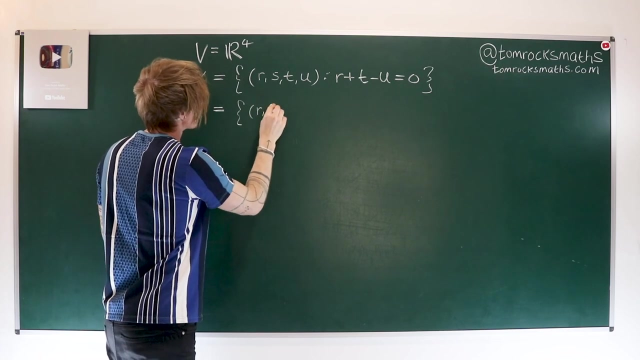 Linear Algebra series x is a subspace and it consists of four dimensional vectors, but they must satisfy this condition. So this is saying the first entry plus the third minus the fourth must always be zero. And we're also going to consider another subspace, y, where y again consists of four vectors. 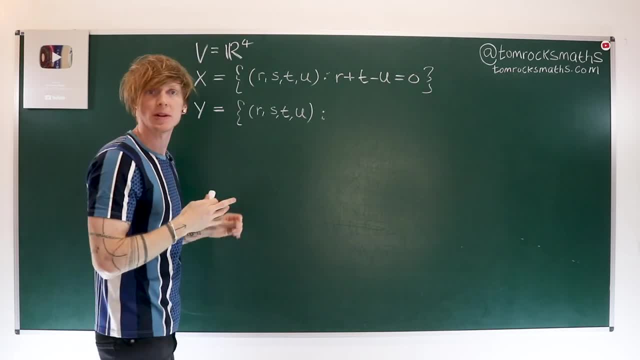 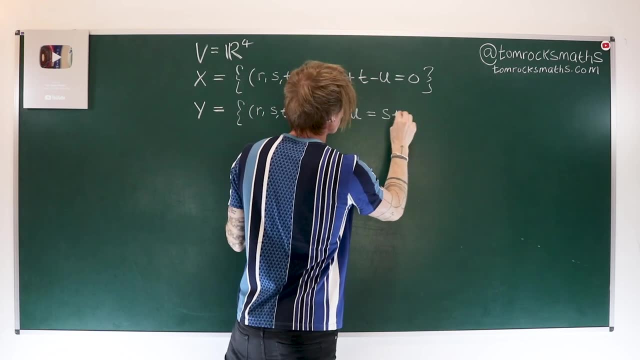 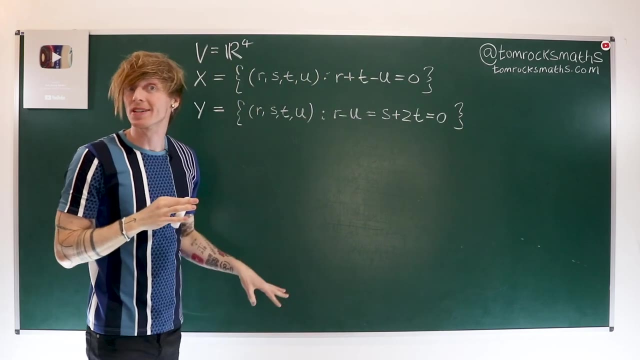 but this time there's a different condition on those entries, and this one is going to be that r minus u is going to be equal to s plus 2t, and both of those are going to be zero. So now we have two separate conditions that have to be satisfied by the four entries. 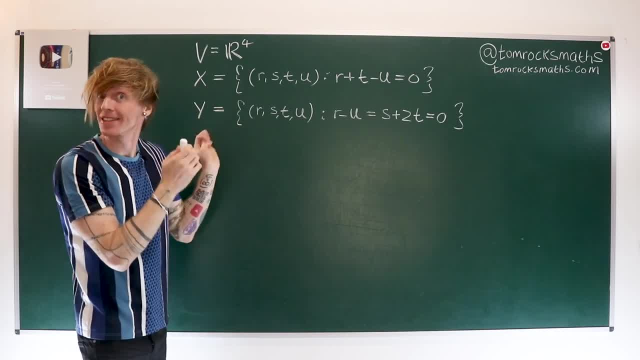 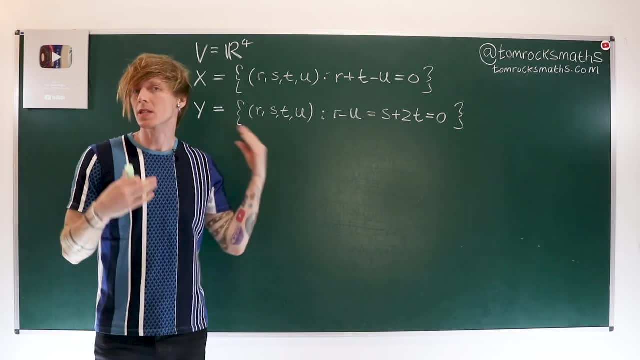 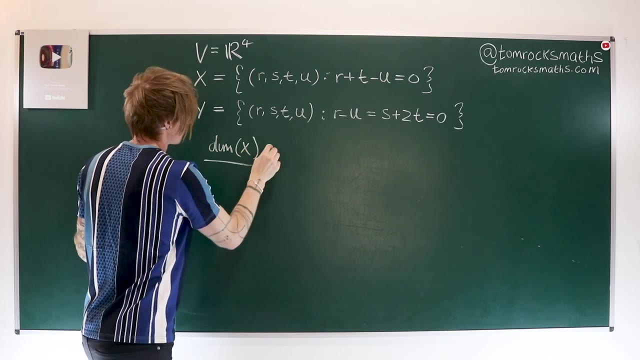 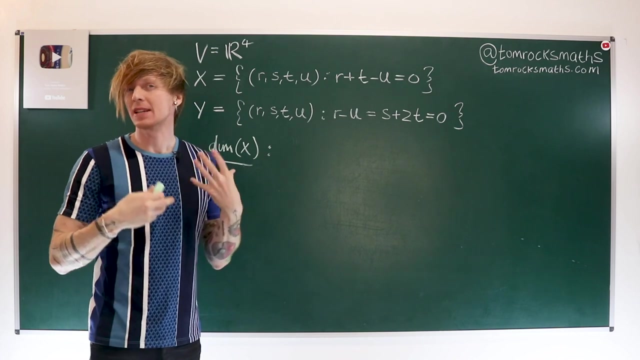 in order to belong to the subspace- and again, you can check this exercise for the viewer- the subspace y. So let's start by thinking about the dimension of the subspace x. So dim of x. Now, when it comes to calculating dimensions, something that I find particularly helpful, 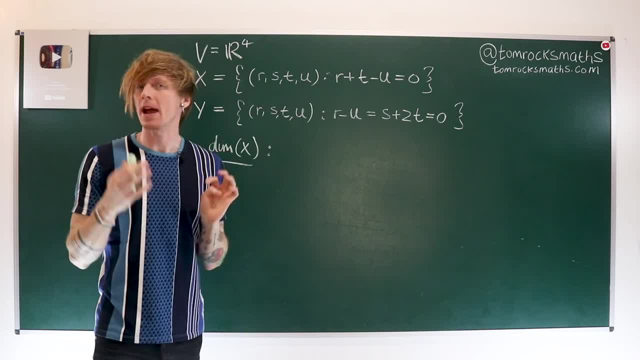 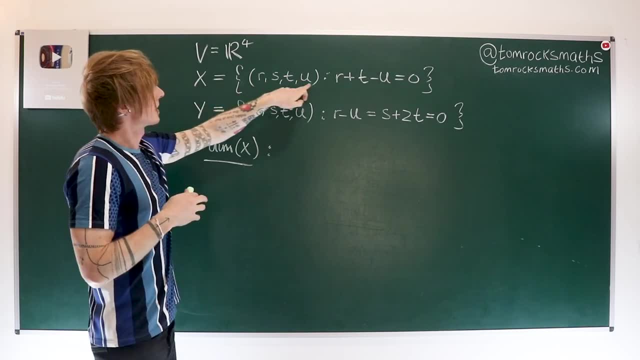 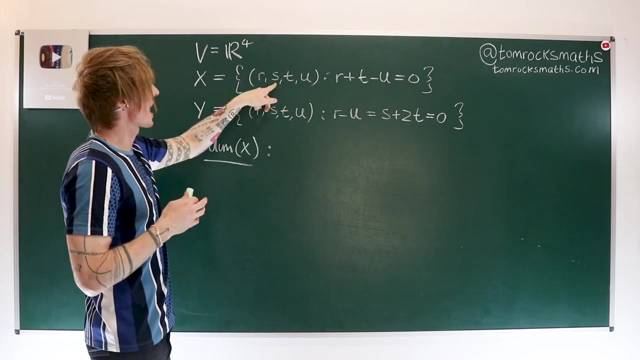 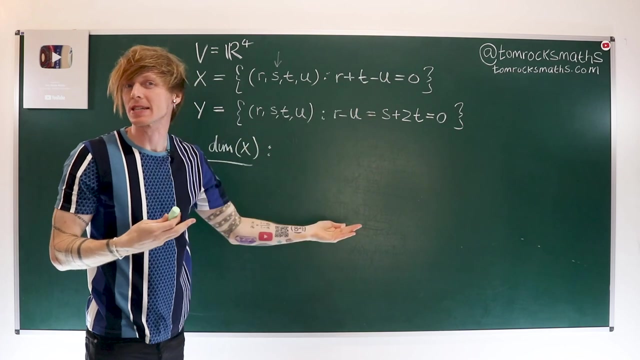 is to think about the possible free variables that you have in your system, And what I mean by this. for example, is we looking at x? we don't have any condition on s, So the entry here, this entry here, it isn't mentioned in this particular condition or this constraint. 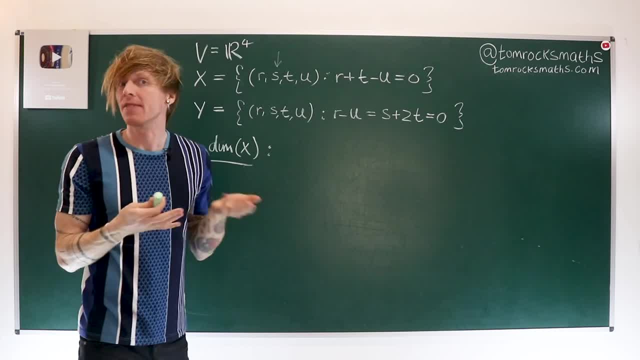 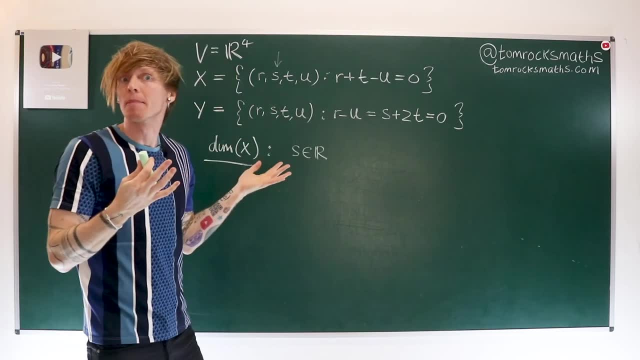 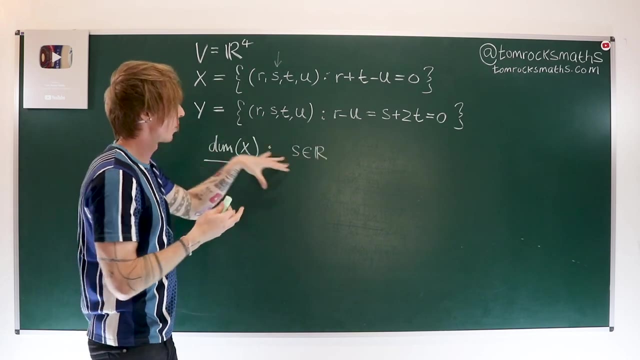 on our variables. So s can clearly be any value. So immediately we can say: well, s can just be any real number, because we're working in r4. So there's no restriction on s. so we sort of have all of the second dimension. we have all of that that we want. 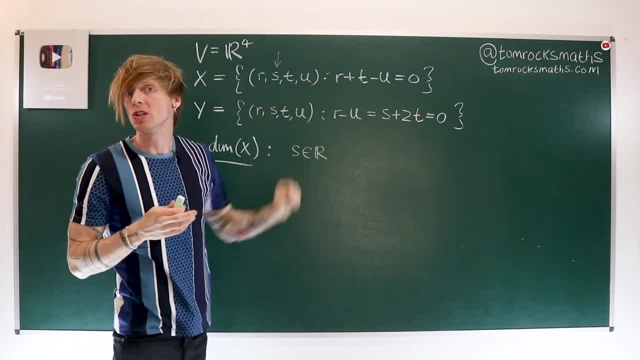 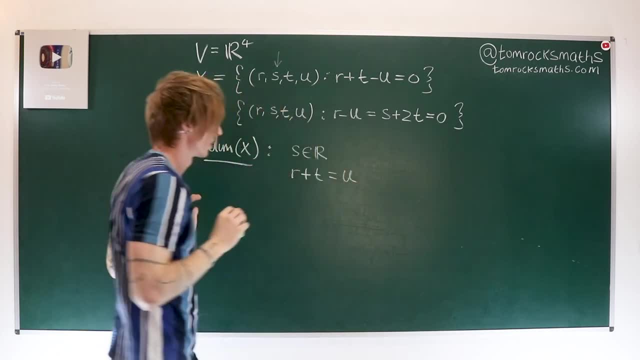 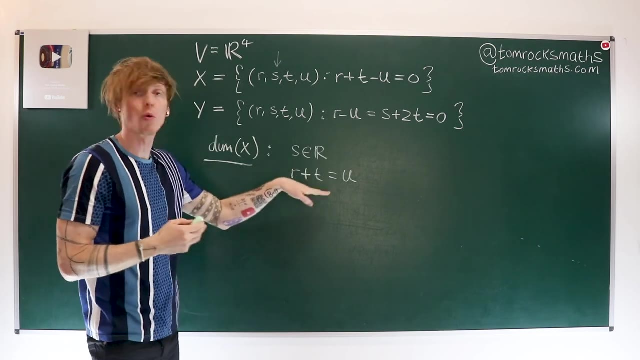 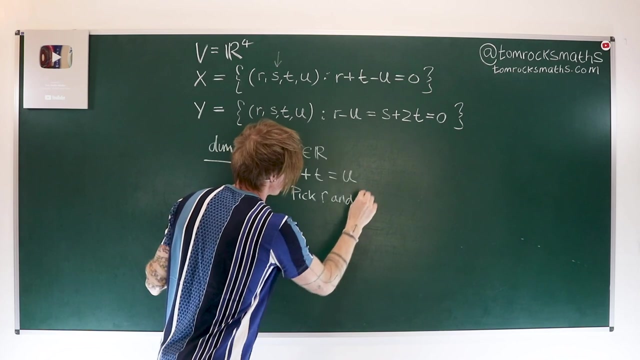 Now here we have a condition on rt and u and we can actually rewrite that and say: this tells us that r plus t is equal to u. So there are three things here, but we are not able to pick all three of them. So if I were to pick, for example, r and t, So I pick those values. and again, let's suppose 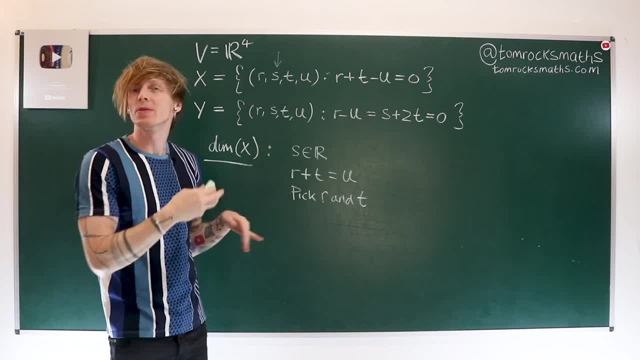 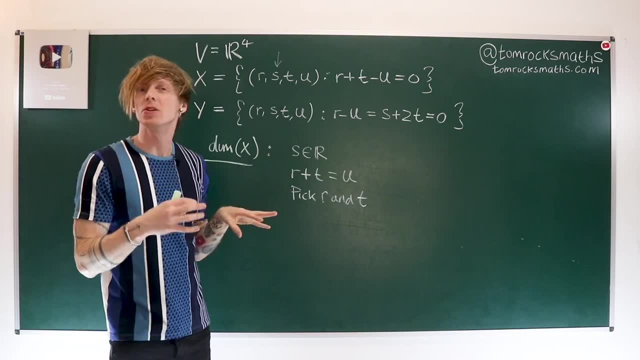 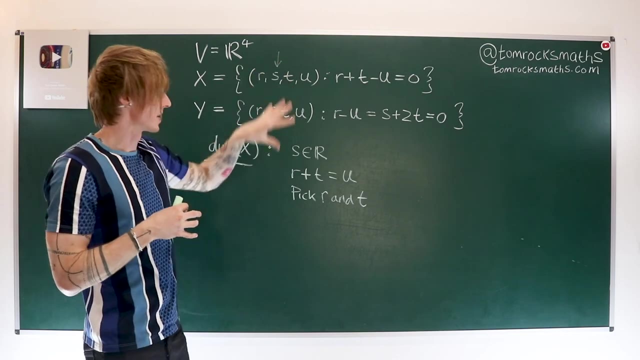 they can be anything I want. Then the value of u is automatically fixed. so we lose that freedom. So this condition on rt and u is actually removing one of our free variables from the four original ones that we started with. So this is a constraint. so in some sense it's like the number of free variables minus the number of. 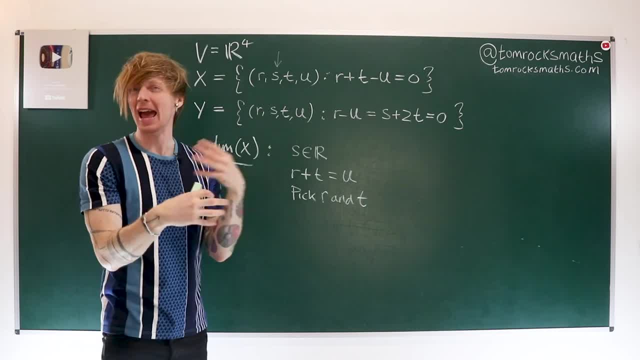 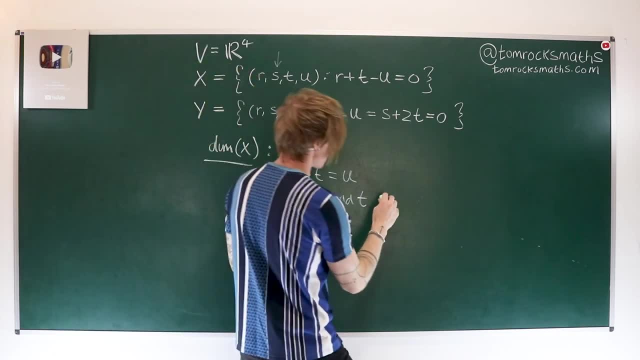 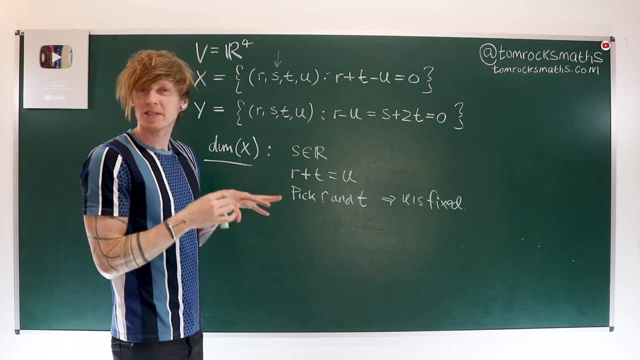 constraints is one way to think about or one way to help get some intuition for what's going on with dimension. So if we pick r and t, then that would imply that u is fixed. so we don't have a choice here. So this to me is suggesting we have a free variable here. we have a free variable here. 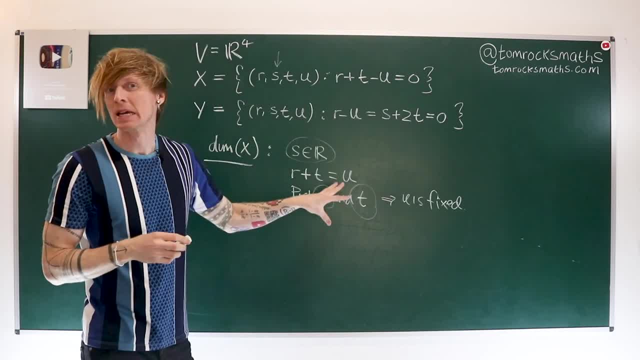 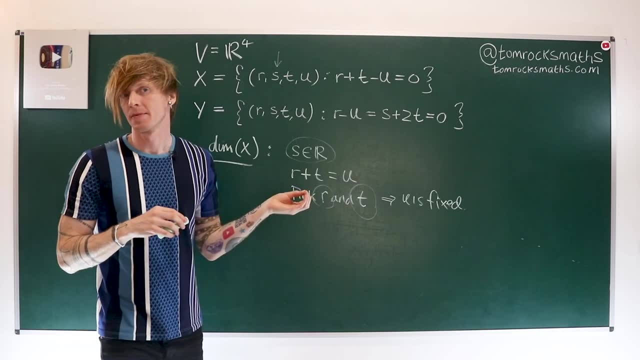 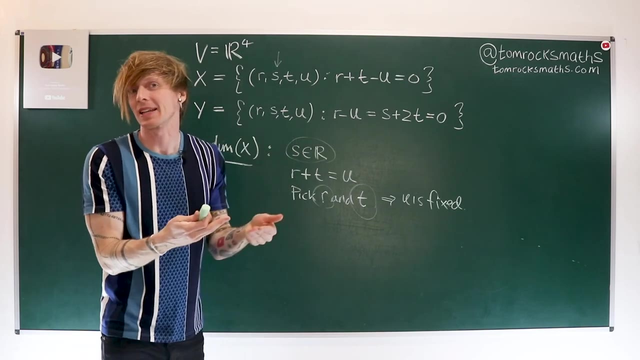 a free variable here, but u is going to be fixed once we pick those first three. So in that sense, I'm expecting the dimension to be three. but in order to prove that, or to show that formally, we need to write down a basis Which has exactly three elements, because, again, the dimension is the number of elements in the basis. 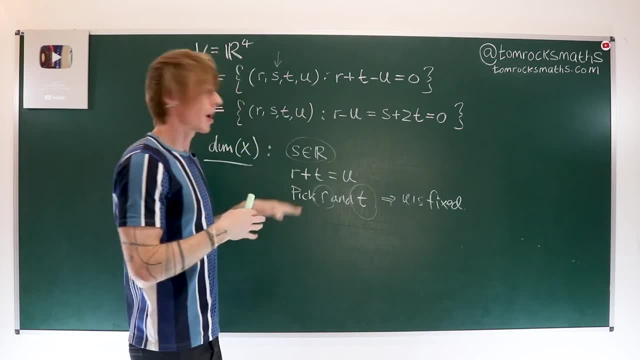 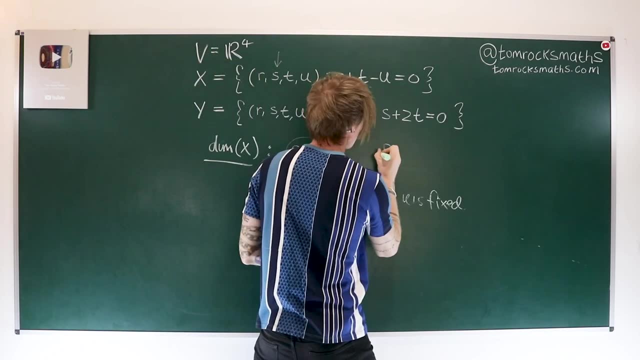 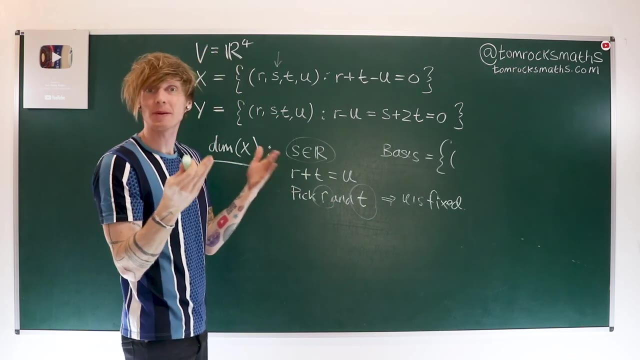 So let's try to construct a basis. So we start with the fact that s can be anything and it isn't mentioned in our constraint or our condition. So immediately we can say, if we want to try and write out a basis, then let's take everything else to be zero and s to be one. So zero, one, zero, zero. 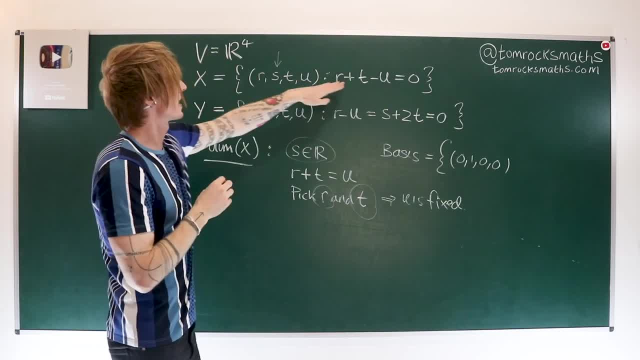 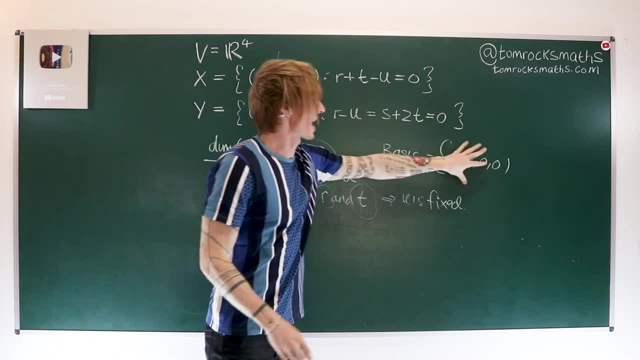 And we can see that that is a four vector which very clearly satisfies this result. r plus t minus u is naught naught. plus naught minus naught is still zero. So this allows us to get the whole of that second dimension. We just multiply this by any constant to get the whole of that dimension. 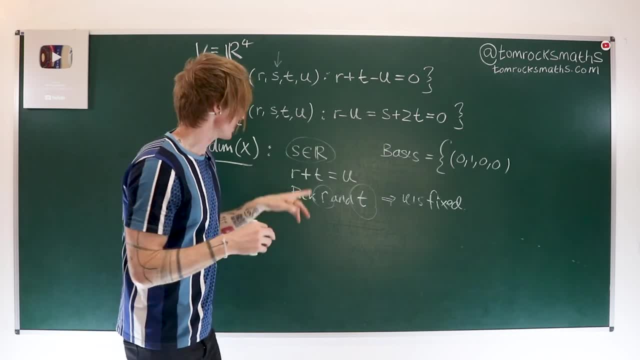 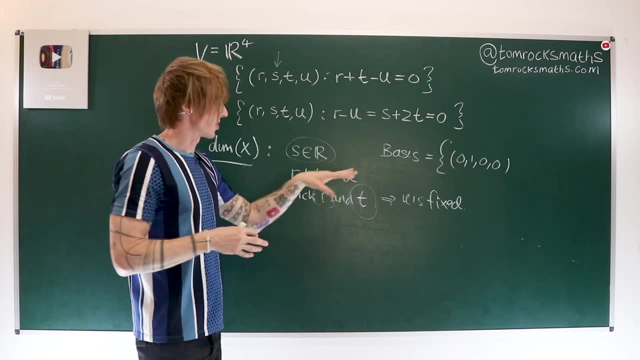 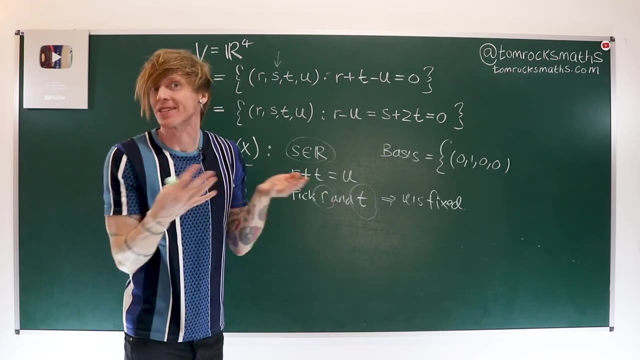 in s, as we were expecting. Now I'm saying here that we can pick r and t, but then u is going to be fixed, And the trick here to creating a basis is basically to make sure that we're going to get one of these zero and the other one- let's say one to keep things simple. So let's start by saying: 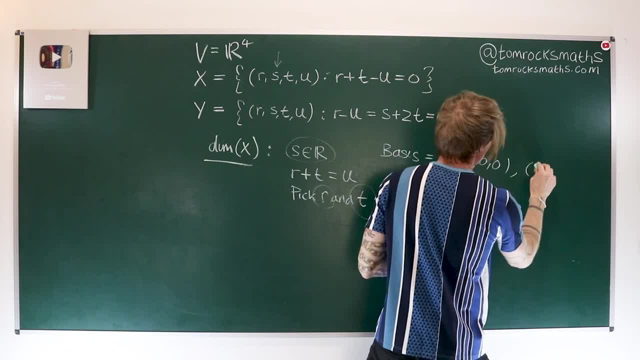 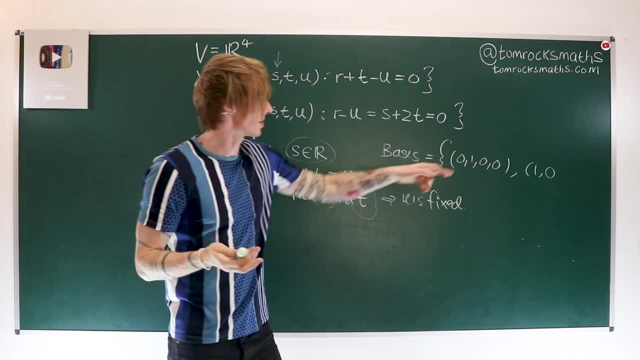 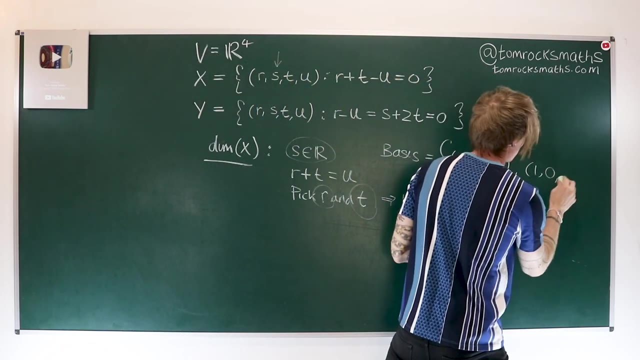 well, suppose r was one. so that's our first entry. Then s we can just write that as zero, it doesn't really matter, because we can always get whatever amount of s we want by adding a multiple of the first vector. Then we're going to say: suppose t is naught. and now our condition is going to: 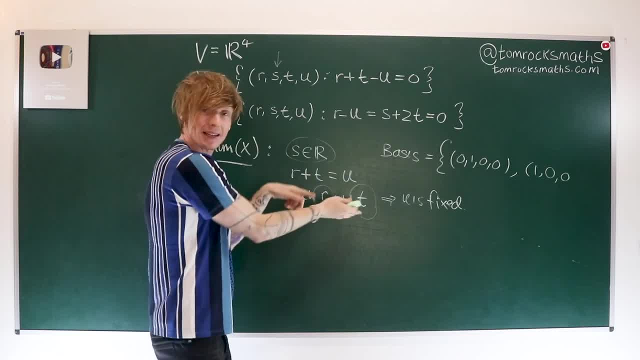 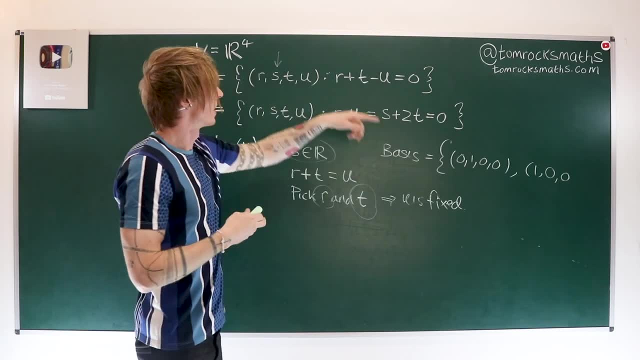 tell us what u has to be, Because we said here, so I picked our first vector and I'm going to write r and t, like I said was possible, and we need to now see what u is going to be fixed as according to this condition. So we've got: r is one, t is zero, so u has to be one as well. 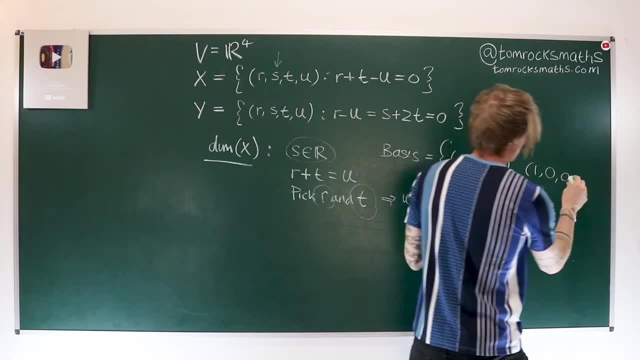 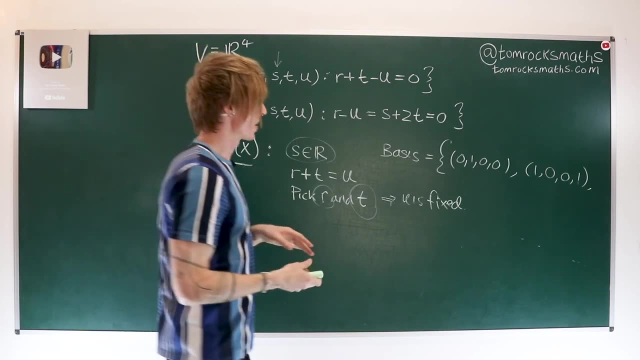 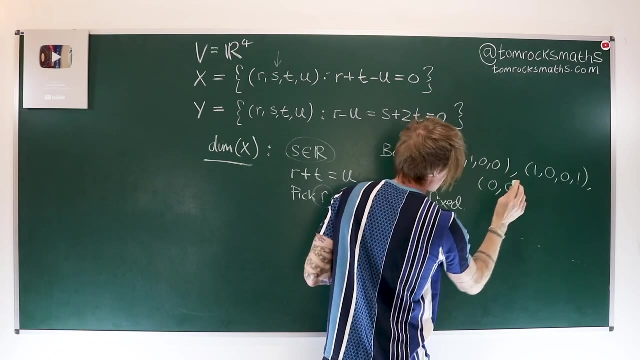 if we're going to satisfy the constraint. So we just need a one on the end. And now swapping the roles of r and t, so swapping the zero and the one we can get here. so we had r is now zero, s can stay as zero, t is one and again, to satisfy this, we're going to need u to be one. 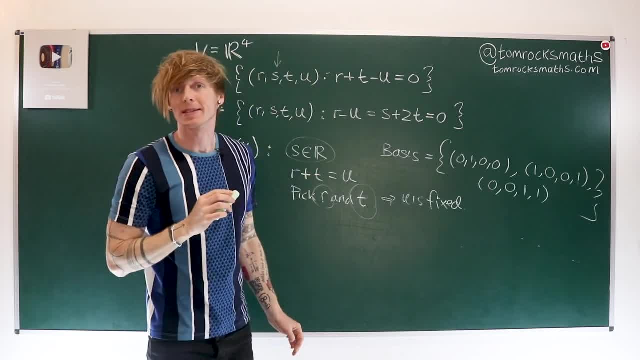 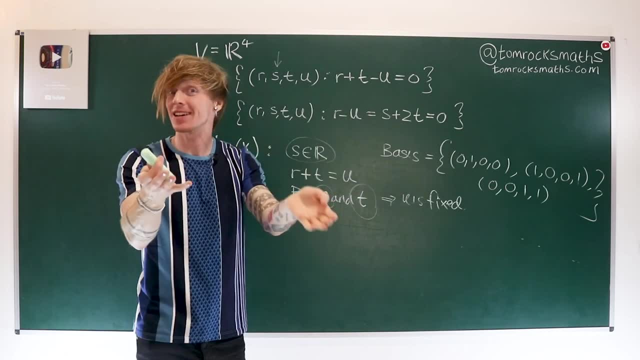 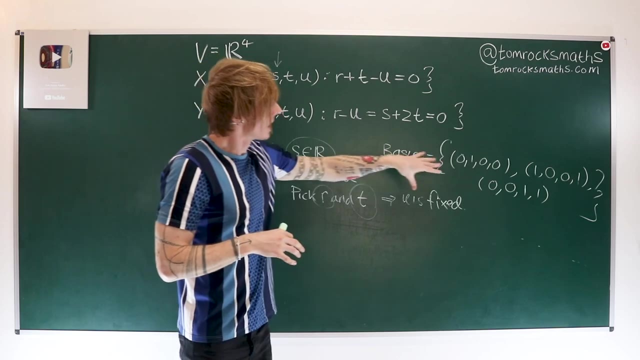 And I believe that is going to be our basis. Now I will not formally check that this is both spanning and linearly independent exercise to the viewer, because that's what we covered in the previous video in the Oxford linear algebra series, But the idea here of using zero and one for these two 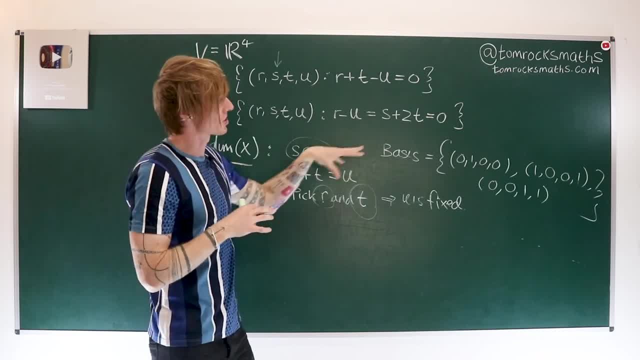 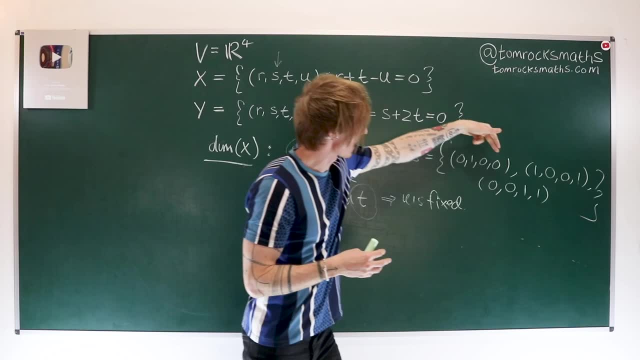 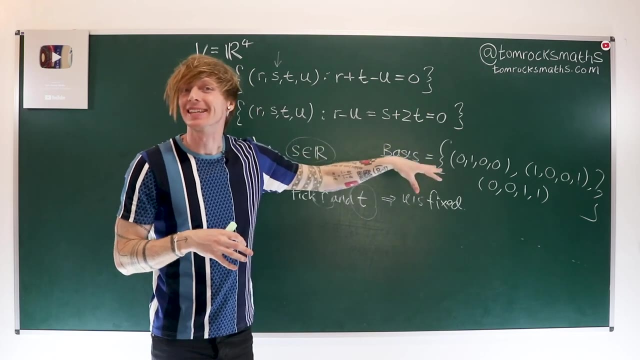 variables is very, very helpful Because it gives you something or a pair here which are quite clearly going to be linearly independent, at least as a pair, And again, because we have lots of zeros here, you can hopefully see that this will indeed be a linearly independent set. Of course, you still need to check that it's. 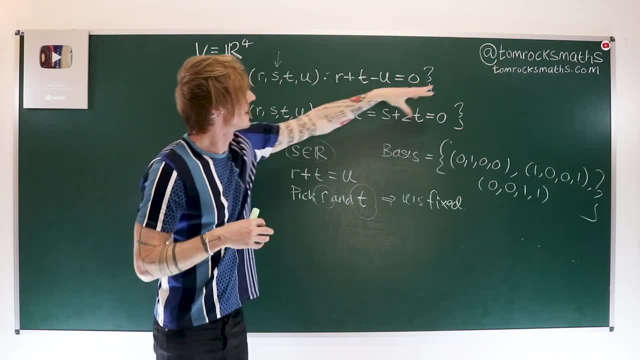 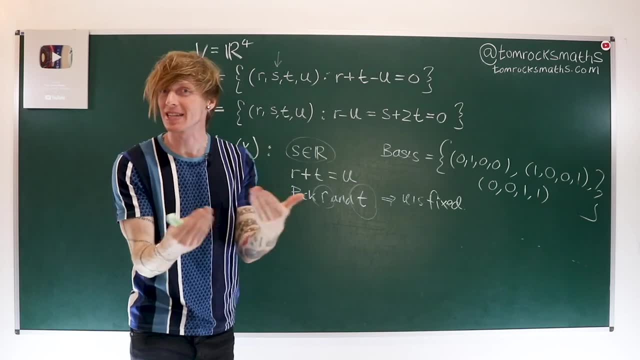 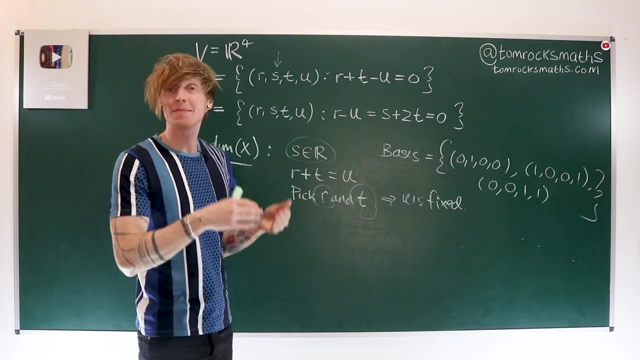 a spanning set as well. so you would need to take a general vector in our subspace x and show that it could be rewritten as a combination of these three. But again, you will see that that is indeed true. So this, I believe, is a correct basis and therefore our dimension as we expect it from. 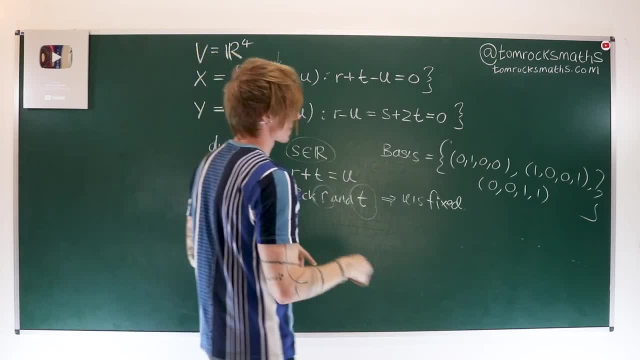 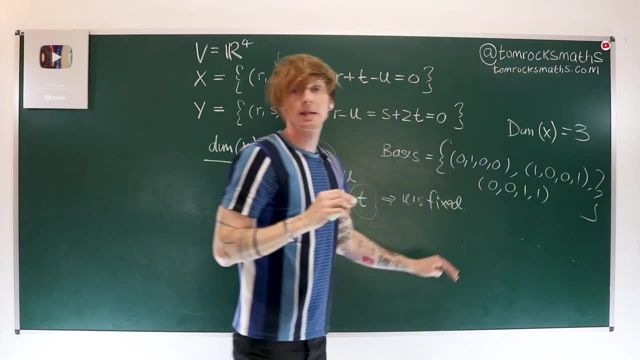 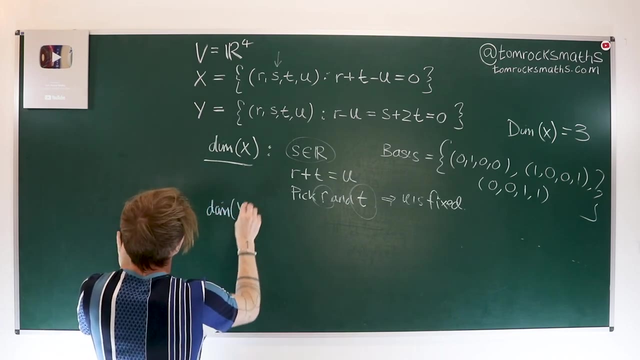 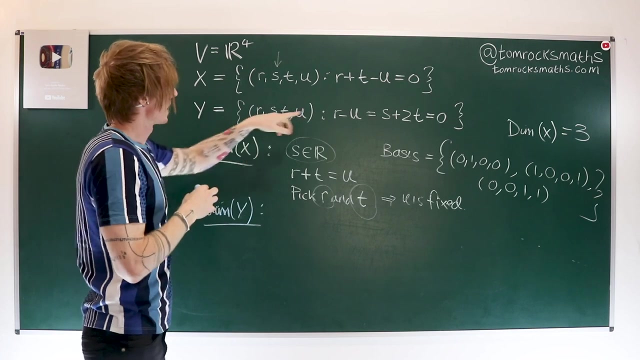 this earlier discussion is going to be three. So the dimension of x- let's write it over here- dim of x equals three. For our subspace, y, we proceed in the same way. So if we want to work out the dimension of y, we are supposed to follow the same idea as we just did for x, And this time we have two. 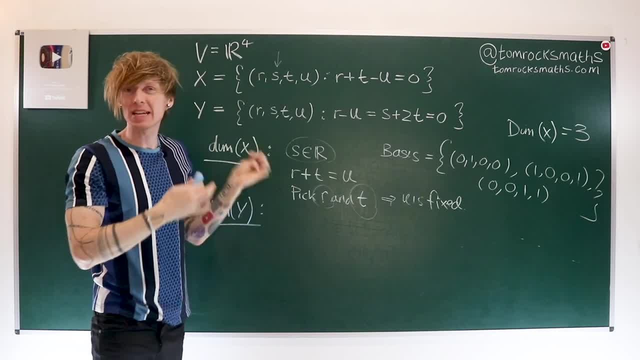 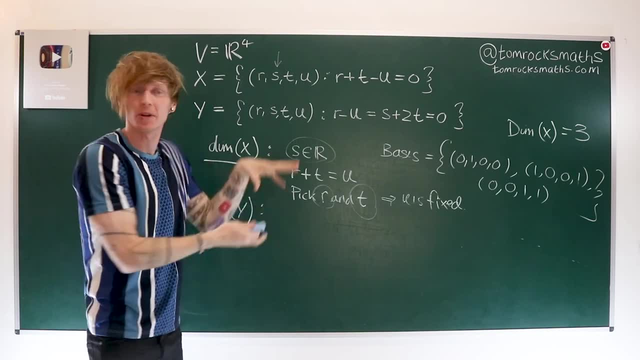 constraints and four free variables initially. So my intuition says I'm expecting this to have dimension two. Of course, this isn't a proof. We're going to go through the steps to show that hopefully, that is indeed the case and my intuition here is correct. So 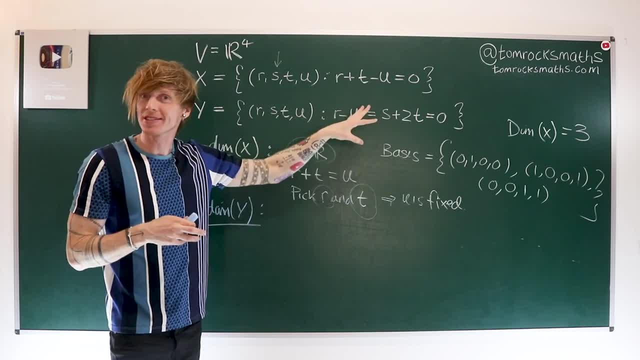 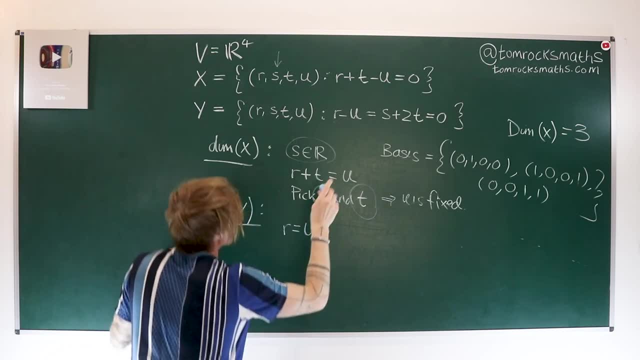 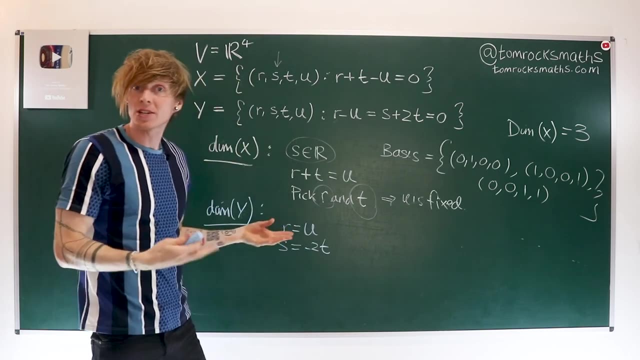 all four variables are now mentioned in our constraints and we have two of them. So we've got that r must equal u as the first thing, and the second one is that s has to be minus 2t. So each of these two conditions are basically telling us that I can pick r, so EG pick r. 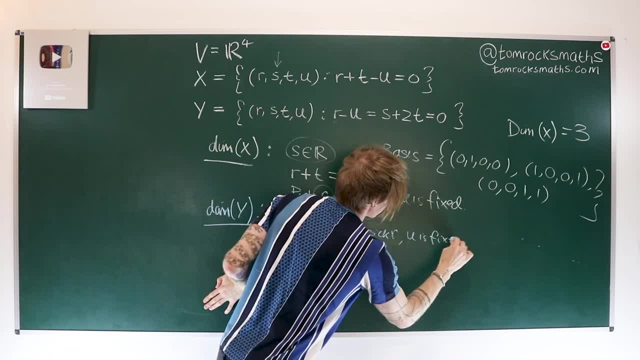 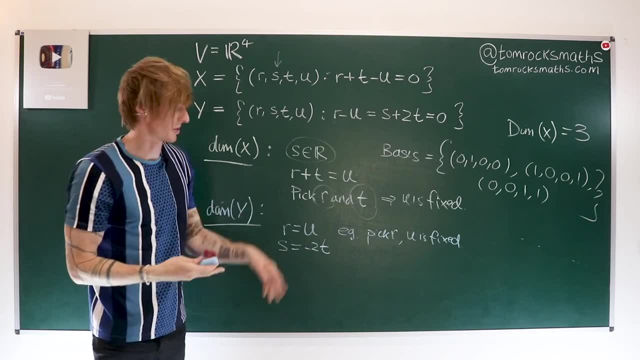 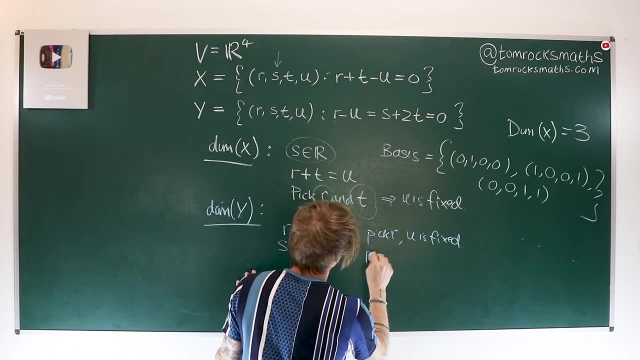 and then u is fixed. And similarly, we have a relationship between s and t, so I am free to pick one of them and the other one is fixed. So that's where I'm getting this idea that I expect the dimension to be 2.. So EG pick s, and then t is going to be fixed. 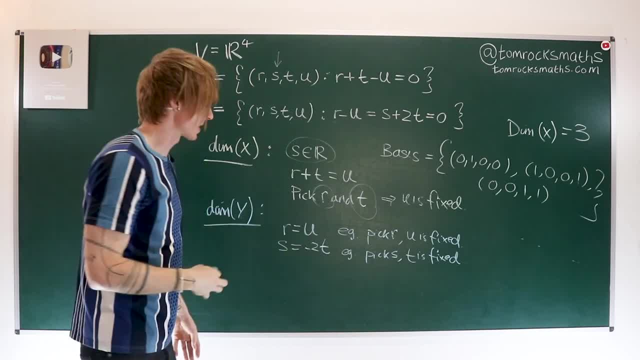 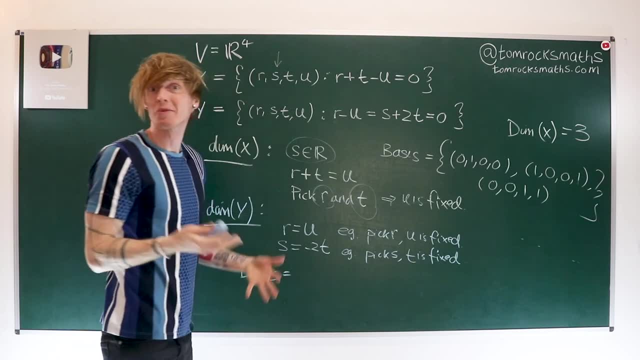 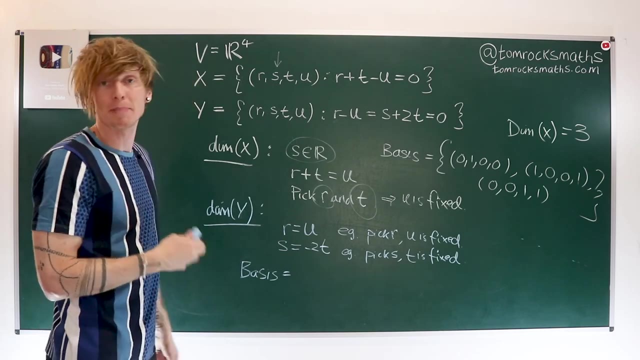 Okay, now again, we need to obviously construct the basis. so let's follow a similar idea to before, which basically means let's try and make things 0 and 1.. So if I pick, we need r and u to be the same. so if I pick them, let's say both to be 0, then that would be okay. 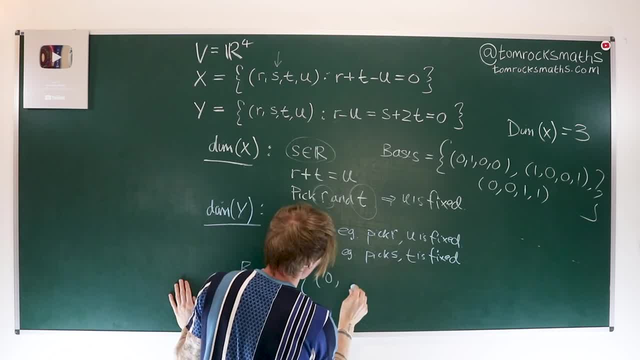 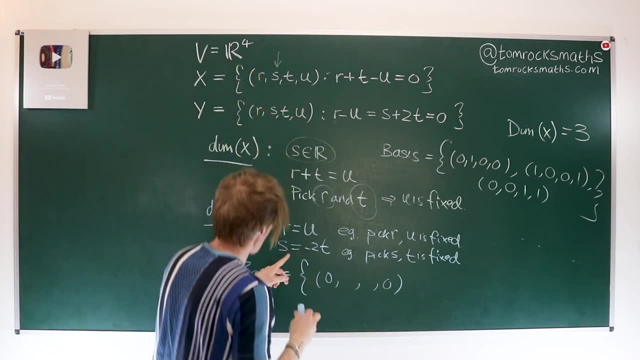 So if I make r and u 0,, so that would be a 0, something, something, and ending in a 0. And now if I pick s to be 1, for example, then what's that going to tell me? So if s is 1,, then 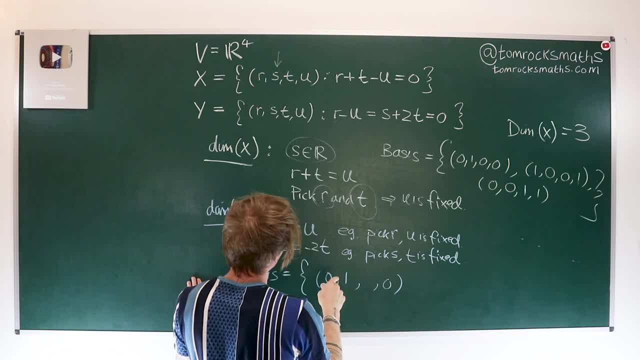 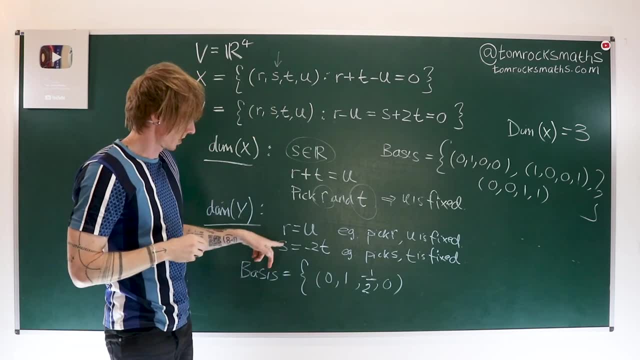 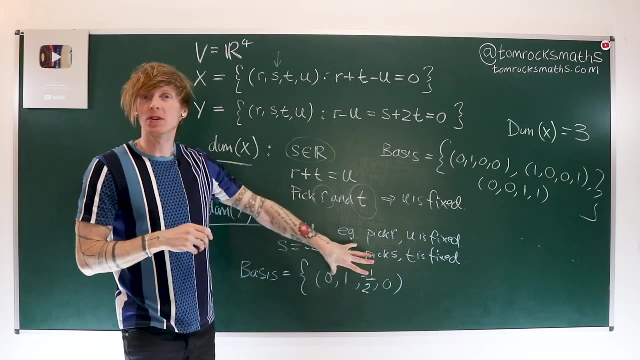 minus 2 times t has to be equal to 1, so t is minus a half. I think is going to work. so s is minus 2 times. that is correct. So that here sort of gives me a non-zero value and a relationship between s and t. So now let's flip it and let's instead put s and 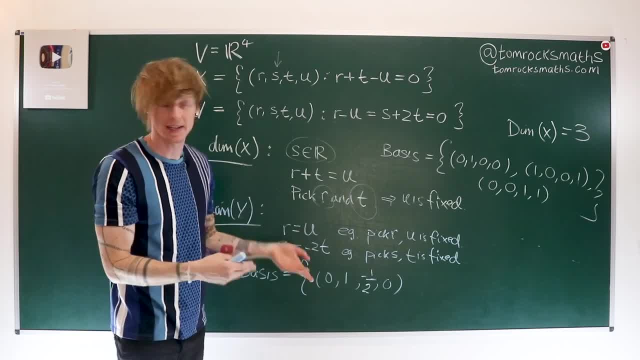 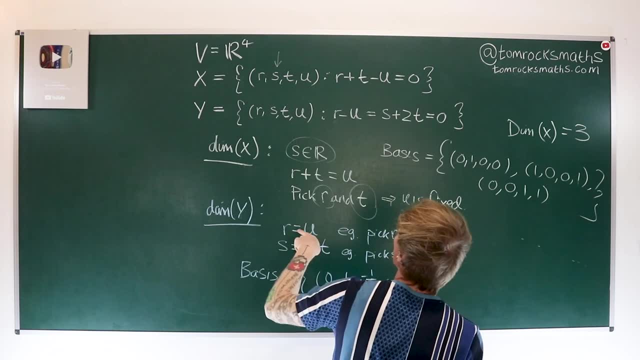 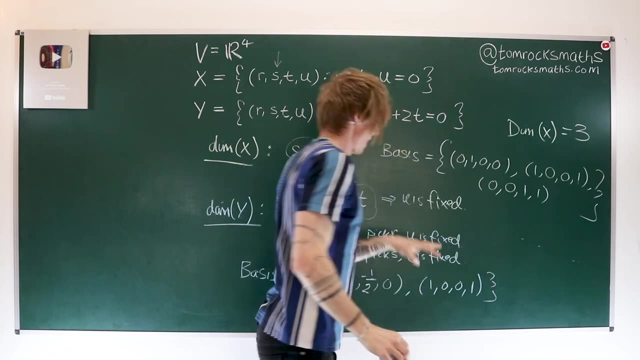 t to both be 0,, so this one is automatically satisfied. And then let's try and take this relationship between r and u. So the simplest thing we can do is make both of them 1, because again they have to be equal, so that'll be 1 0, 0, 1.. And again you should check that this is indeed a 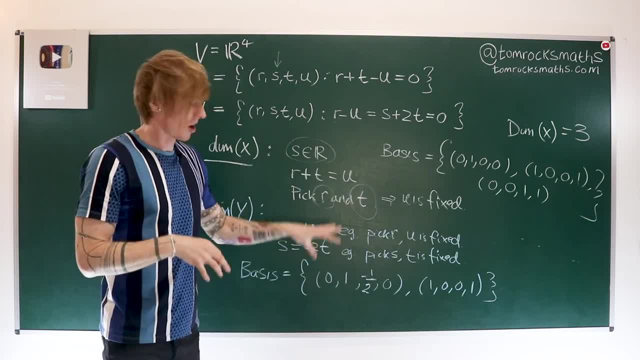 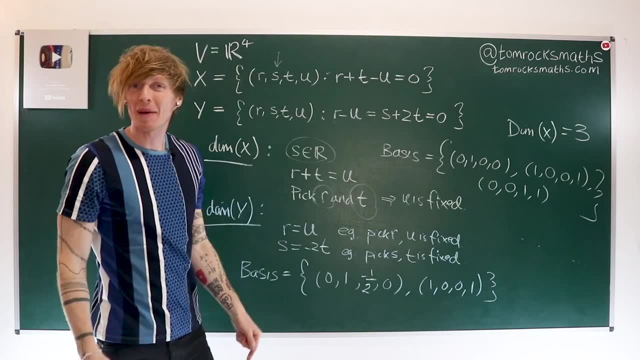 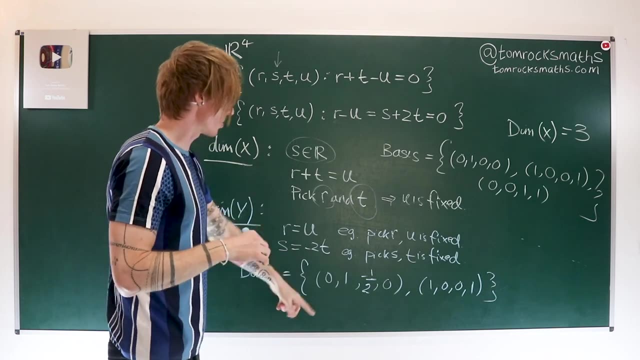 basis check. this is spanning check. these two vectors are indeed linearly independent, though you can hopefully see that, because we have zeros sort of alternating between the pairs of positions, which is why picking your variables to be 0 is very helpful. So again, we have 2 over here. 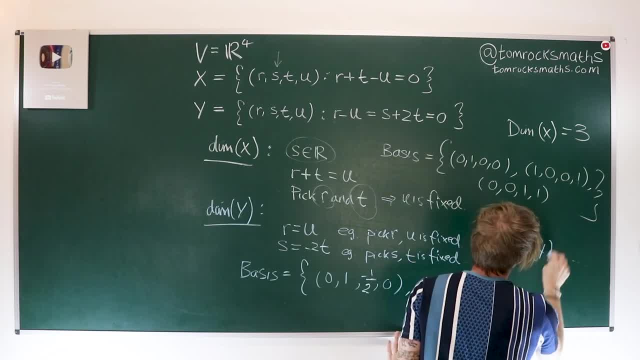 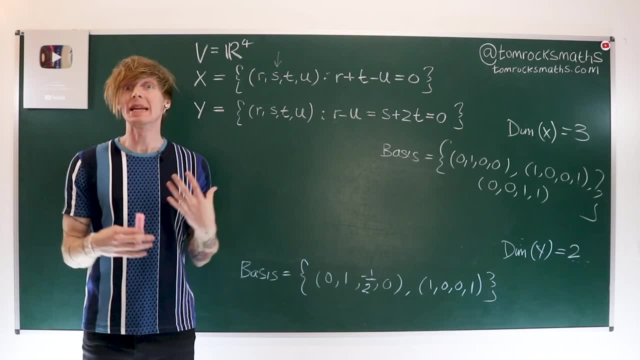 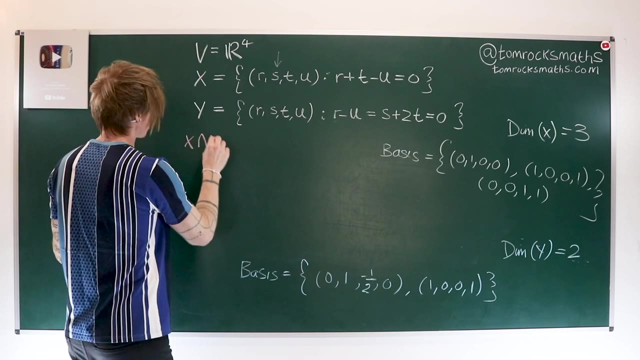 so I can say: the dimension is the number of vectors in my basis. so the dimension of y is equal to 2.. Let's now look at some combinations of our two subspaces, x and y, namely x intersect y. and let's also look at x. 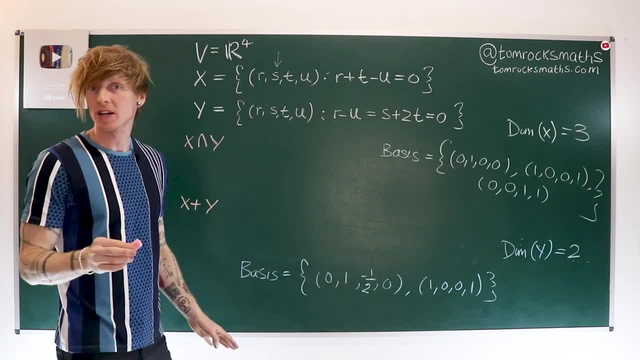 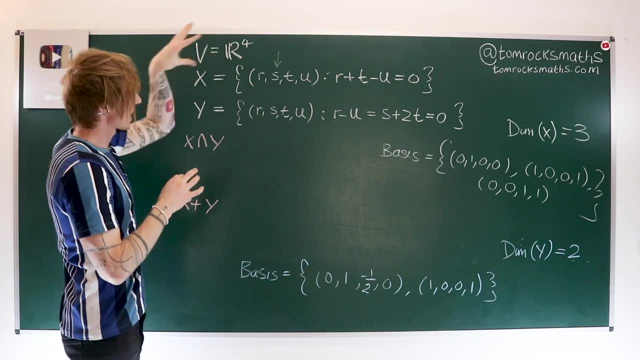 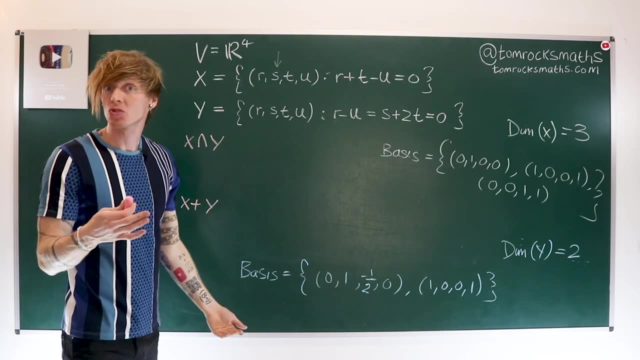 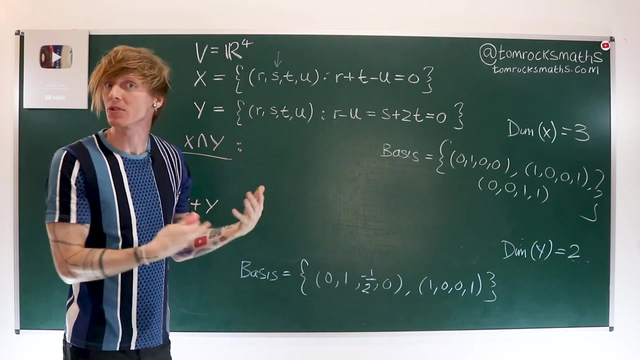 plus y. So first the intersection. If we have a vector that is in both the subspace x and the subspace y, then all three of these conditions must be true. So for something belonging to the intersection of the sets, it means it's in both sets simultaneously. So we need this to be true. 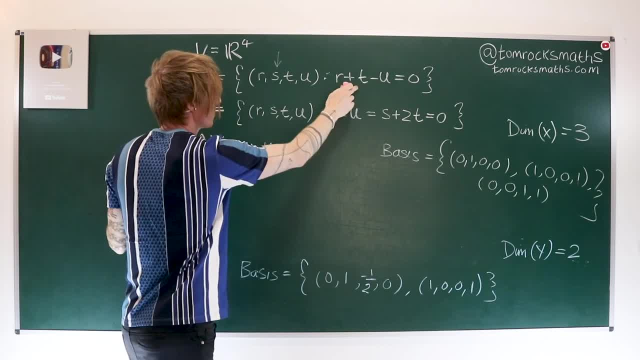 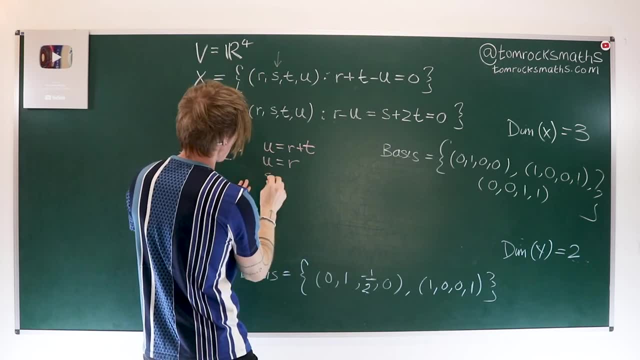 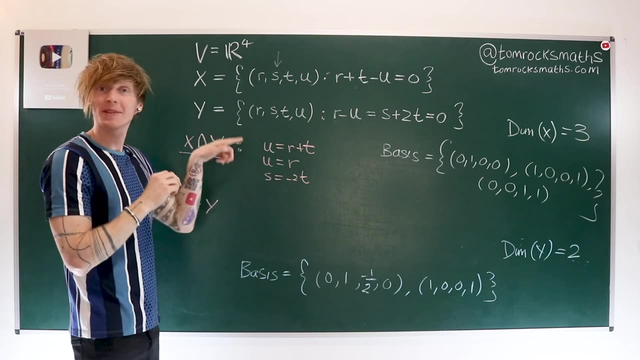 so that tells us that u is r plus t from here. We also know that u is r from here, and here we know that let's say s is minus 2t. So the first condition, u is r plus t, combined with the second condition that says u is r. 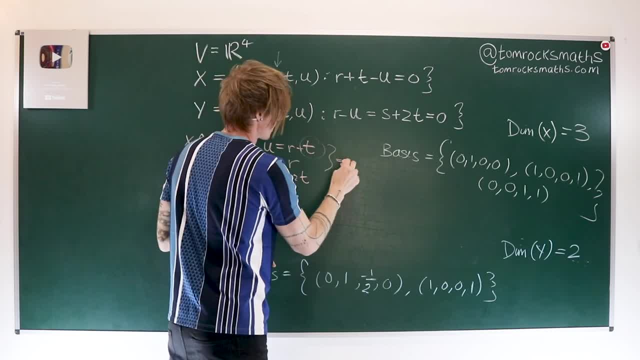 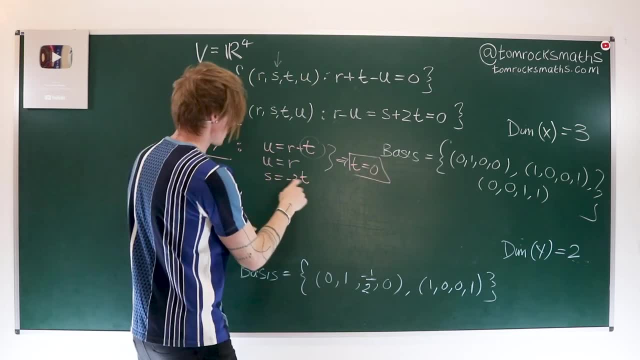 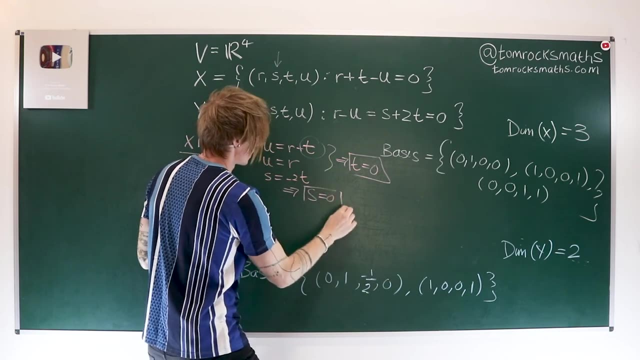 so we can cancel that, and that just leaves us that t has to be zero. So this tells us that t is 0,, first and foremost. And then we also have this condition that says s is equal to minus 2t. but if t is 0,, then this also tells us that s is 0. So we can see immediately. 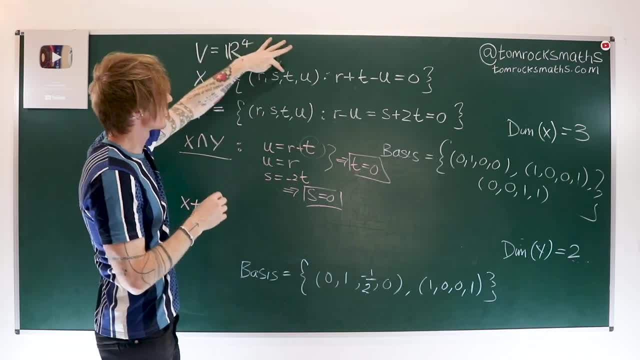 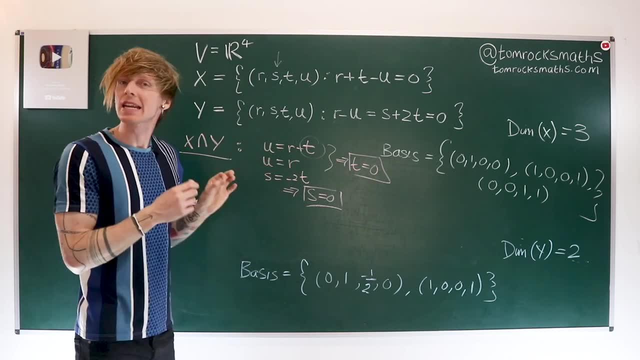 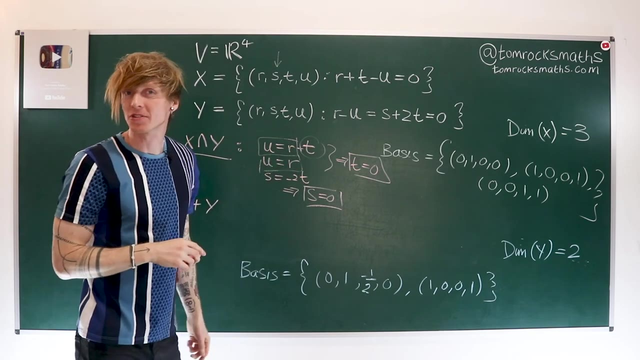 in order to be in both of these sets, you must have s on t, both equal to 0.. Now, in terms of u and r, there aren't actually any other conditions. We just need u to be equal to r, repeated twice, because t here is now of course 0. 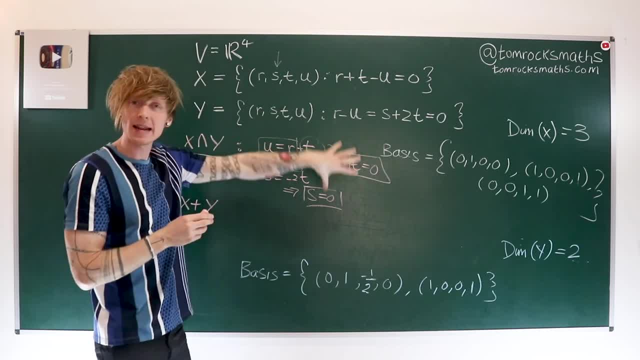 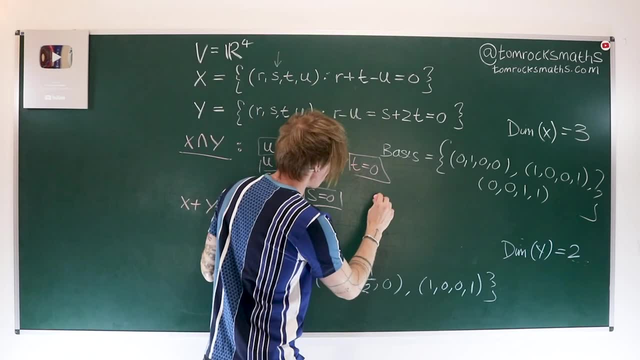 And that's it. So as long as u and r are the same and s and t are both 0, then we're going to be okay. So the only vector that's going to satisfy that would be something of the form 1, 0, 0, 1.. 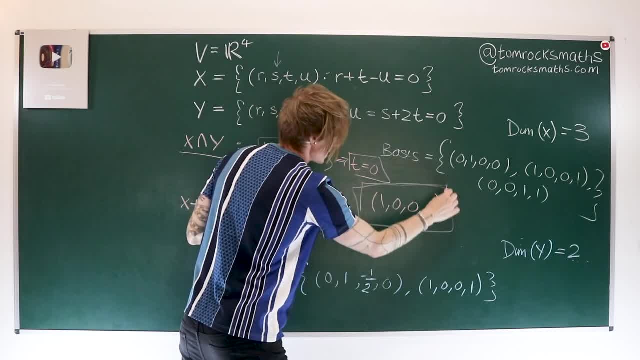 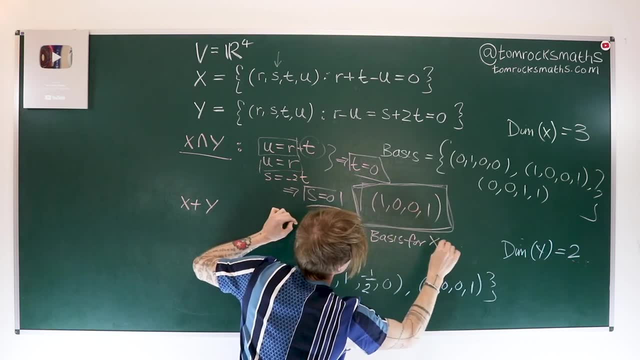 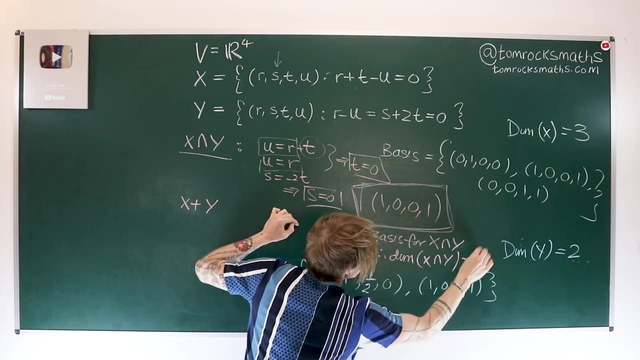 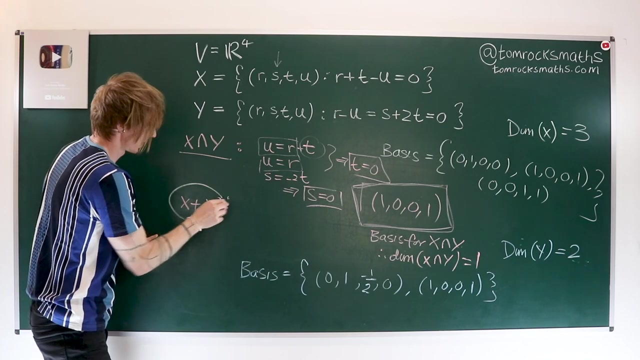 So this is going to be the basis for our intersection. So this is the basis for x intersect y, and therefore the dimension of x intersect y is going to be equal to 1.. Now for x plus y. over here we don't actually need to do any further calculation. 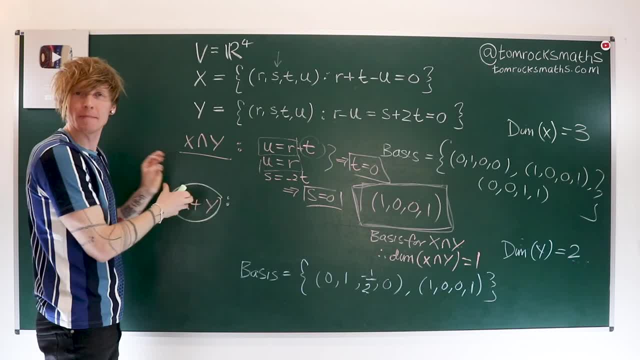 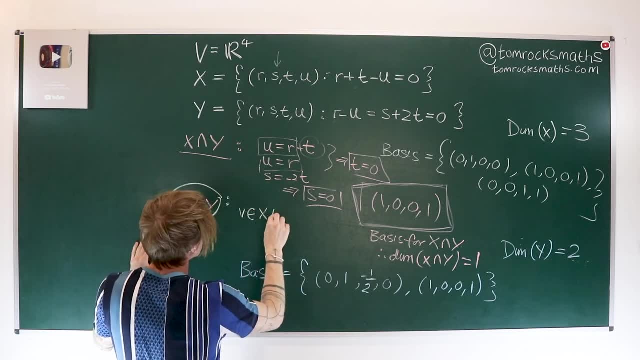 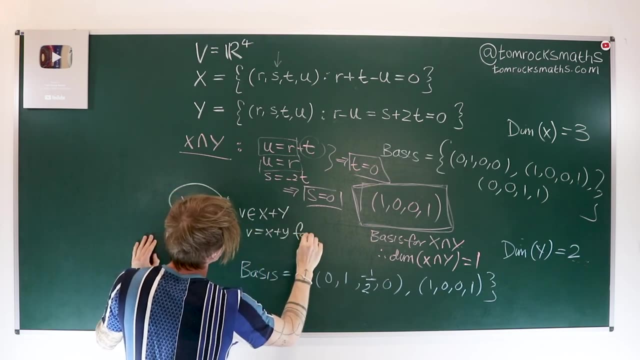 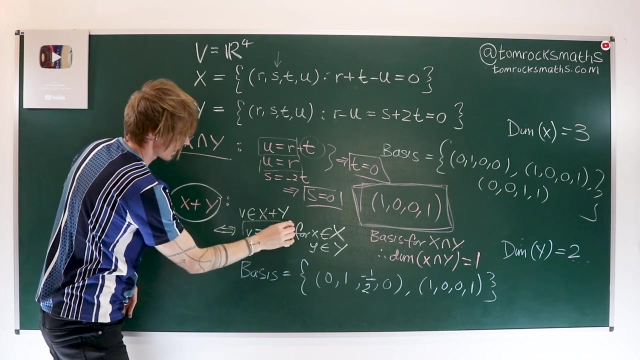 Because if a vector belongs to the sum of two vector spaces, then what this means is, let's say, v belongs to x plus y, then that's telling us that v must equal x plus y for sum x in x and y in y. So you have a vector which is made by adding together two pieces. One piece comes from: 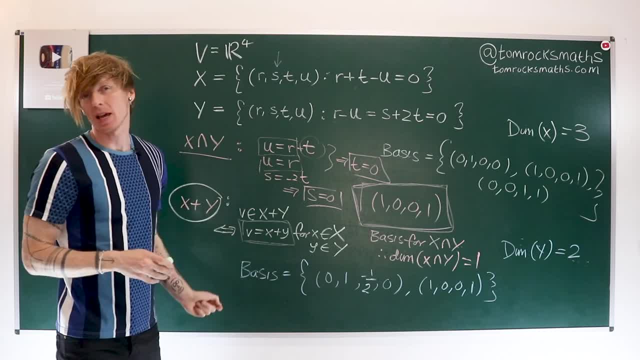 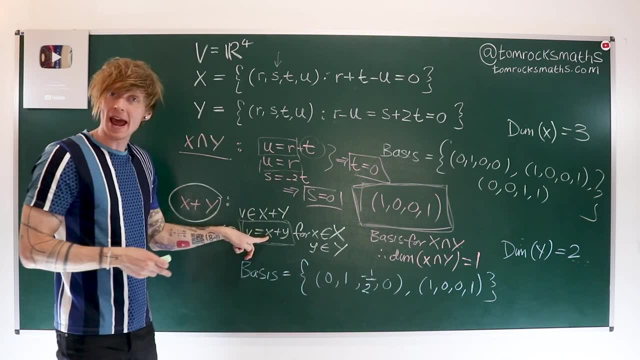 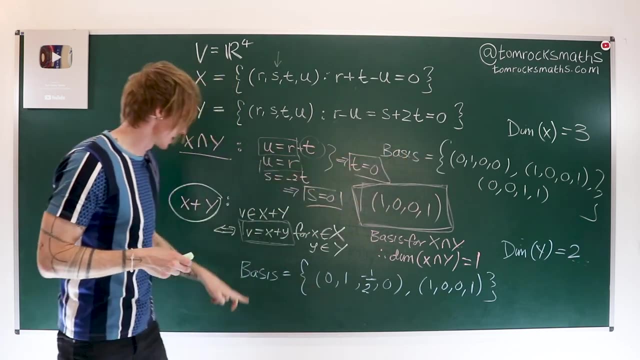 the first subspace, x, and the other piece comes from the second subspace, y. So anything in here has this form. Now we know that anything in x has to come from a linear combination of the basis vectors of x and anything in y has to come from a linear combination. 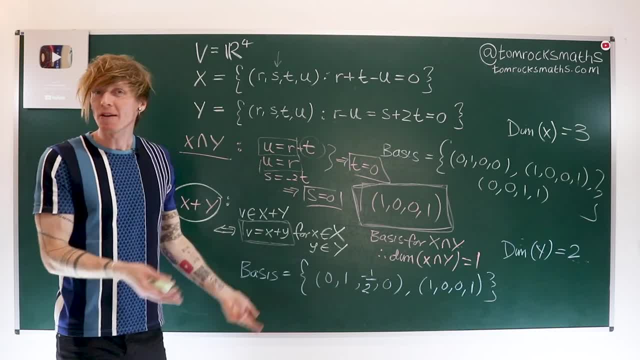 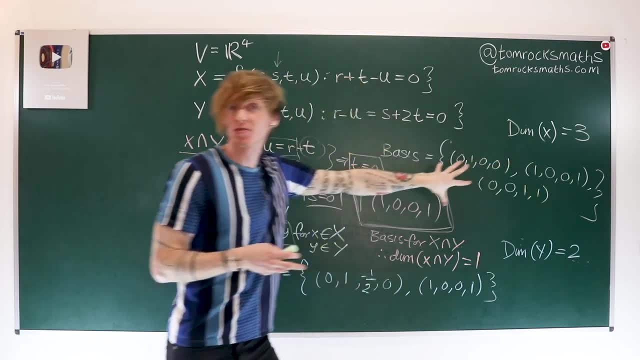 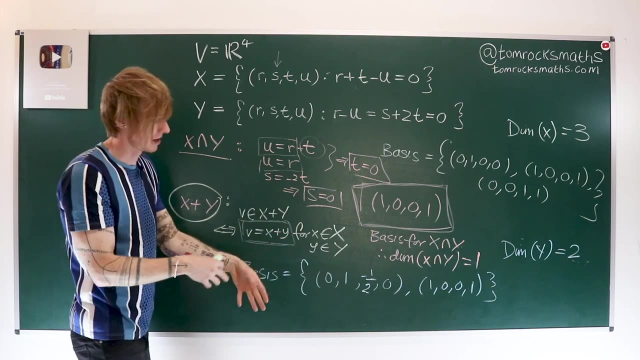 of the basis vectors in y. So, therefore, because we are able to add any amount of the x basis vectors, so any amount of these three, any linear combination, and that would give us something in x, And then we add on any amount of these basis vectors the basis vectors of y. 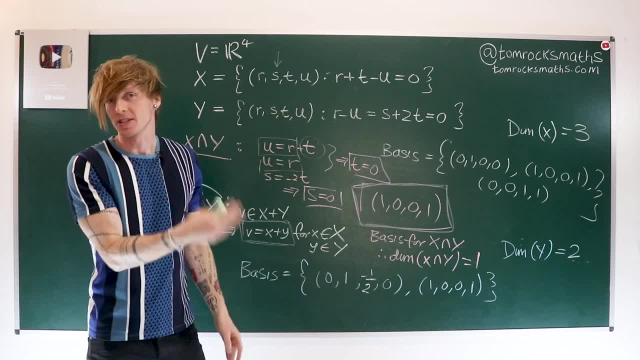 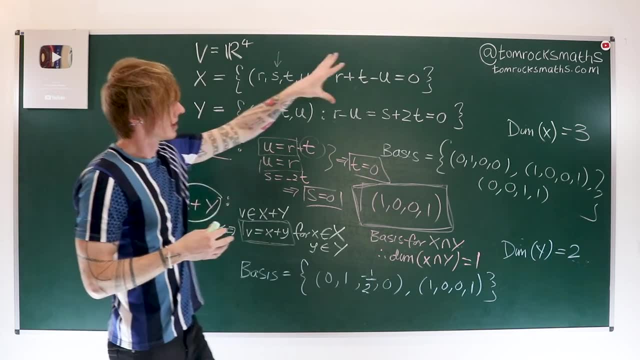 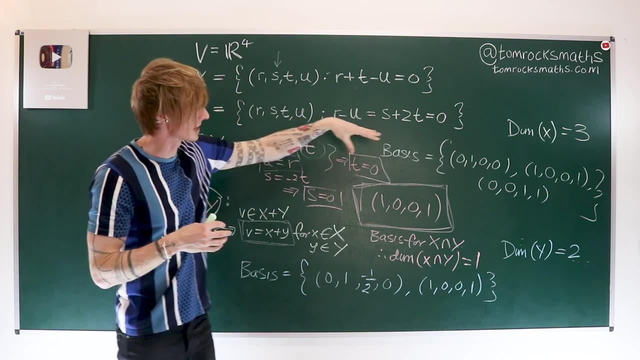 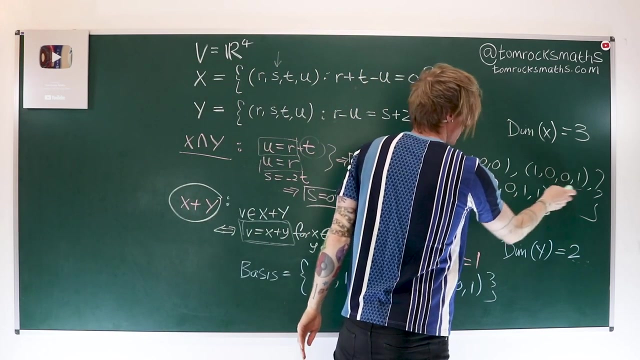 because that gives us the most general element in the subspace y. Any v over here is actually just a linear combination of these three plus these two, And if we look at these two bases we can see there's actually a repeat element. We have this: one, zero, zero, one element. 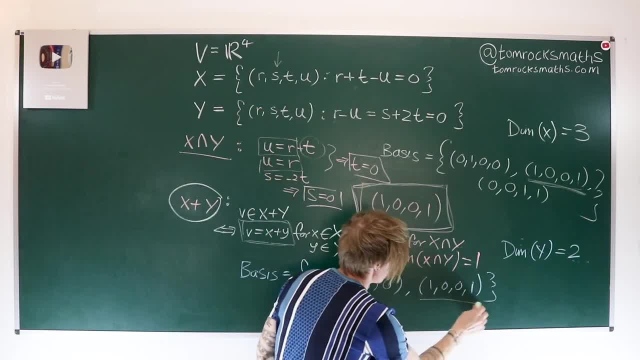 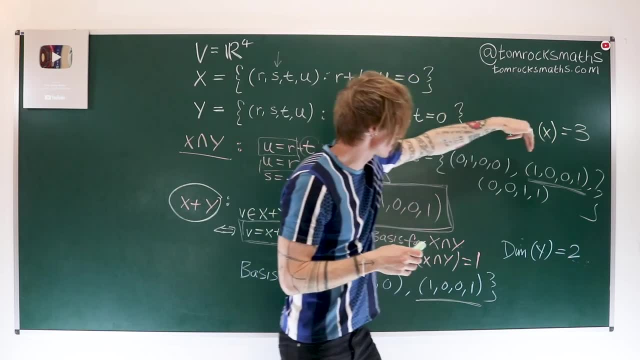 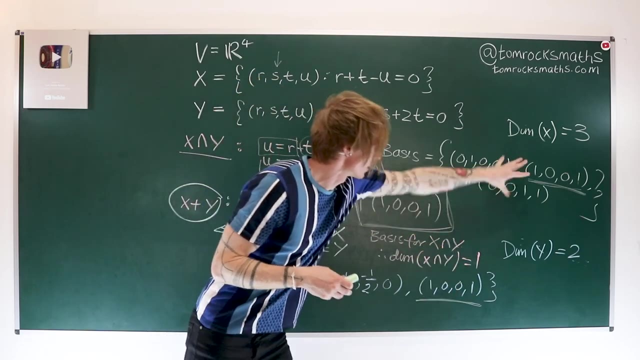 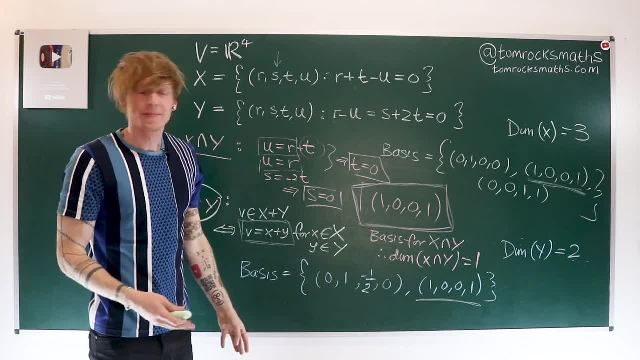 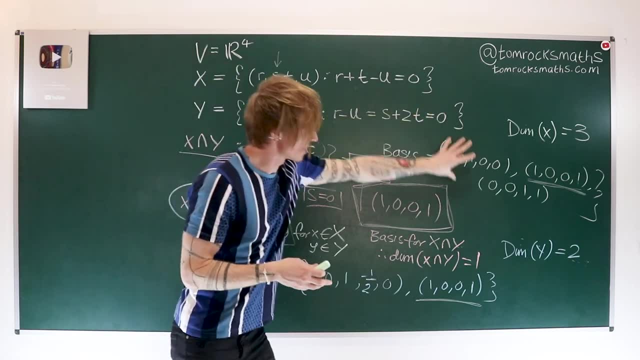 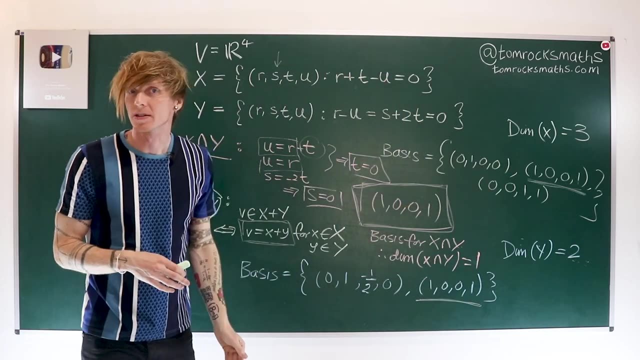 So we only need to actually represent it once. So the dimension of x plus y is going to be the sum of the dimensions of the two bases, but without this repeated element, because, again, it is redundant. So what we're going to see here is that the basis. 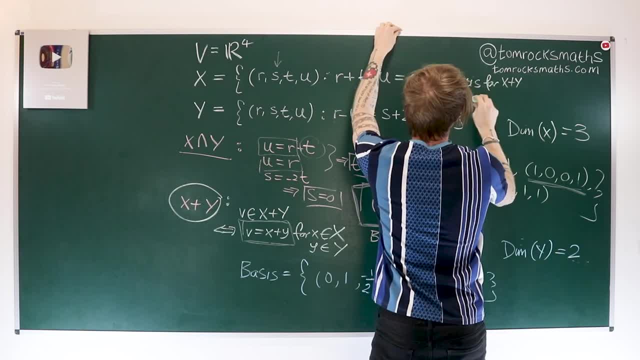 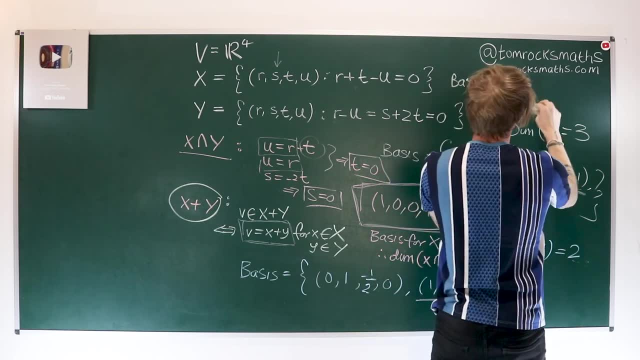 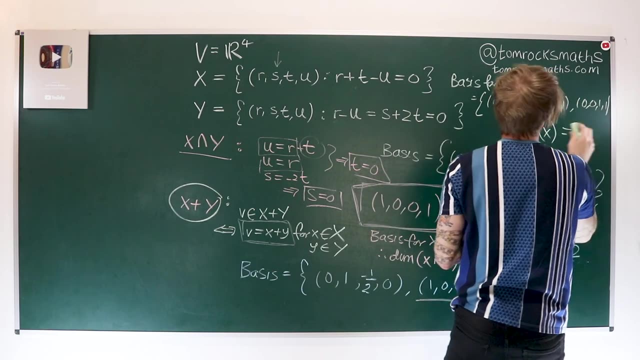 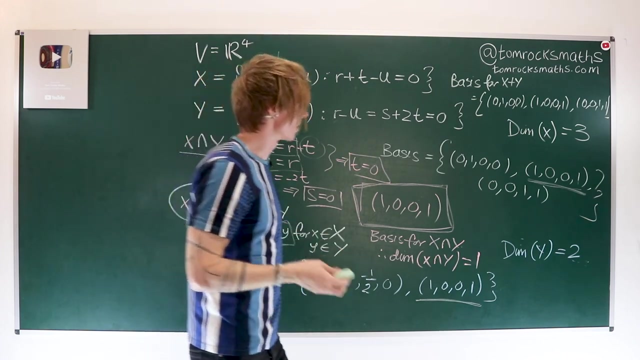 for x plus y is actually going to be the sum of the dimensions of the two bases. So that's going to be, let's say, all of the basis of x: zero, zero one and zero, zero one one. And then we take the other remaining different element from the basis for y. So zero one minus a half. 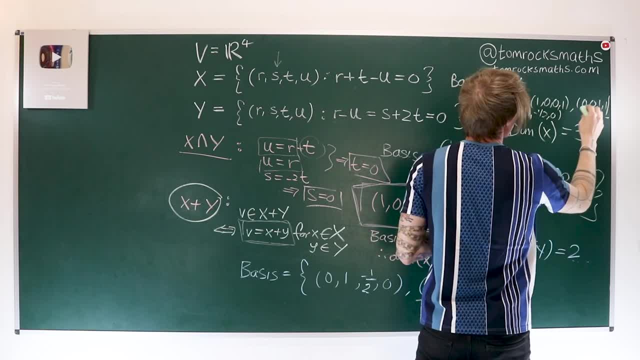 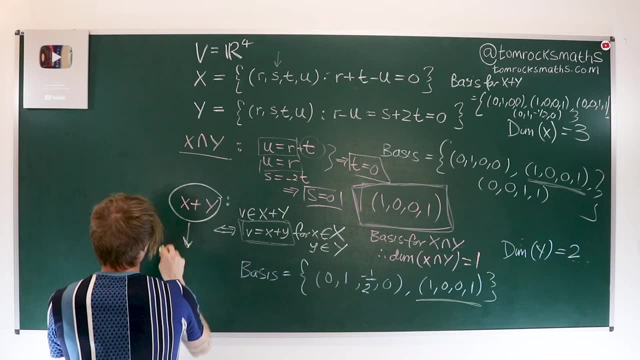 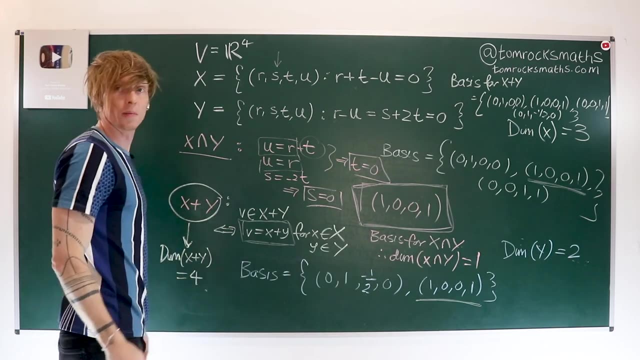 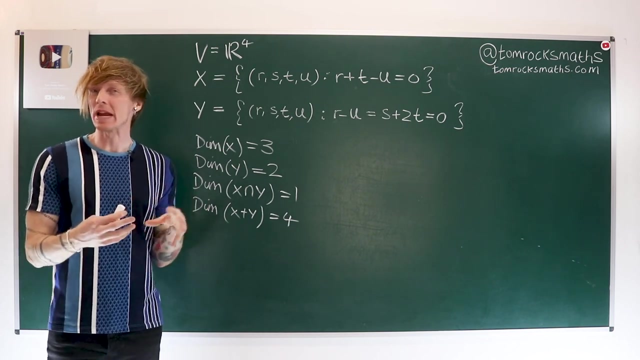 zero. So that's going to be our basis, and so, therefore, the dimension for x plus y- Let's write it down here- the dimension of x plus y is going to be equal to four. Now, in that last calculation there was actually quite a big clue as to what was going on with the dimension formula, the subject or the topic. 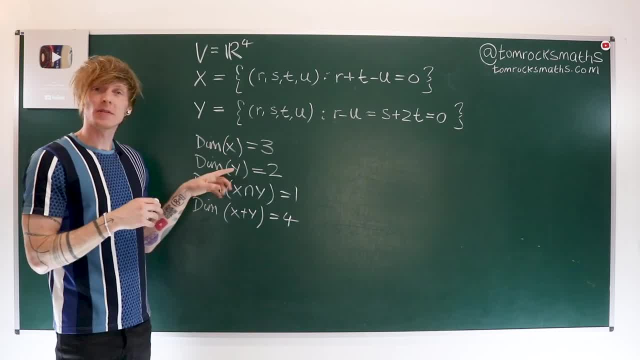 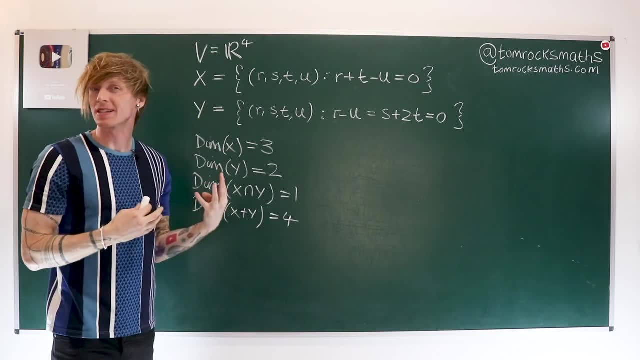 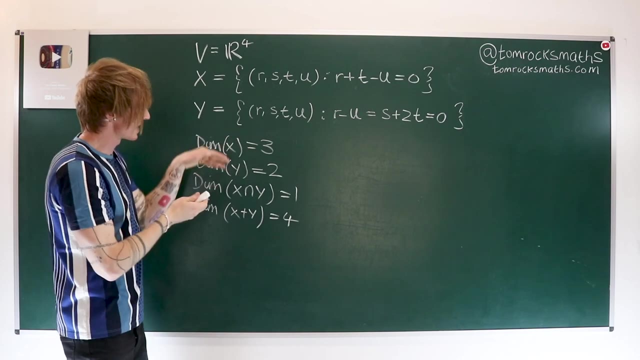 of this video. So we saw that in order to get the basis for x plus y, the sum of the of our two vector spaces, In order to get that basis, we just sort of took the union or added together the bases for x and y, but we removed the bit that was repeated because it was redundant to 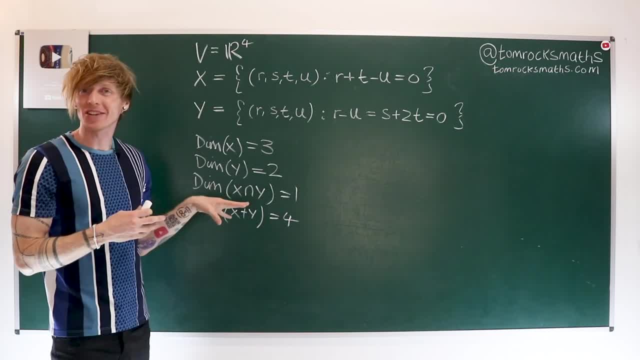 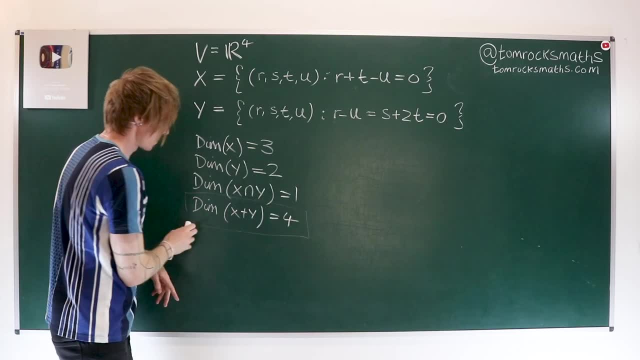 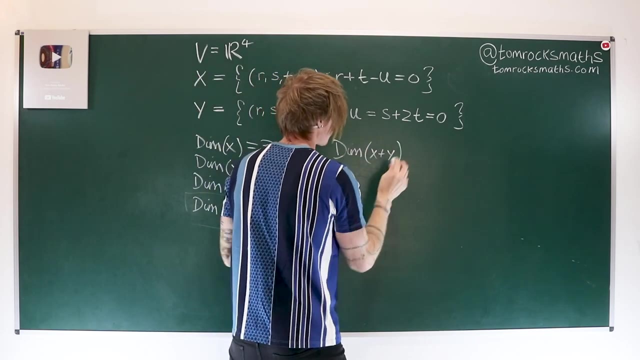 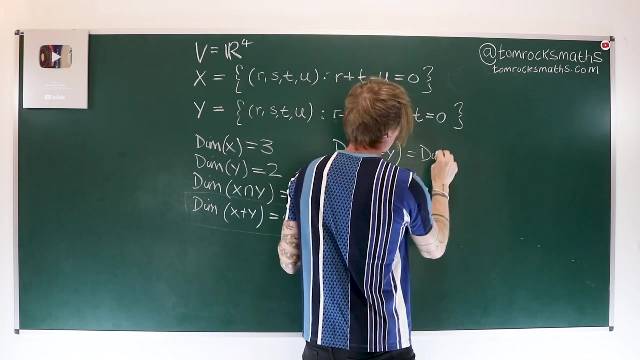 include it twice. And if you look at the dimensions, that's basically what's happened, because if we take the dimension of x plus y, which here is 4, so if we say dim of x plus y, which again is 4, and then we can say: well, that's equal to the dimension of x, which is 3, plus the dimension of y. 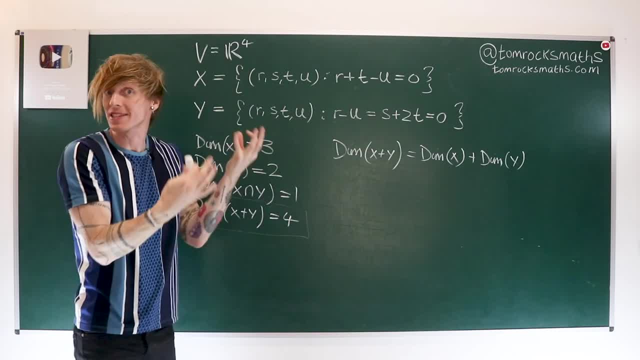 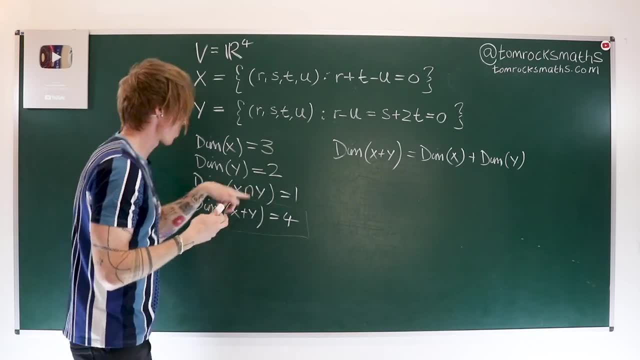 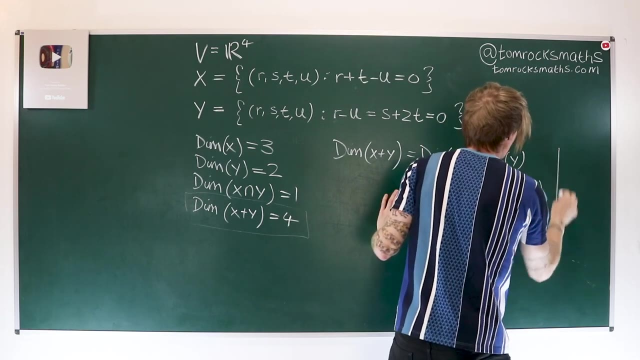 so sort of adding together those two bits and adding together their basis vectors. but we have to remember to subtract off the bit that's been repeated, the bit that's in both of them. so we subtract the dimension of x, intersect y, and this result is in fact the dimension formula which, in just a moment, 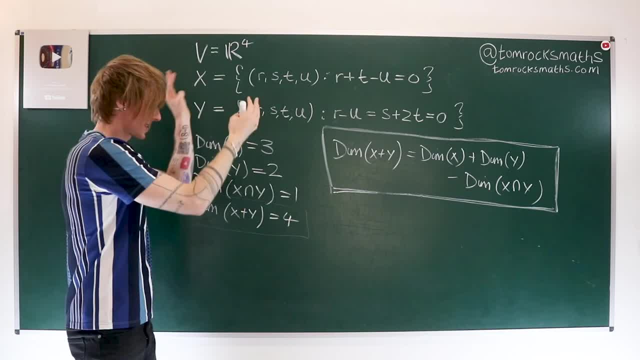 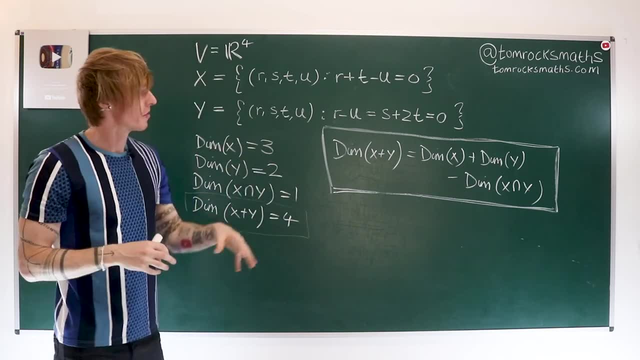 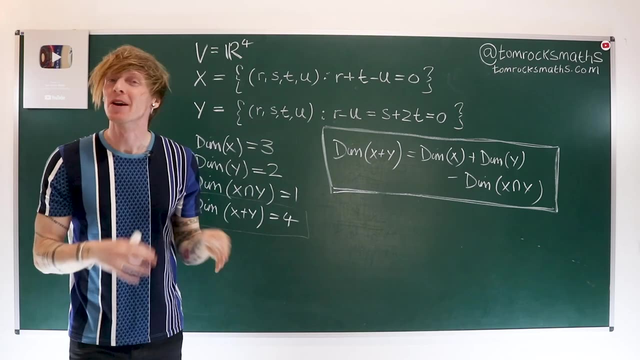 we are going to prove. This, of course, is a single example where it happens to be true, but I was hoping to use it as motivation for where this formula comes from. But of course, being mathematicians, we can't just rely on examples where it works. 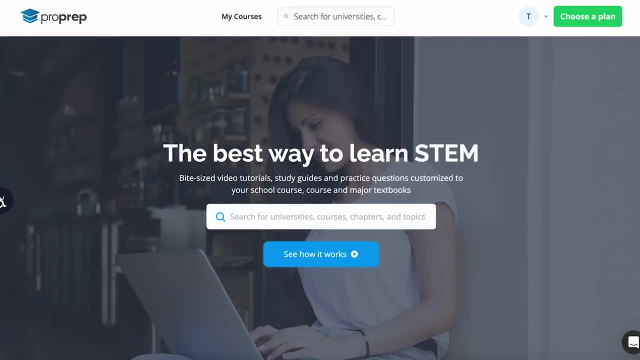 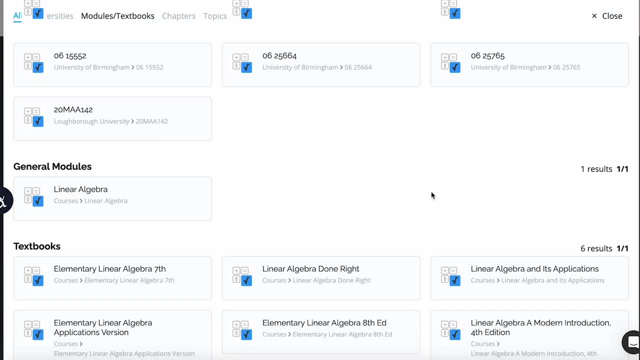 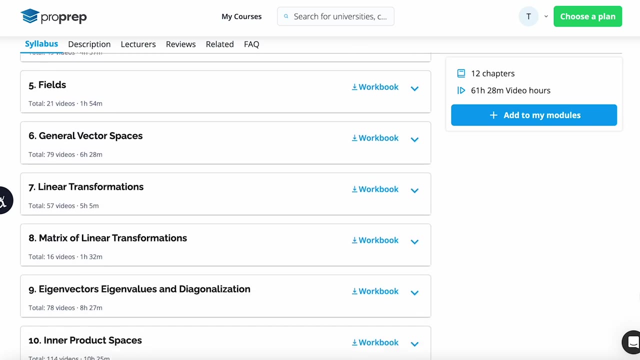 We need to actually do a formal proof, But before we do that, let me first point you in the direction of ProPrep, an online resource which provides customized tutorials for students looking to improve their skills in stem-based subjects. The linear algebra section is a great accompaniment. 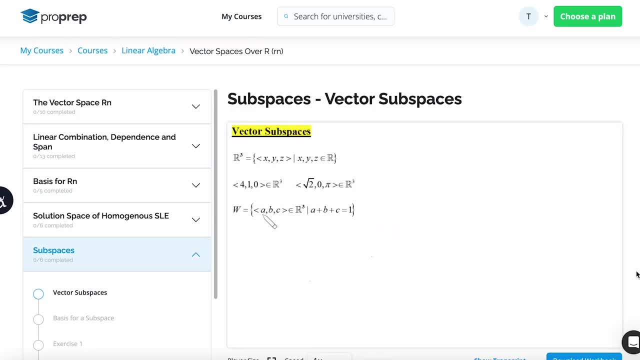 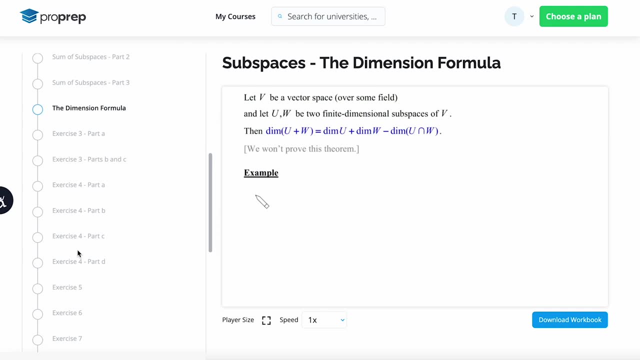 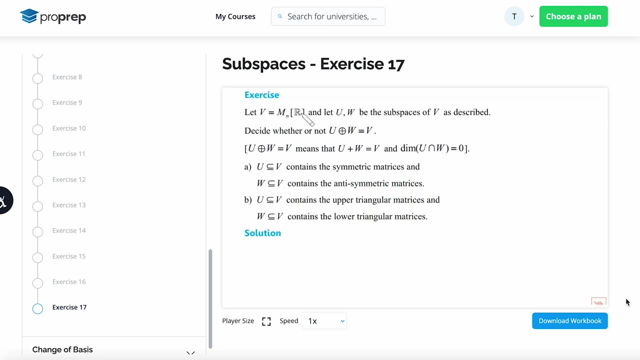 to the Oxford linear algebra video series, with short lecture videos going over the key topics, Alongside several worked examples. for each section, the dimension formula has its own video, along with 17 exercises for you to have a go at, each with their own video solution. and if you just 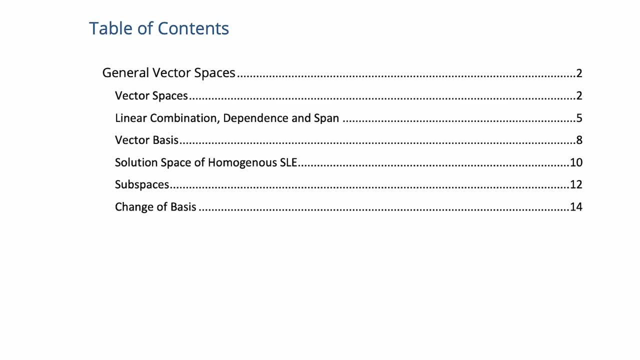 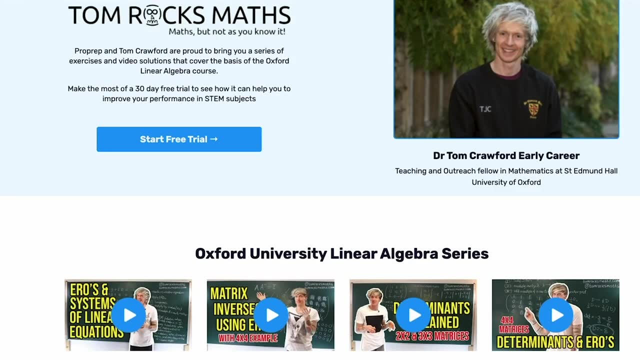 want to check your answers, you can always head straight to the exercise workbook, which contains each question and solution for the entire linear algebra course. Sign up for a 30-day free trial by clicking on the link in the video description and discover how ProPrep can help you to. 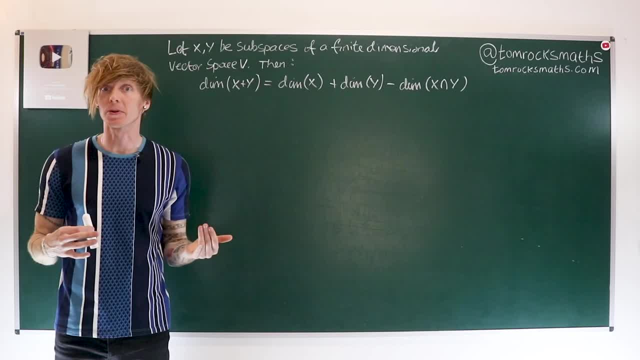 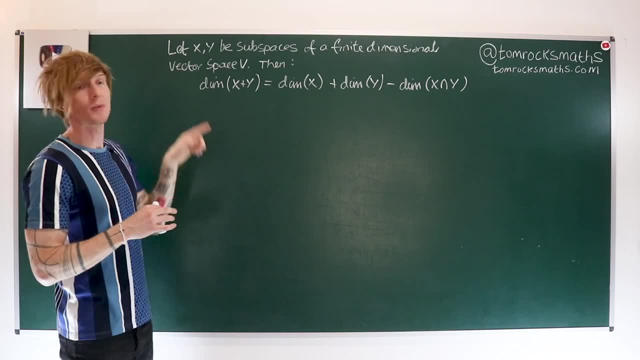 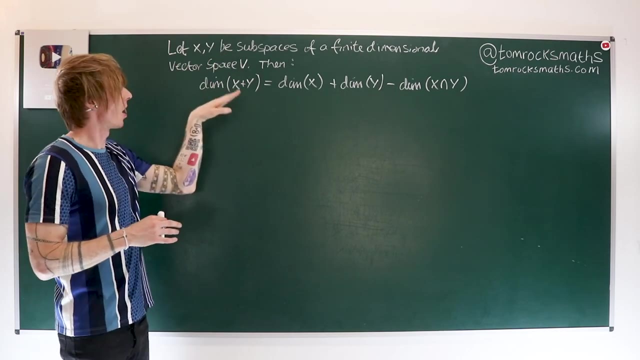 improve your stem skills. Okay, time for the proof. The formal statement of the dimension formula is written here on the board. so we have x and y are subspaces of a finite dimensional vector, space v, and we want to show that the dimension of x plus. 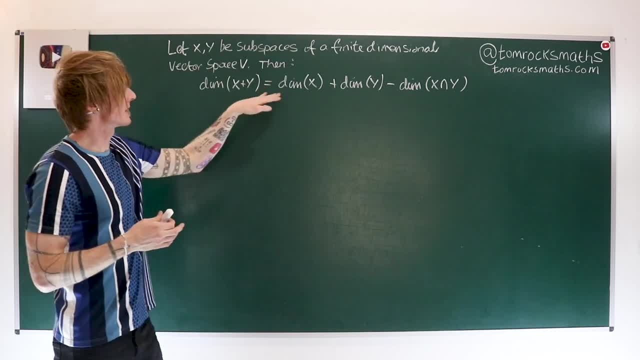 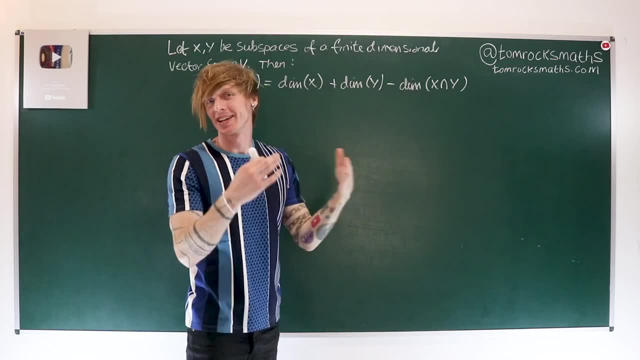 y as a subspace itself is equal to the dimension of x plus the dimension of y, minus the overlap, minus the dimension of x into the vector space, and the dimension of x plus y plus the dimension of y minus the dimension of x into the vector space. 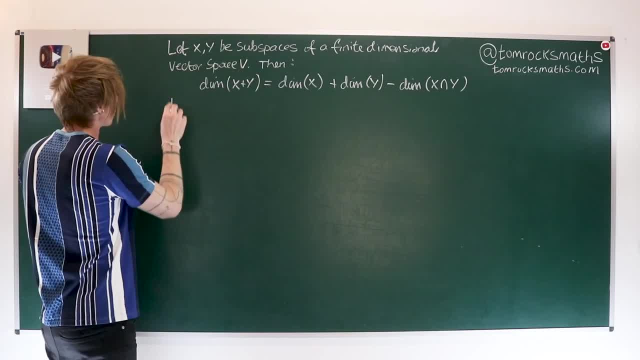 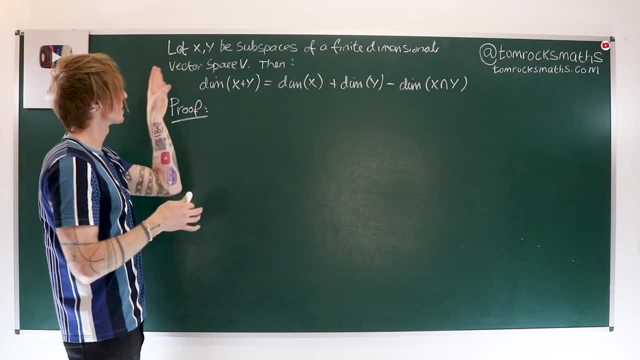 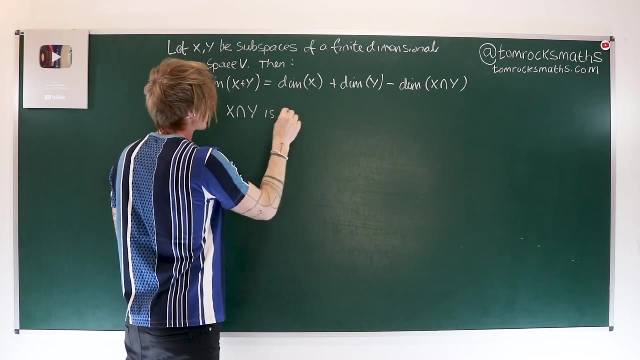 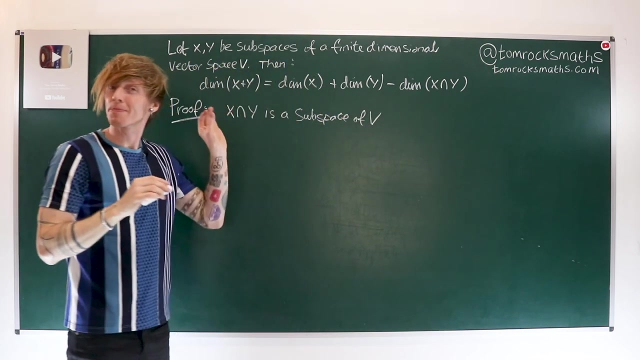 โ� โ� y. So proof Now. our starting point relates to the fact that both x and y are subspaces and therefore x intersect. y is a subspace of V. Now we did prove this in an earlier video in the Oxford Linear Algebra series. It was the video on: 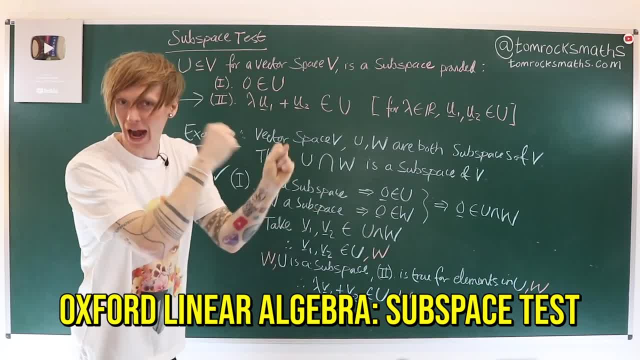 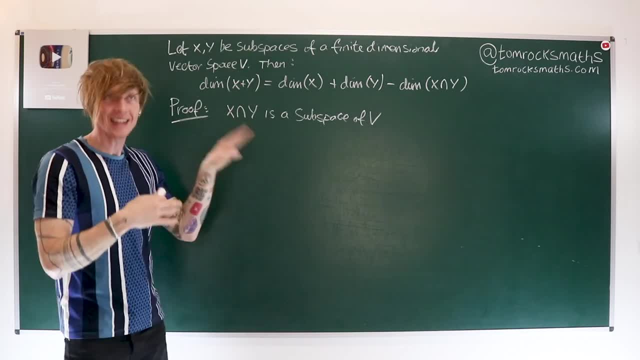 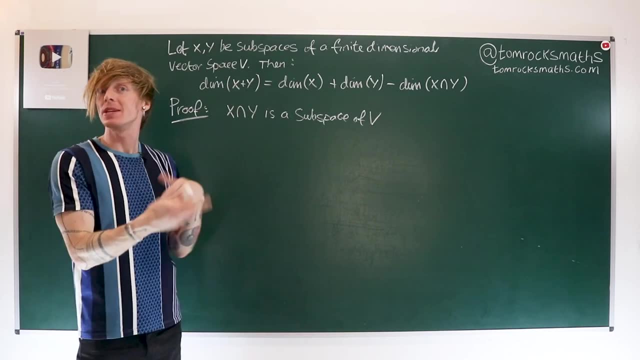 subspaces and the subspace test, and we simply applied the subspace test to the intersection of two previous subspaces to show that the intersection is also a subspace. So I won't do that here. we will simply assume this fact. but if you need, 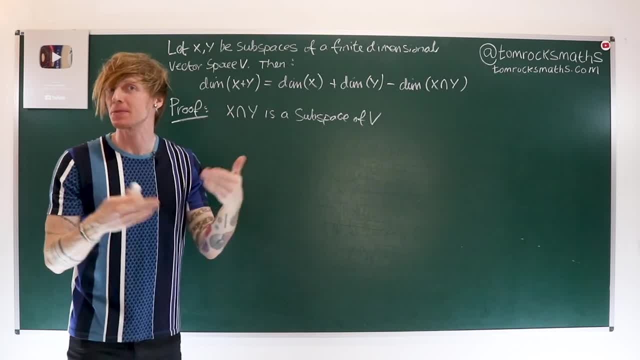 a reminder, you can go back now and watch the video on the subspace test. So, given that x intersect y is a subspace of V, we simply applied the subspace test to the intersection of two previous subspaces to show that x intersect y is a subspace of V. 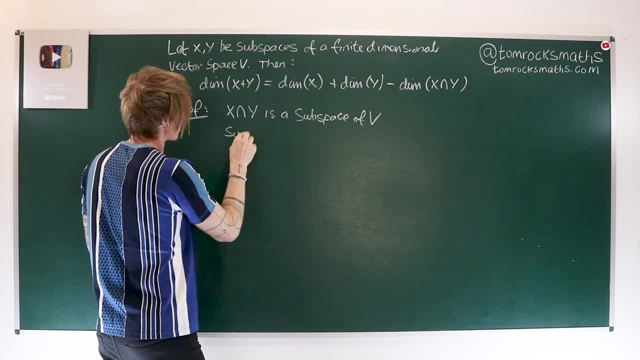 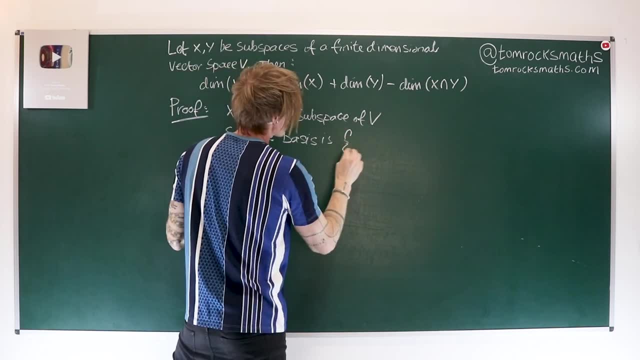 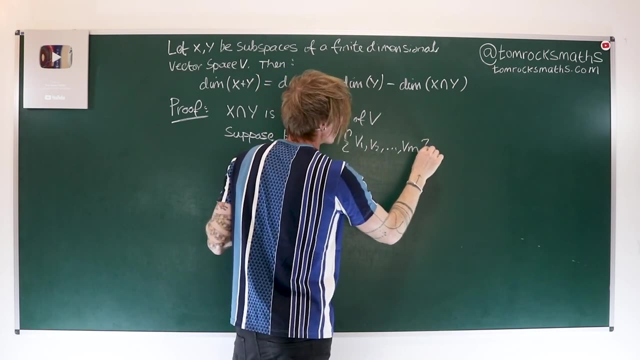 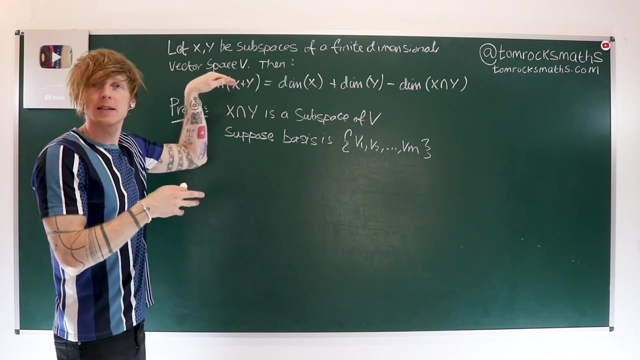 That means it has a basis. So suppose the basis is given by a series of vectors. Let's call them v1, v2, up to vm. So it has some size. its dimension here is clearly m, And since x intersect, y is contained in x. 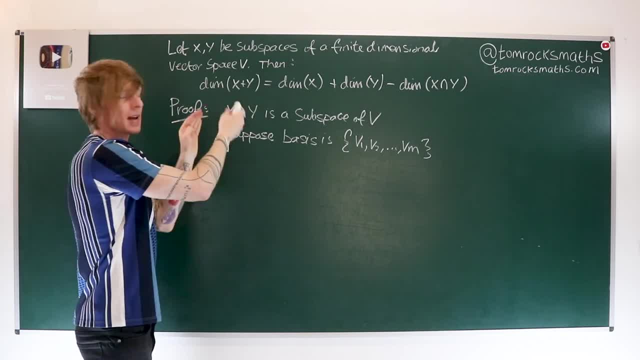 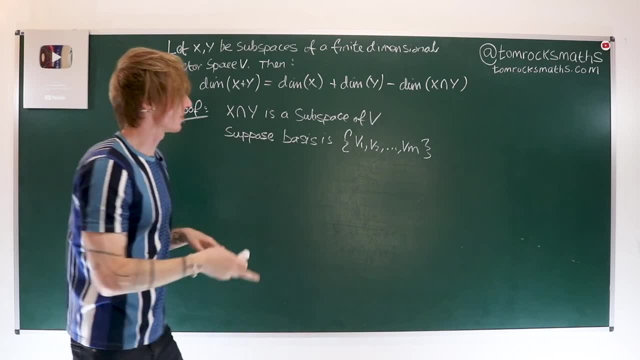 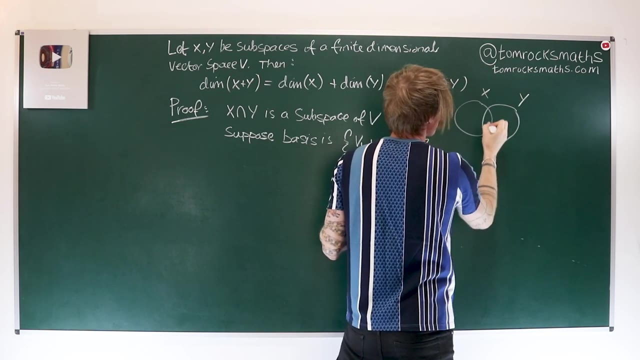 and since x intersect, y is contained in x, because this is all vectors that are in both x and y. So clearly, everything in this subspace is also in x itself And, if you prefer, you can think of it using a Venn diagram. So if this is x and this is y, then this bit in the middle is going: 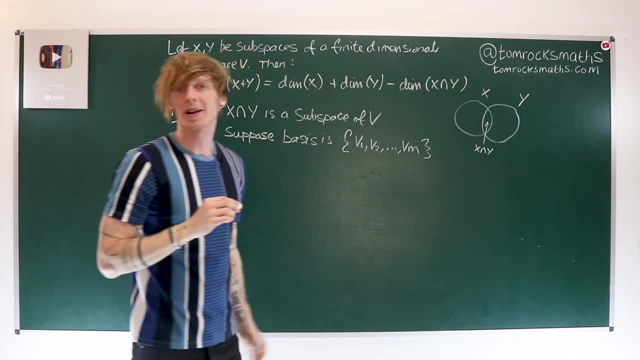 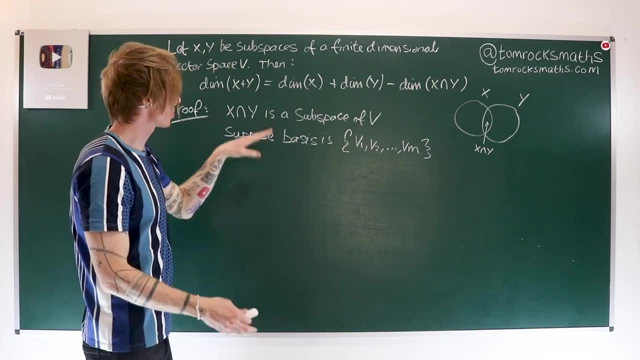 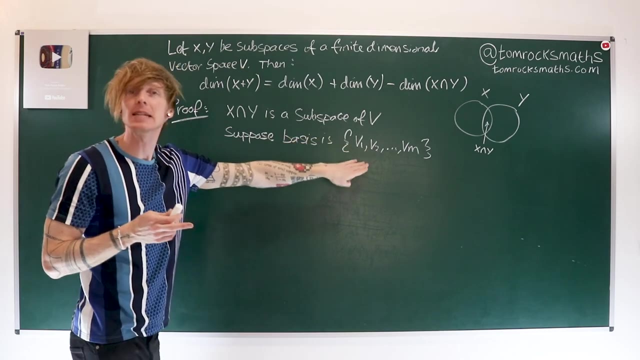 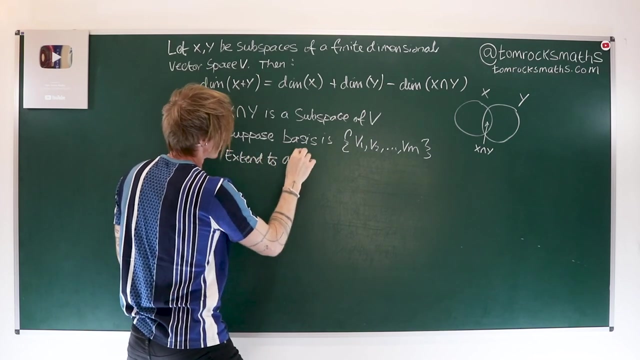 to be: x intersect y, And in fact, this picture is very helpful for understanding where the dimension formula has come from. So, So everything in the intersection is also in x. So what that means is: we can extend this basis. So we can extend to a basis of x. 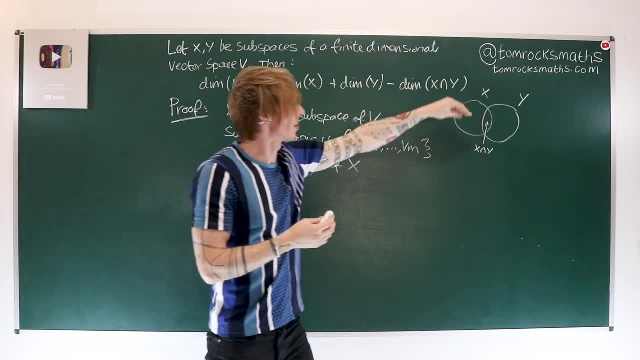 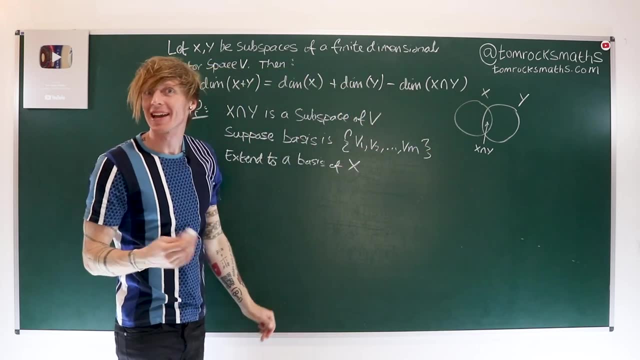 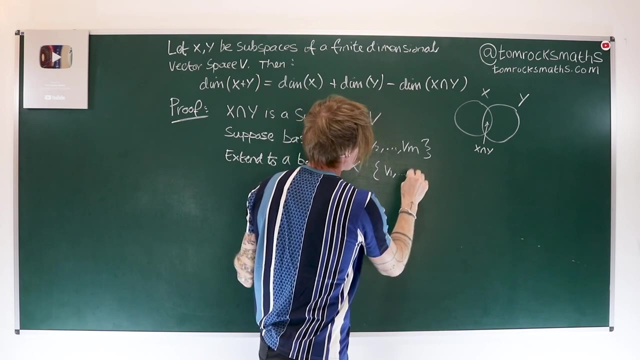 So we have a basis for everything in the middle and then we just say, well, we can just keep adding new vectors until suddenly we have enough to cover all of x. So if we extend this to a basis of x, then we can suppose that is now v1 up to vm. 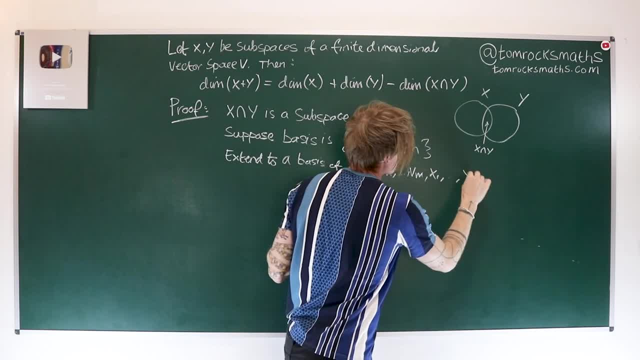 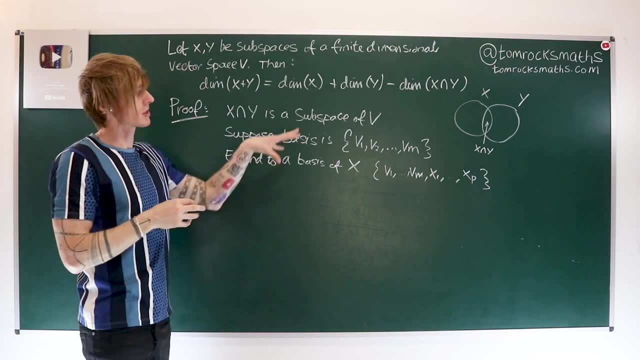 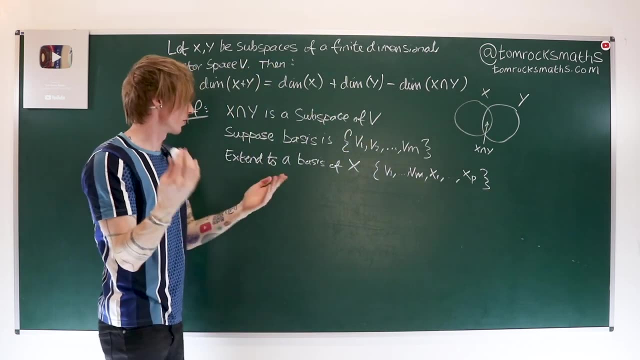 And now let's suppose we've got x1 up to xp, So this now has a dimension of m plus p. But just like x intersect, y is in x, it ocse is also in y, So we can also extend. So we can also extend to a basis of y. 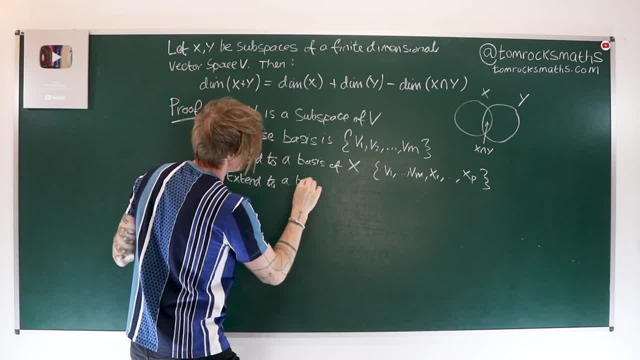 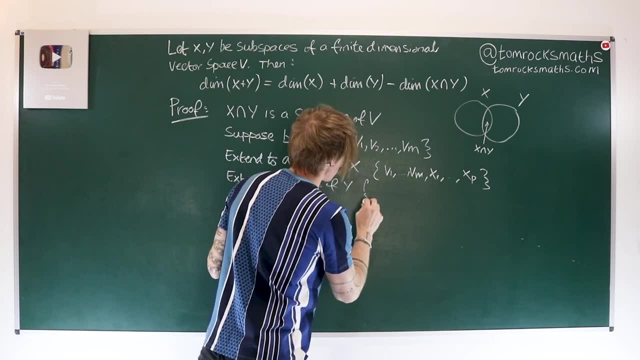 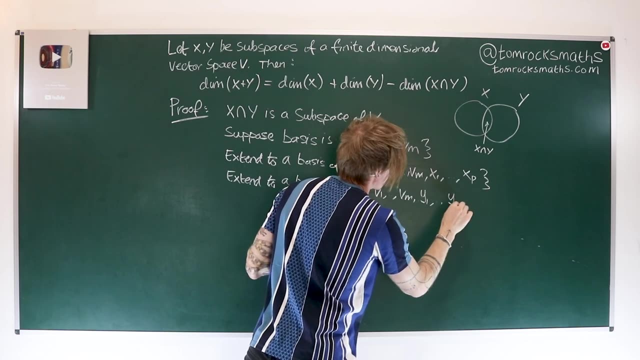 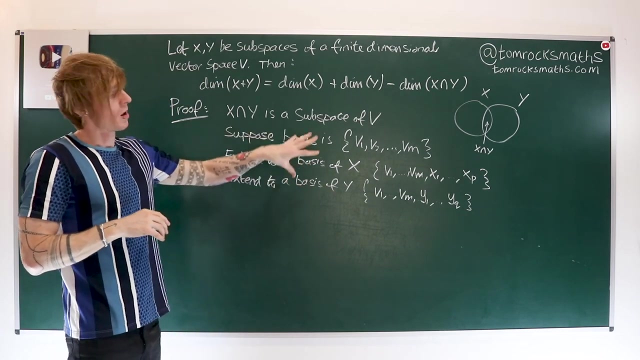 So extend to to a basis of y, and now we will be adding different vectors. So we still have v1 up to vm, but now let's add y1 up to yq, So this has dimension m plus q. Now, what I'm going to claim, and then, of course, we will have to prove- 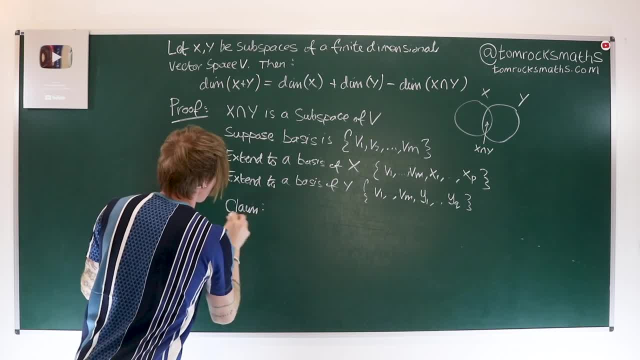 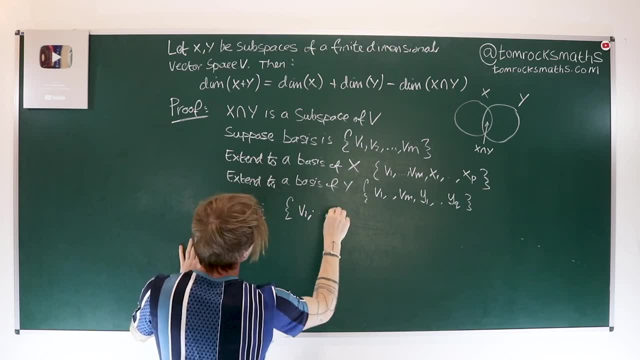 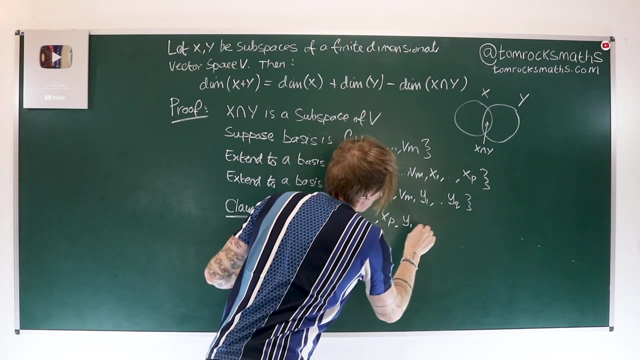 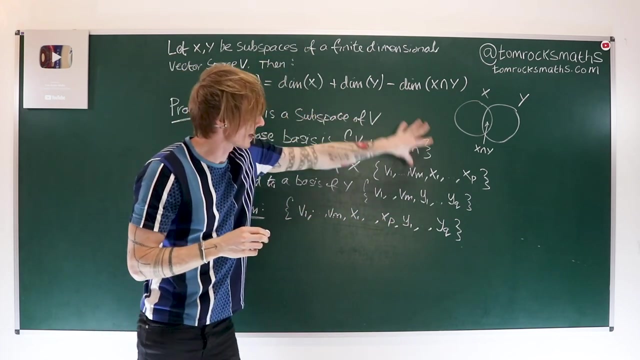 but I will write it as a claim- Is that the following set, given by v1 up to vm, x1 up to xp and y1 up to yq, I'm going to claim that this set, made by combining sort of the three different sets that we have, 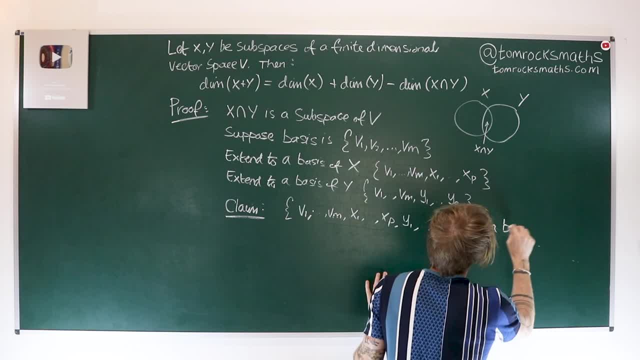 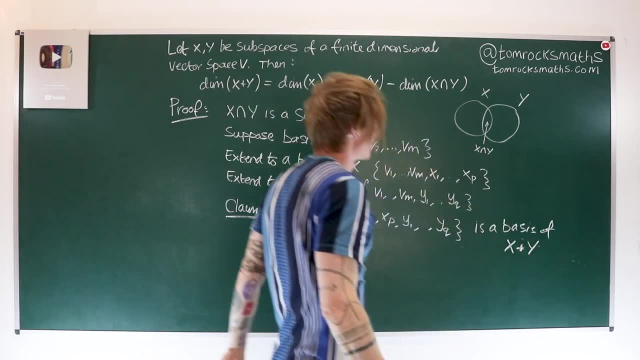 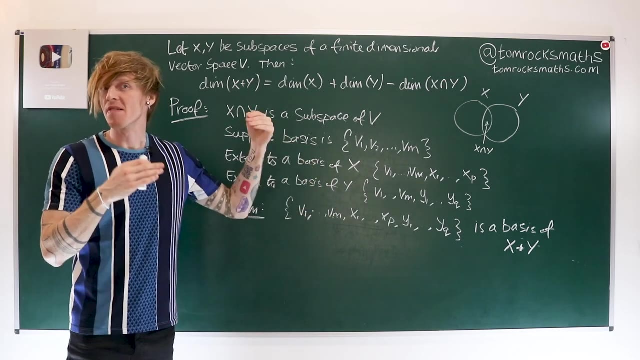 without repeats, I'm going to claim that this is a basis of x plus y. So for the moment let's just assume this is true. Again, we will prove this claim very shortly. But if we assume that it's true, then 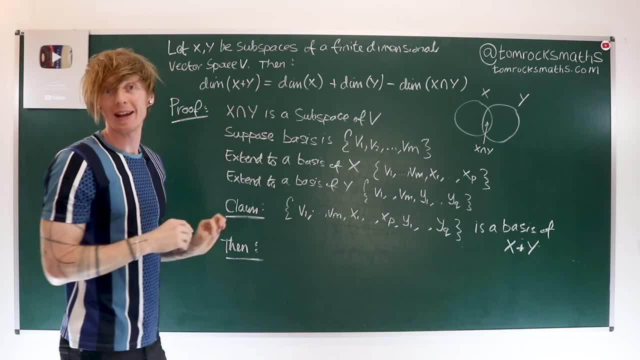 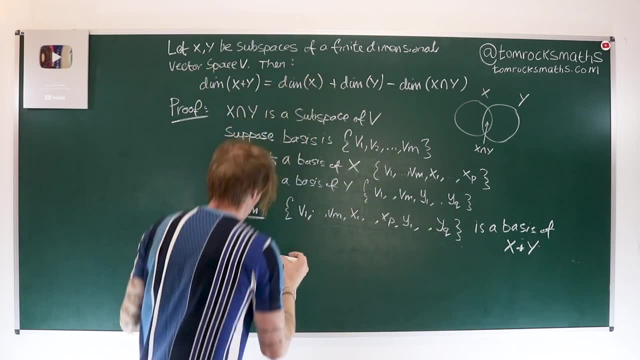 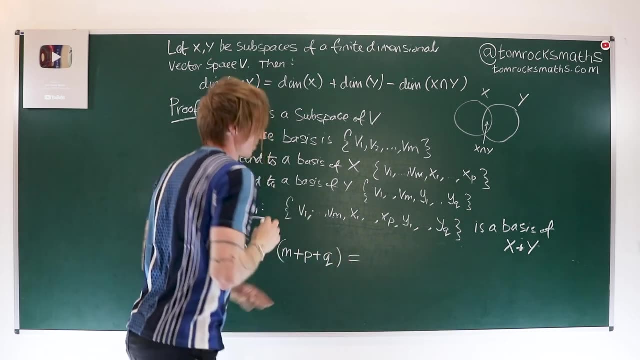 by construction of these general vector spaces, the dimension of x plus y is simply m plus p plus q. So I can say m plus p plus q And we want that, according to what we're trying to prove, to be equal to the dimension of x. 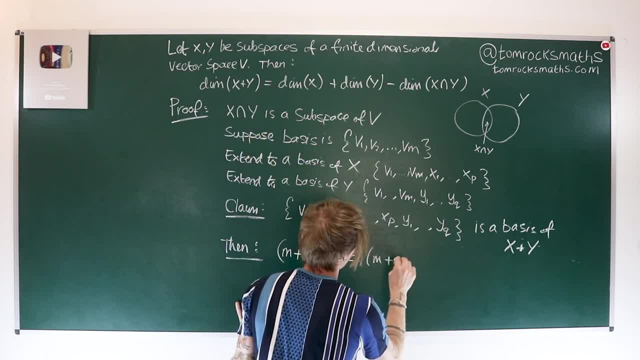 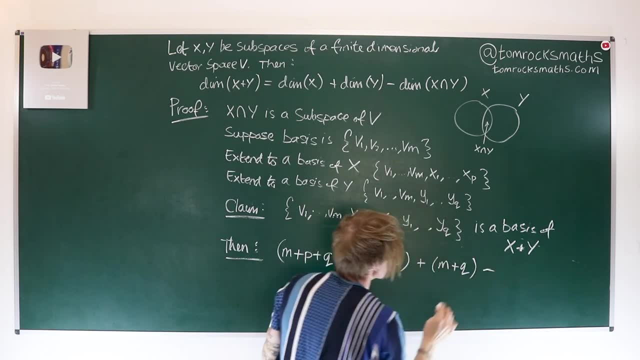 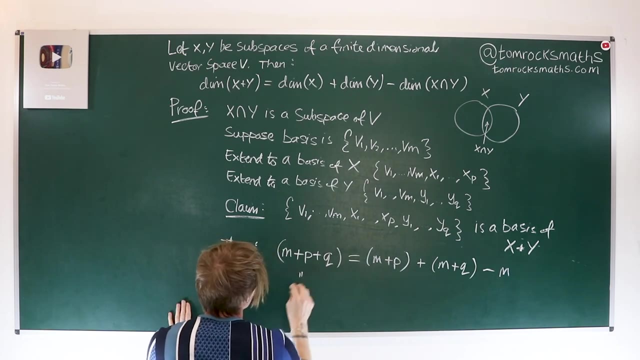 Well, that is m plus p plus the dimension of y. well, that's m plus q minus the dimension of the intersection, which was m. So we're saying here: this is dm of x plus y, provided we can prove that. 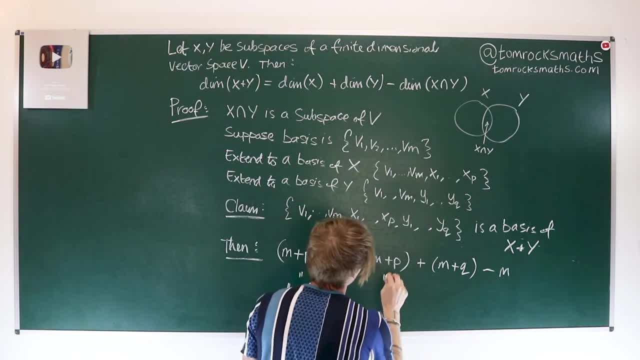 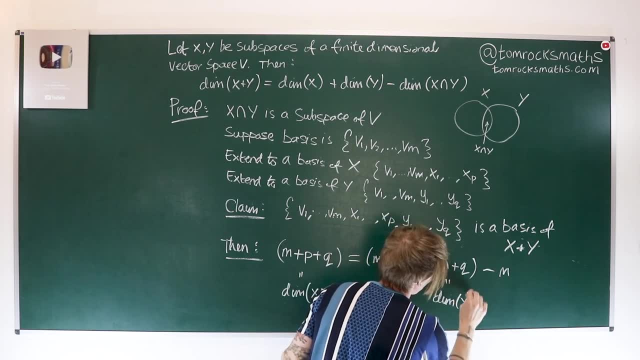 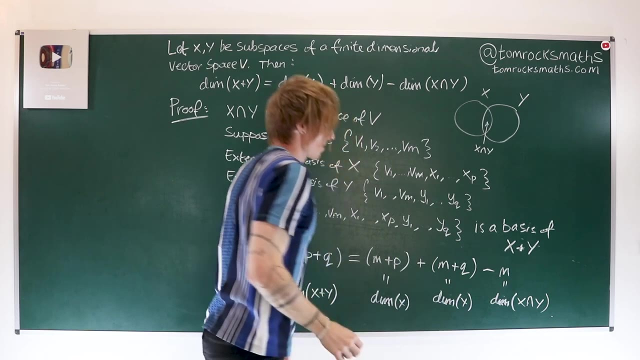 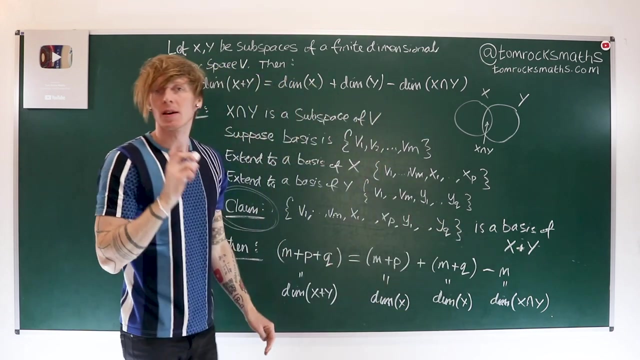 Haven't done that yet, but we will. This is the dimension of x, this is the dimension of y and this is the dimension of the intersection. So, again, provided we can show this is true, provided we can show this is a basis of x plus y. 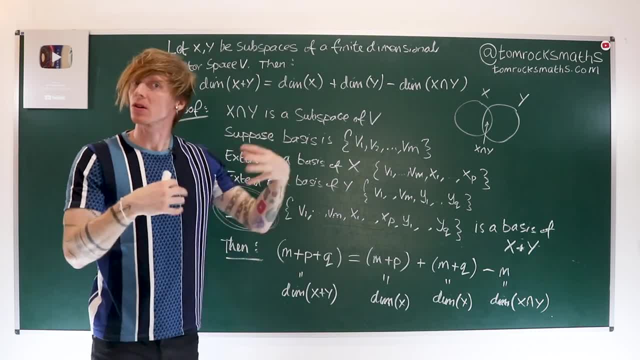 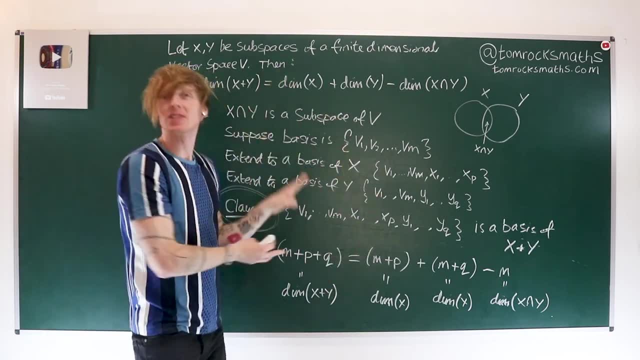 we need to show it's spanning, and linearly independent according to the definition of a basis. But provided we can show that, then this formula holds true in this general case and therefore we will have proven the theorem and proven the dimension formula. 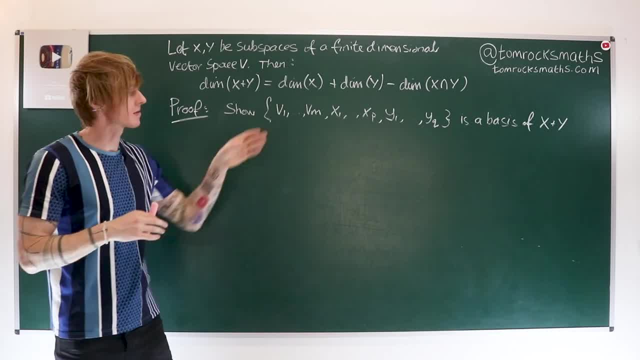 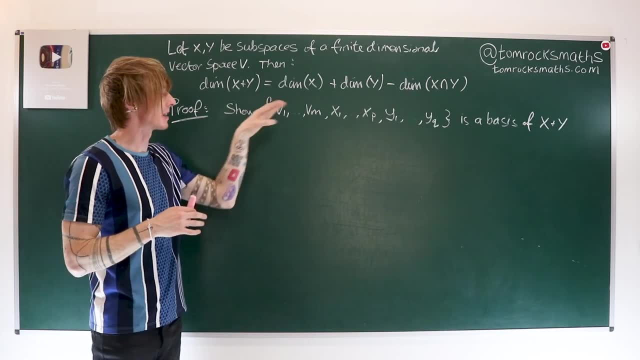 To show this set of vectors is in fact a basis for the vector space x plus y. we have to show two things: It must be spanning and the vectors must be linearly independent. And if you're unsure of the definitions of those two terms, 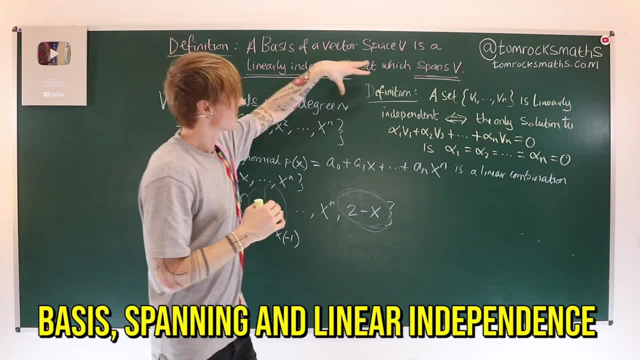 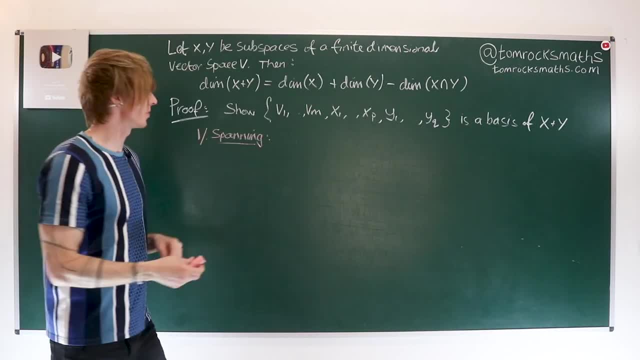 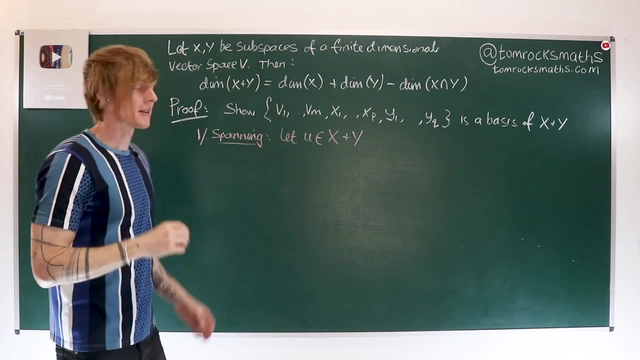 then again, I recommend going back and watching the previous video on basis spanning and linear independence. So let's start with spanning. If we take a general vector, let's call it u, that u belong to x plus y, then this means that 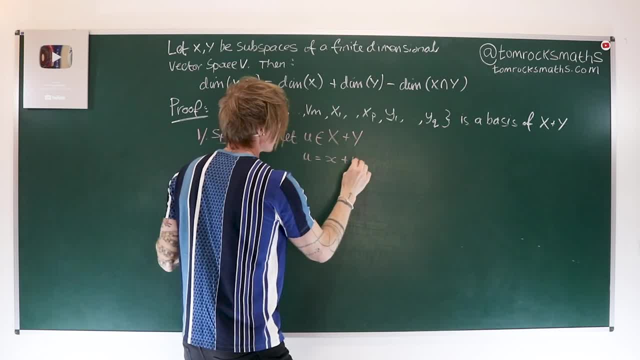 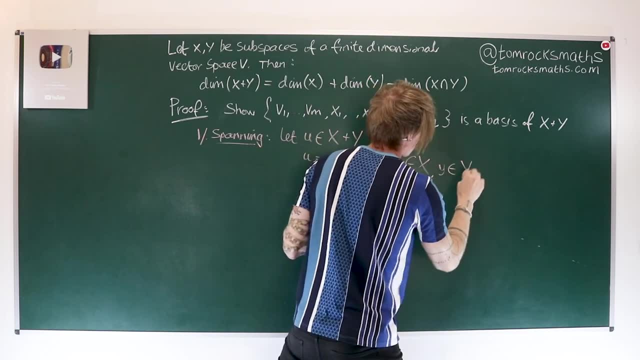 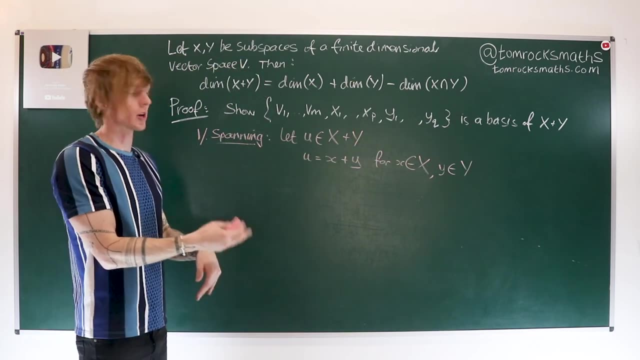 u is equal to some x plus some y, for x in the vector space x and y in the vector space y. Now we already know the basis for x and the basis for y, so, keeping this as general as possible, we can then say: 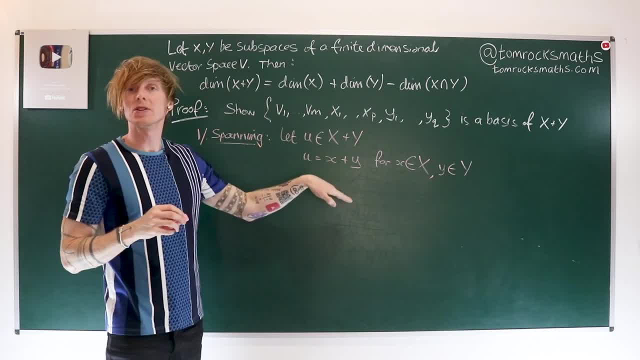 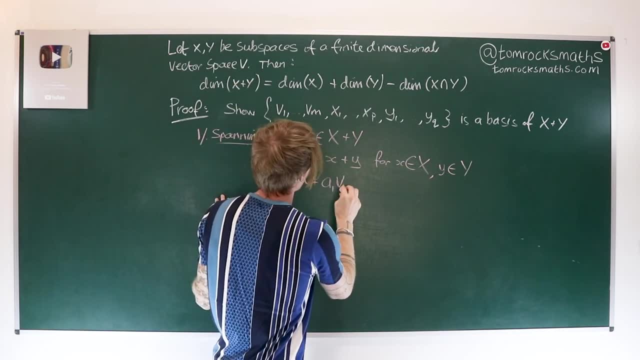 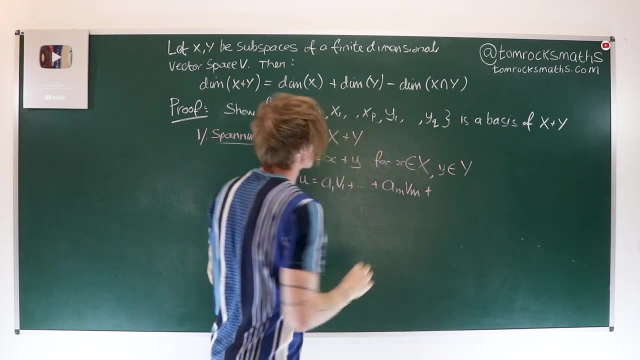 well, that means that u is equal to a linear combination of the basis vectors of x. so let's call it alpha one, v one plus dot, dot, dot up to alpha m, v, m plus. let's call these betas now. 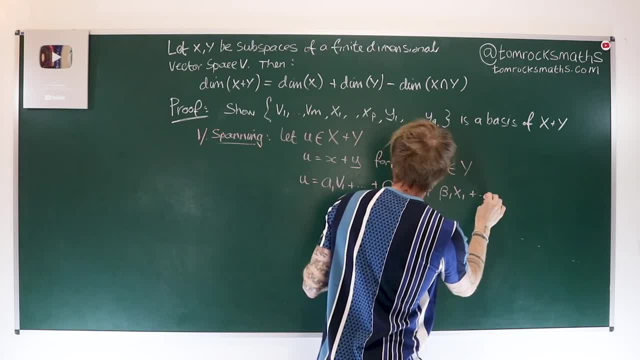 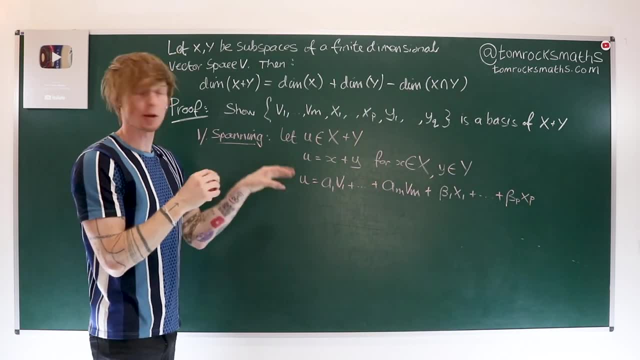 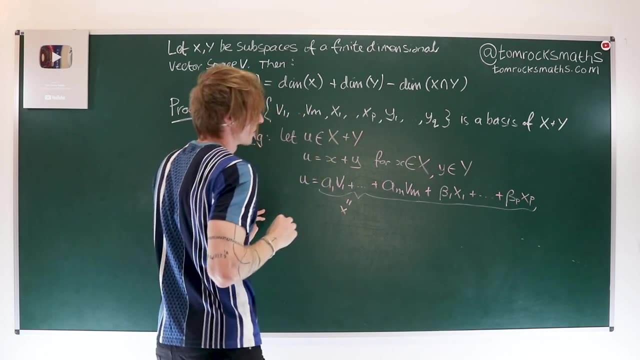 beta one x one plus dot, dot, dot plus beta p x p. So that is the x component, So I can label this. just to make it very clear, This equals the x part of u, And then we can add on the y part. 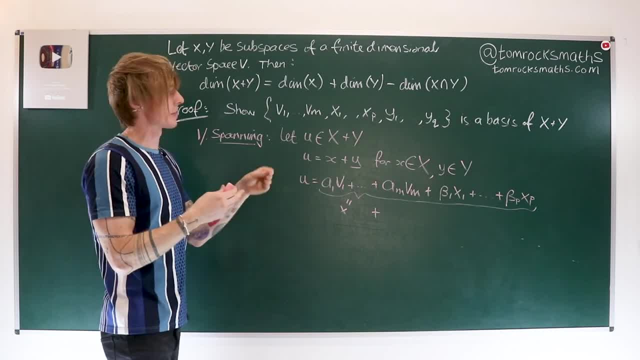 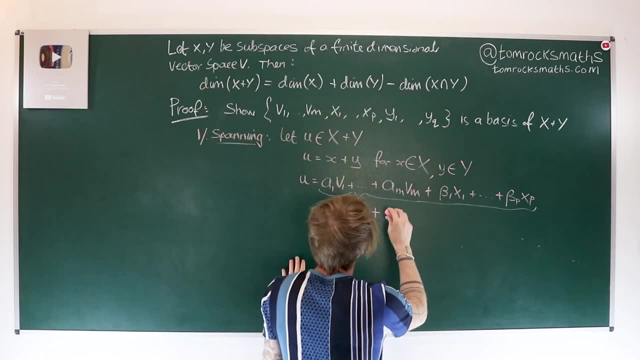 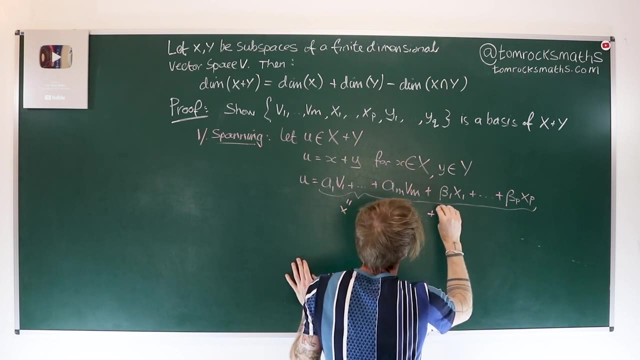 where the y part is again going to be a linear combination of the basis vectors of our subspace, y, which were the v's and the y's, So plus a gamma one, v one plus dot, dot, dot, plus gamma m, v, m. 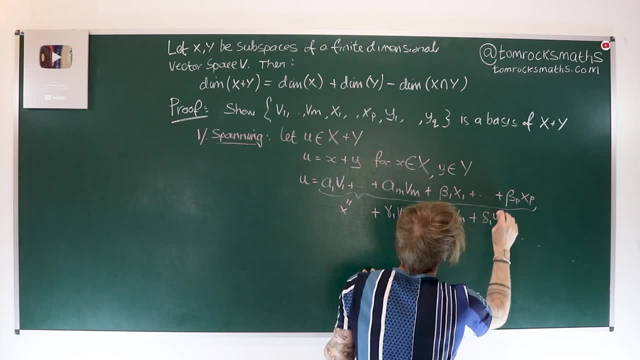 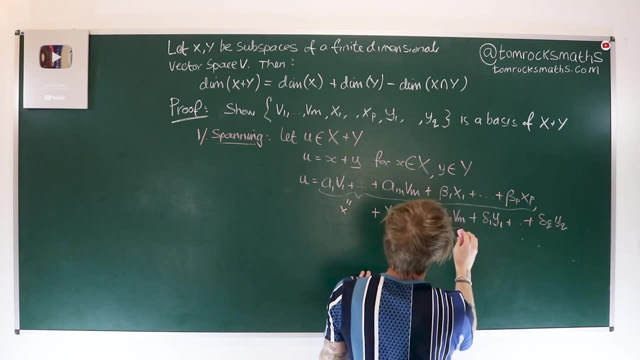 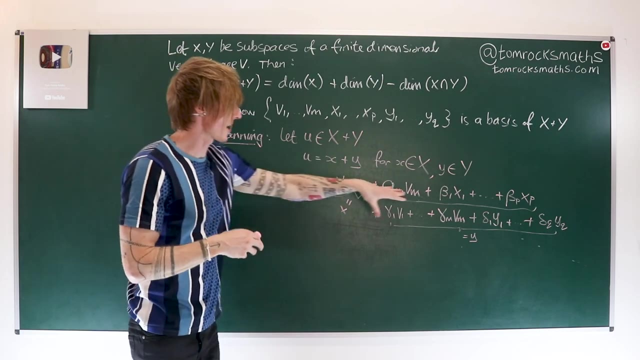 and then plus delta one y, one plus dot, dot, dot. plus delta q, y, q, And then the second part is of course the y part. Now we can group together some of these terms, because we have several copies of each of the v's. 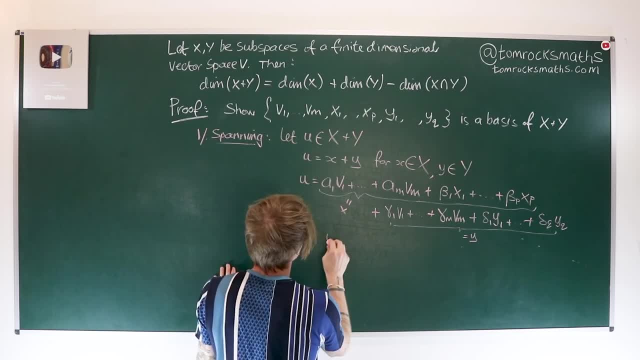 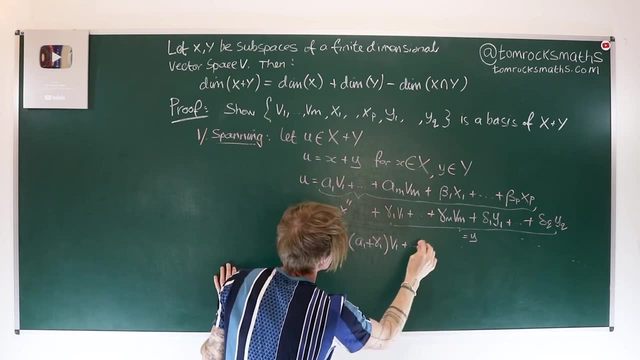 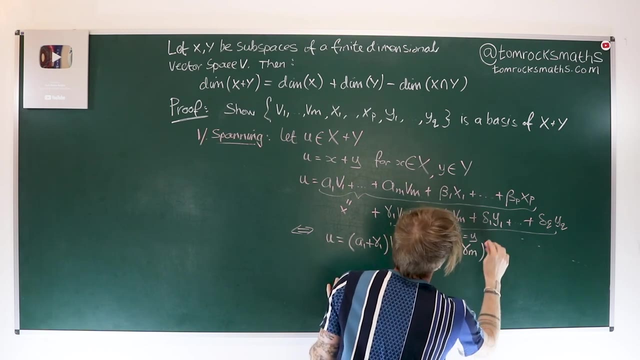 So if we group those together we can say: well, this is actually equivalent to u being equal to a one plus gamma, one times v, one plus dot dot dot plus a m times gamma m. a m plus gamma m, even times v m. 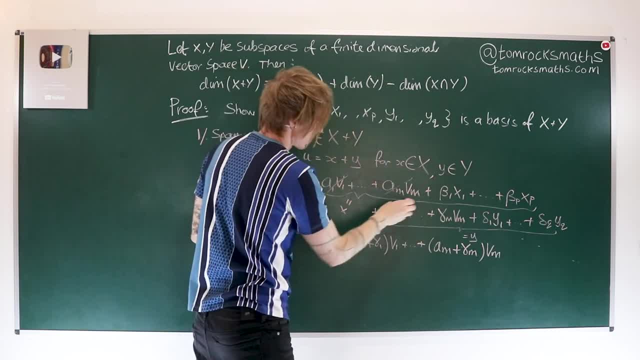 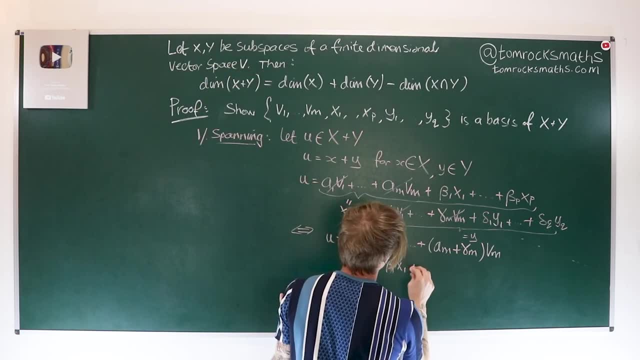 So that covers all of the v terms. So we've crossed off these. Then we've got some amount of all of the x's. So plus beta, one x one, plus dot, dot, dot, plus beta p x p, That's all of them. 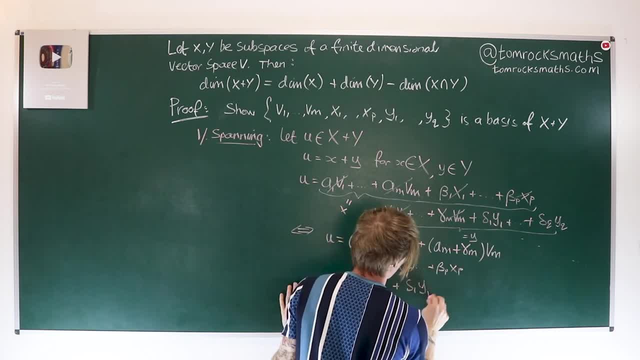 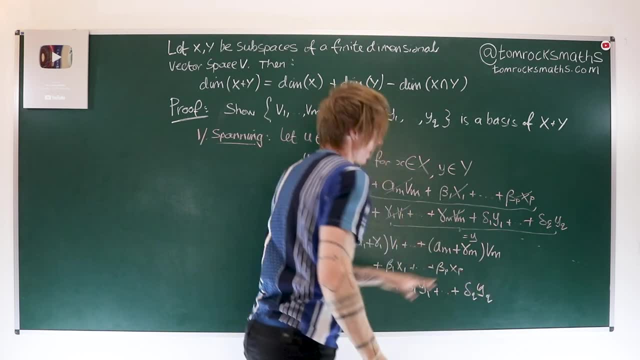 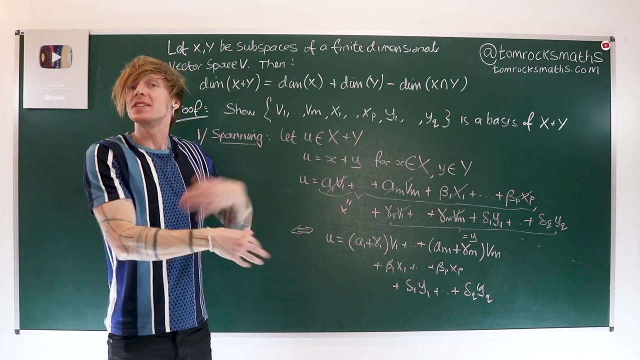 And then we've got the y's. So plus delta one y one, plus dot, dot, dot, plus delta q y, q. But that, of course, is exactly a linear combination of our basis vectors, or the set of vectors we're trying to show is a basis. 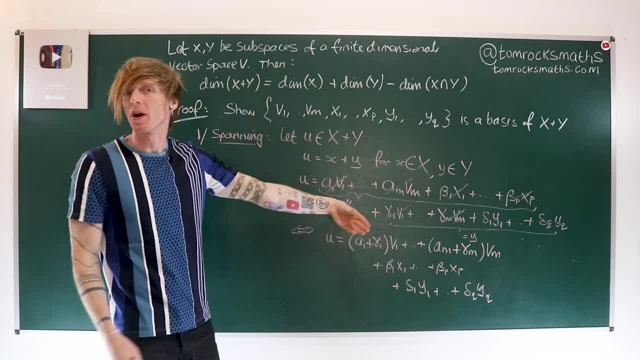 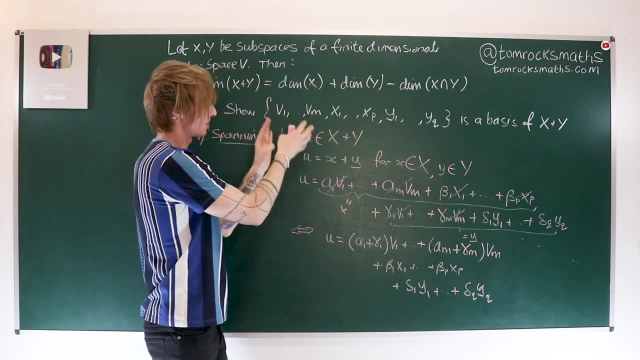 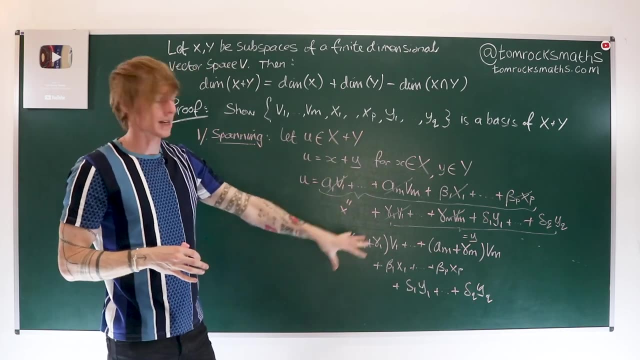 Because we've got two constant amounts of v one added together. but that is still some amount of v one. So we took the most general possible vector u that belonged to the sum of our vector spaces and we were able to rewrite it as a linear combination. 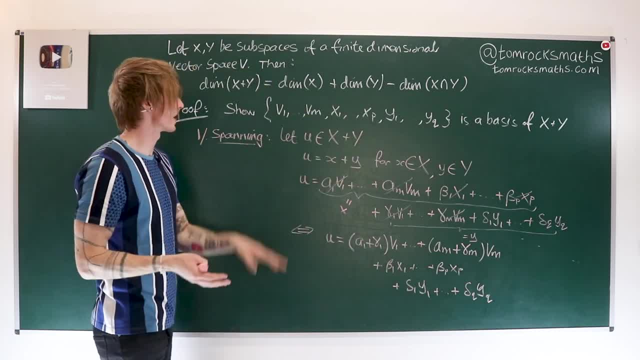 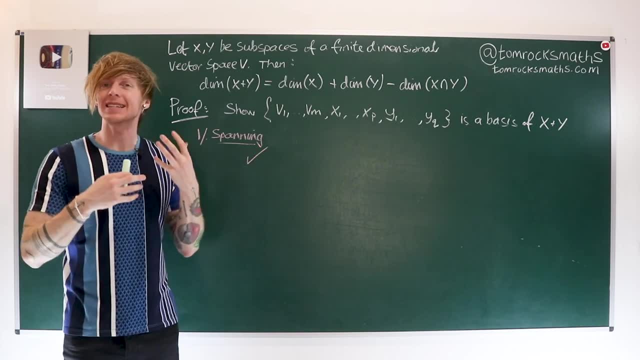 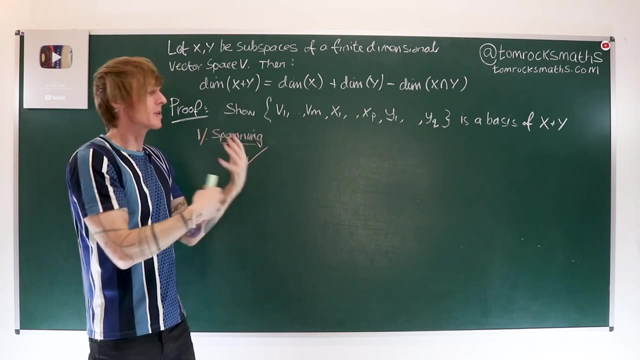 of just the vectors in this set. Therefore we can say: spanning is going to hold. Now for linear independence. we need to show that, given any linear combination of these vectors equal to zero, then we must in fact have all of the coefficients themselves equal to zero. 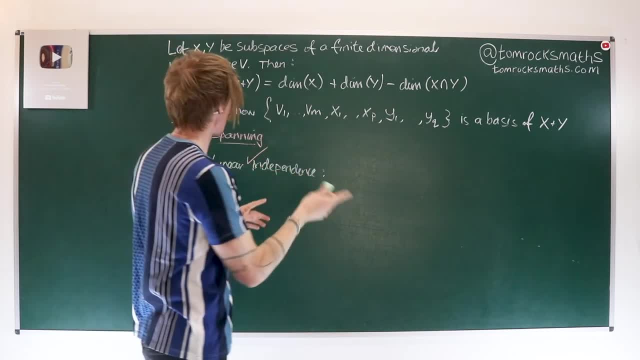 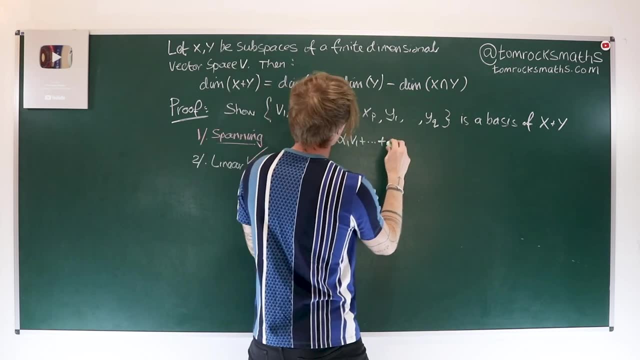 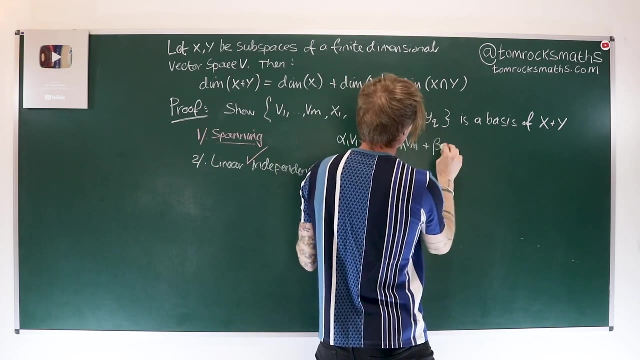 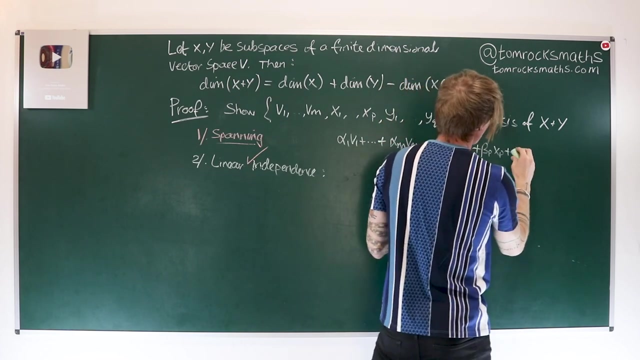 So, writing that out, we consider exactly that linear combination. So let's suppose we have alpha one v one plus dot dot dot plus alpha m, v, m plus beta one x one plus dot dot dot plus beta p x, p plus gamma one y one. 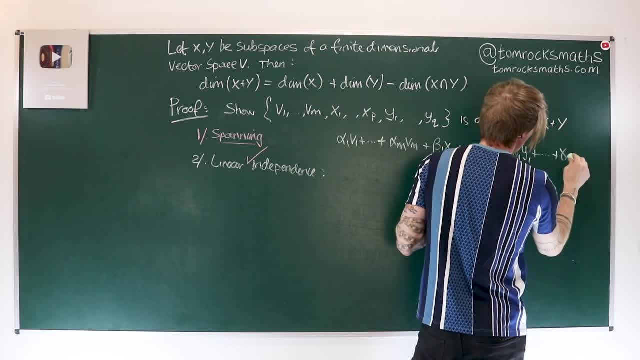 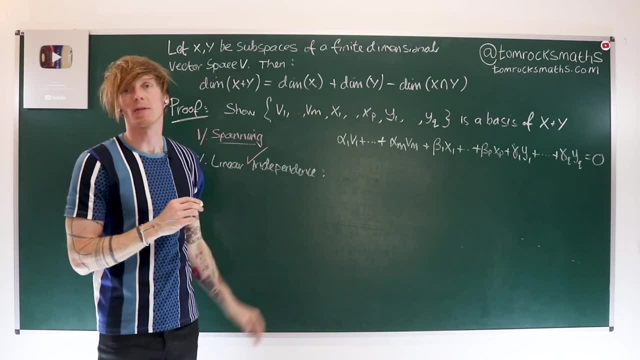 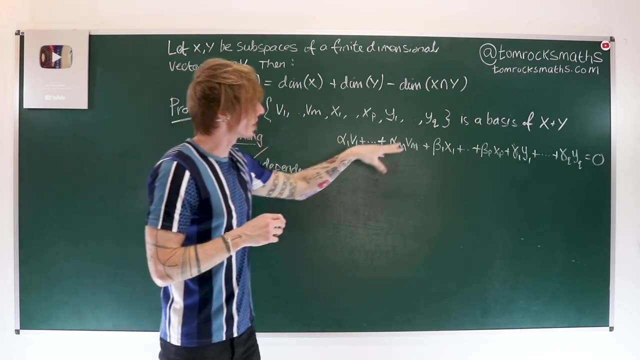 plus dot, dot dot, plus gamma, q, y, q, And let's suppose this linear combination is equal to zero. Now, in order to show linear independence, which is what we want, then we have to show: the only solution to this equation is for all of our coefficients. 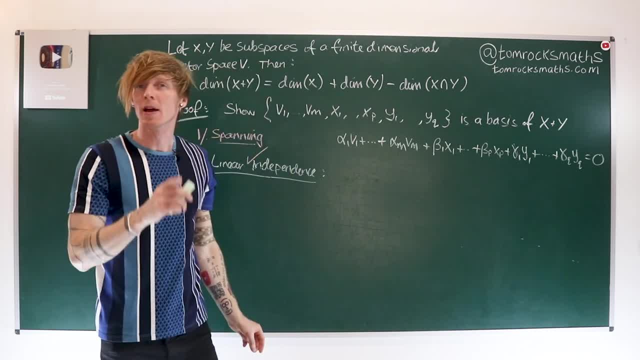 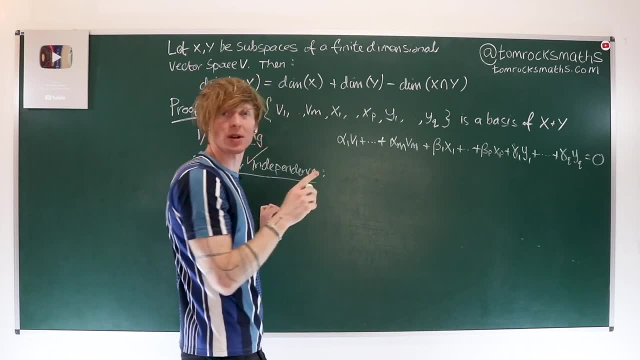 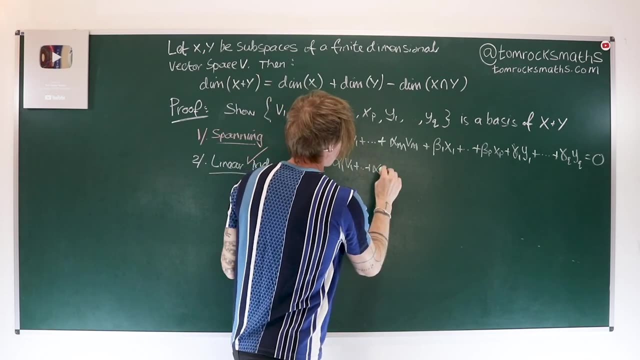 the alphas, the betas and the gammas to all be identically zero. So what I'm going to do to start with is actually rearrange this equation ever so slightly, So I can say alpha one v one plus alpha m v m. 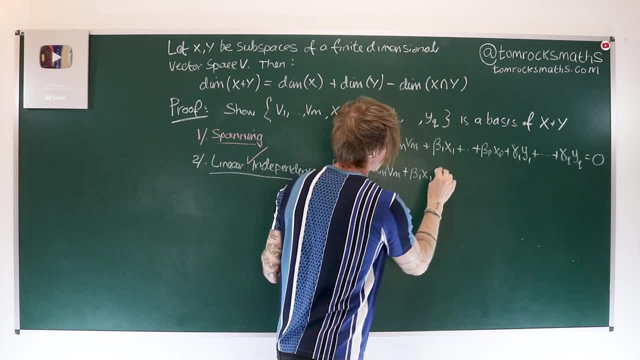 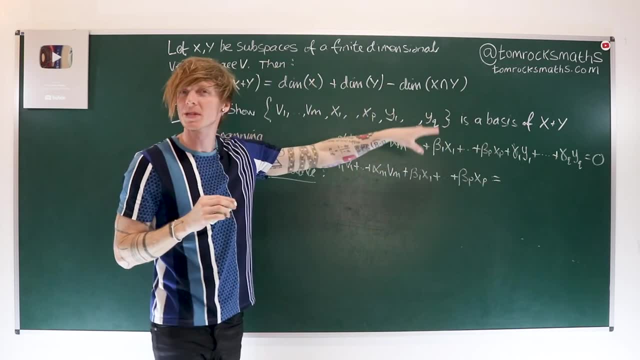 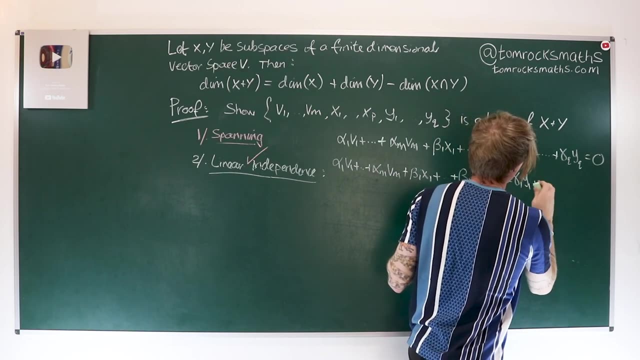 keep the x's here. so plus beta one x one plus dot dot dot. plus beta p x p. But if I now take the terms in y across, so they now become negative, is equal to minus gamma one y one plus dot dot dot. 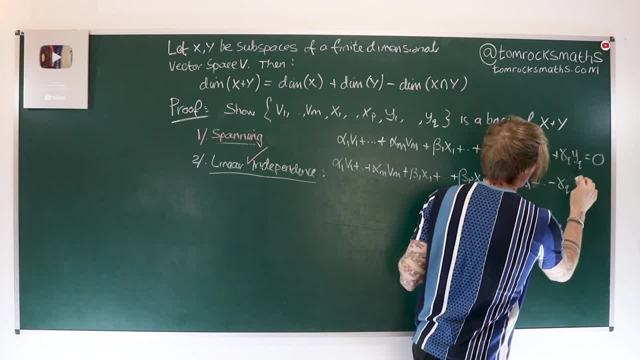 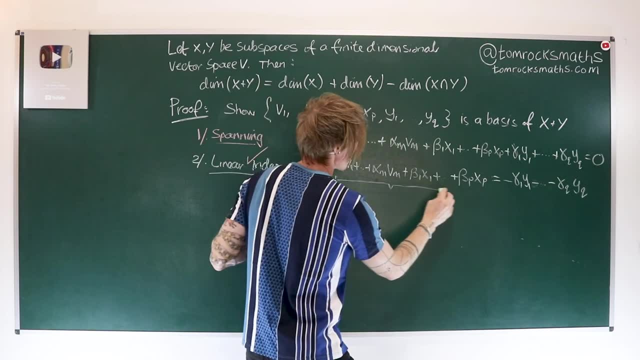 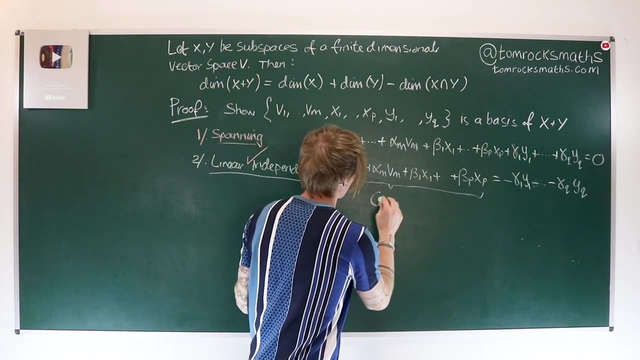 not plus minus dot, dot, dot, minus gamma, q, y, q. So what I have now is a combination here, a linear combination of vectors v's and x's, which is exactly the basis of x. So this belongs to our space x. 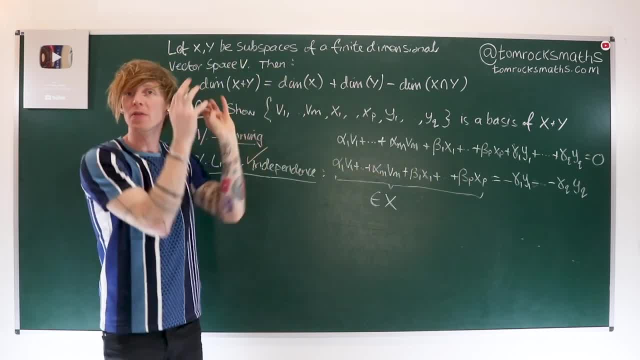 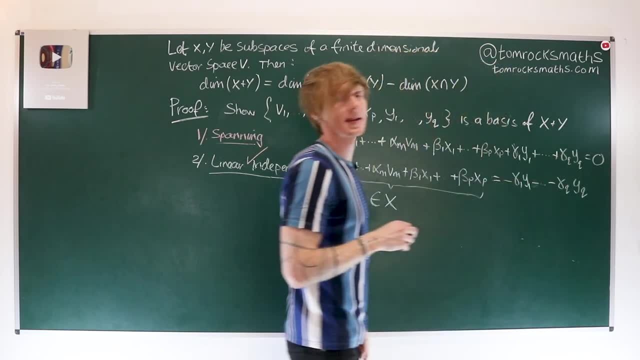 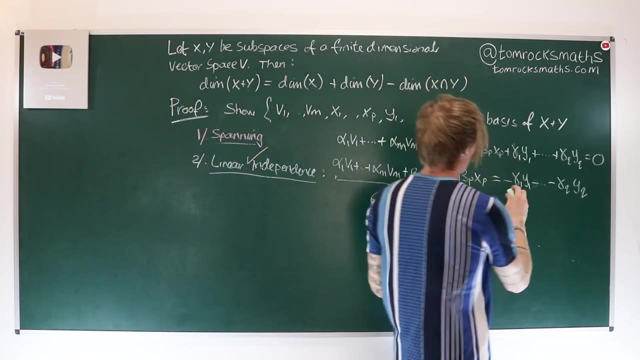 because it's a linear combination of the v's and the x's and those together form the basis of our space x And over here I have a combination of y's. now the y's only appeared in our original three bases inside the space y. 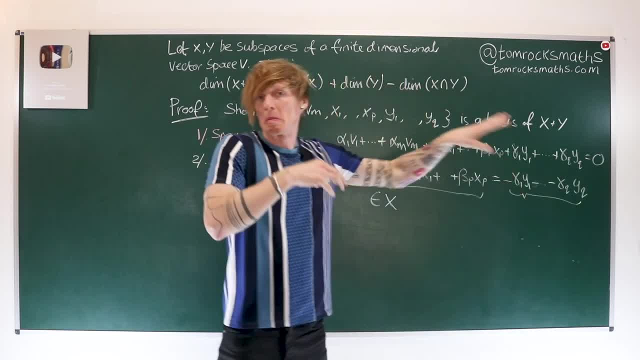 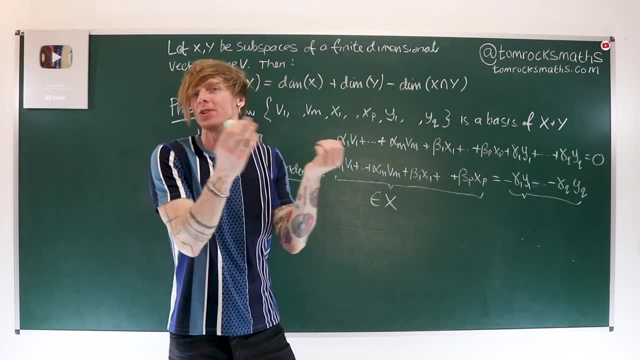 So this is a combination of part of the basis vectors of our space y, so therefore it still belongs to the space y. You can think of it as all the other coefficients being zero, if that helps, But either way, this is definitely in y. 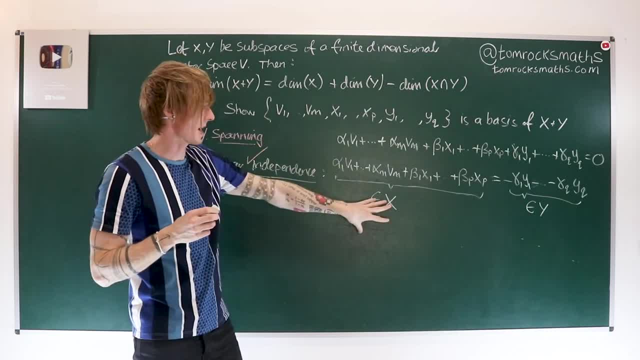 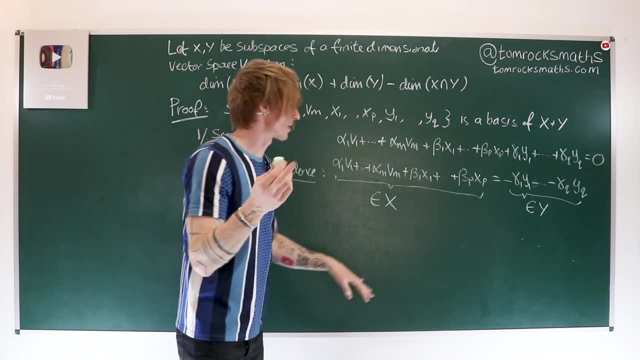 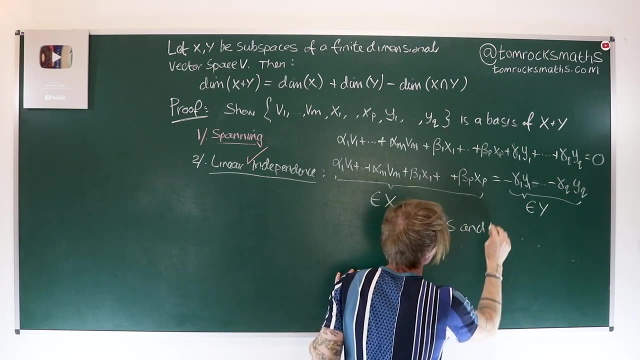 So the left hand side is in the space x. it's equal to the right hand side, which is in the space y. So therefore, in fact, both both left hand side and right hand side, which again are equal. 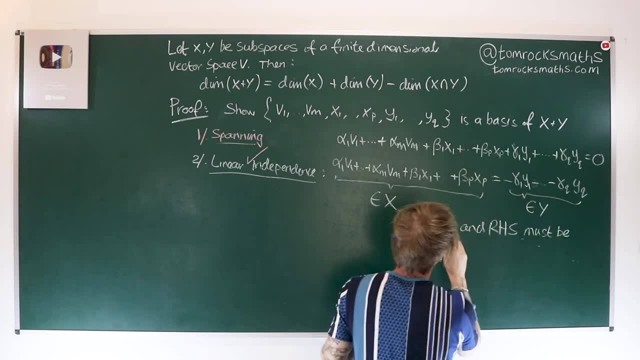 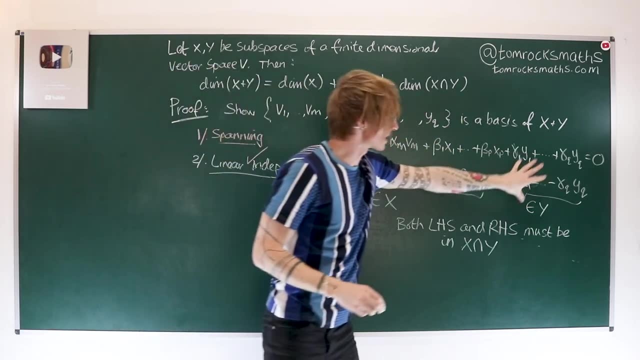 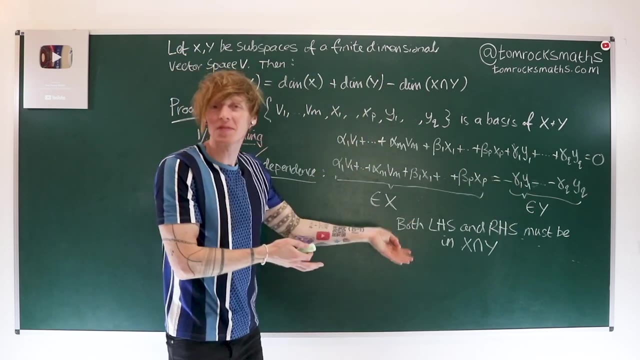 must be in the intersection Because, again, the left is definitely in x, the right is definitely in y, but they're equal. So something in x equal to something in y, something in y equal to something in x, Clearly both of them belong to both. 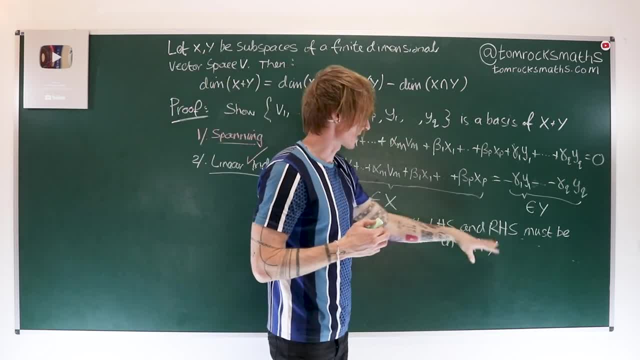 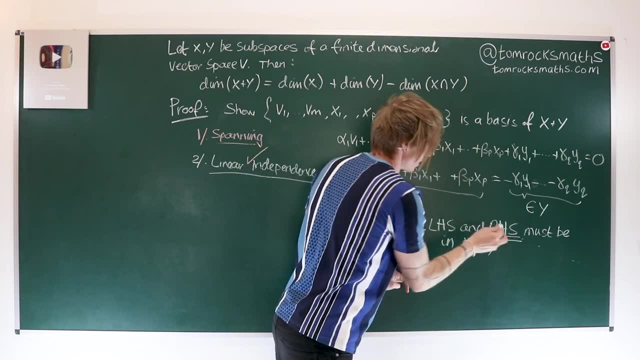 x and y. So we can say the left hand side is in x intersect y, as is the right hand side. Now, the right hand side is actually where we're going to start. So we know this thing, which is written as: 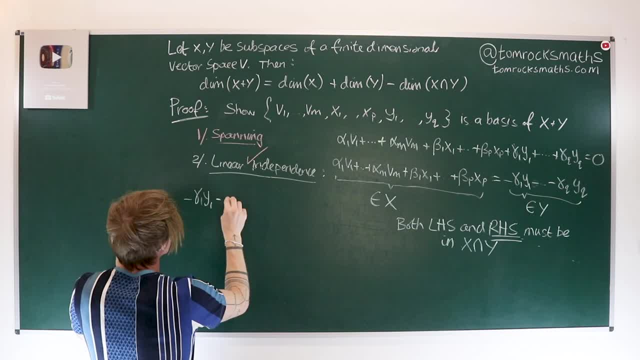 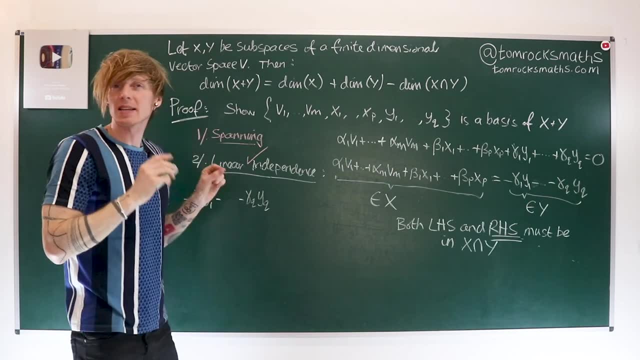 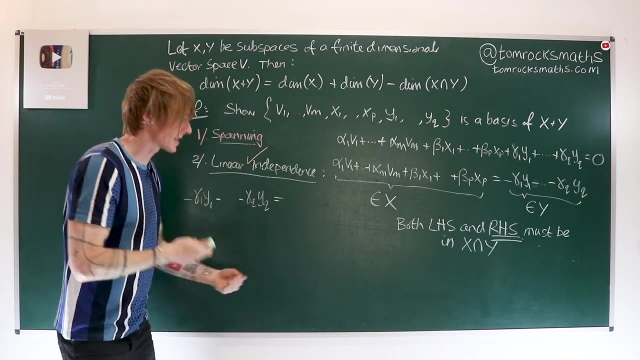 minus gamma 1, y1 minus dot, dot, dot. minus gamma q, yq. This is in x, intersect y. So that means this can be written as a linear combination of the basis vectors of the intersection. Now, those basis vectors were the v's. 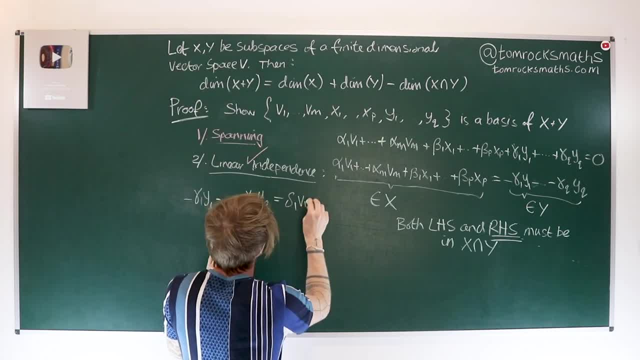 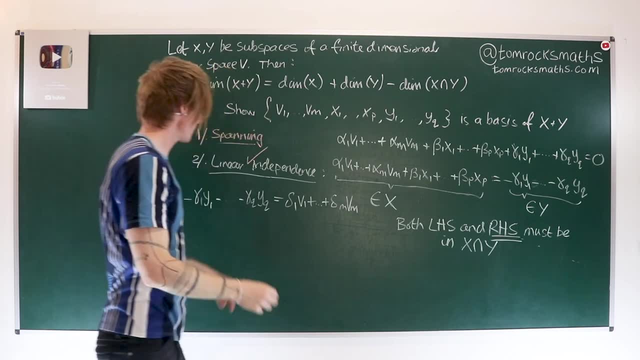 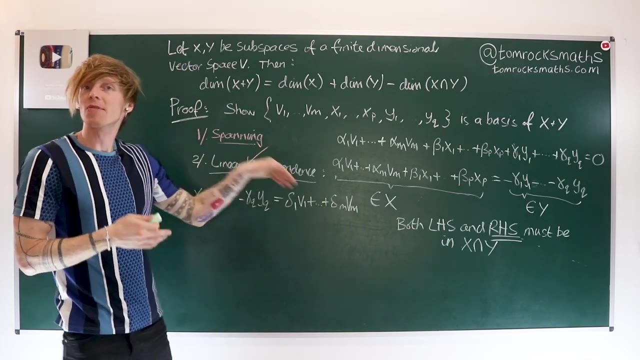 So this is equal to some combination of the v's. Let's call it delta 1 plus dot, dot, dot up to delta m, v, m. So again, this we know is in the intersection from our calculation over there. This is a general way of writing something. 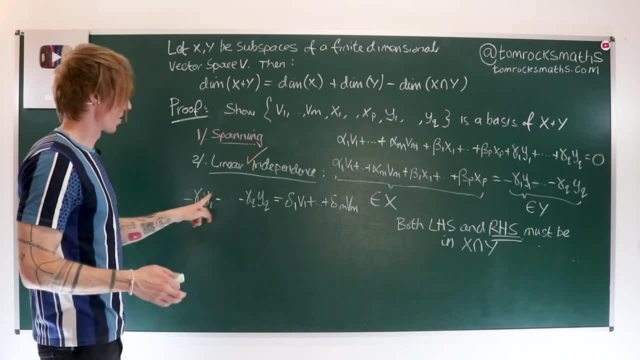 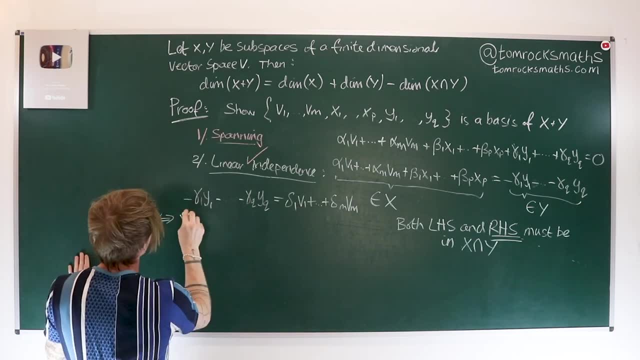 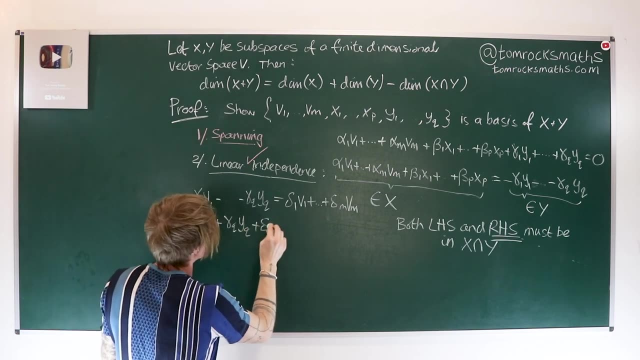 in the intersection. But now, if I take all of the y's across to the right hand side of this expression, that's then equivalent to saying gamma 1- y1 plus dot, dot, dot plus gamma q- yq plus delta 1- v1 plus dot, dot, dot. 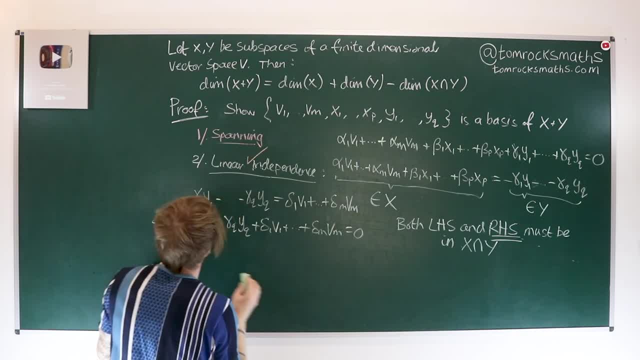 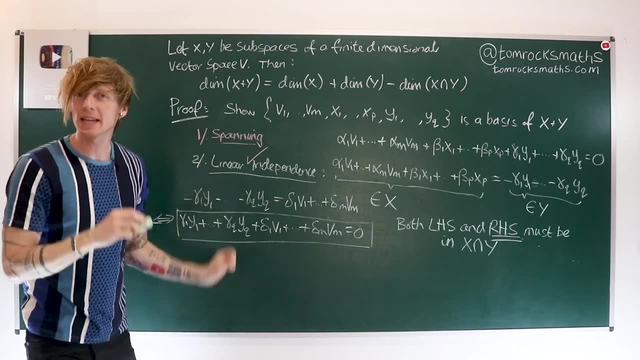 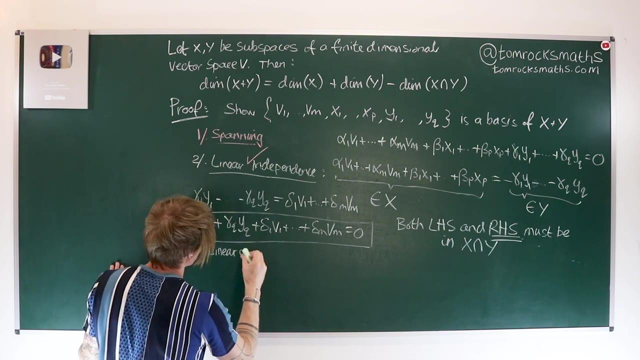 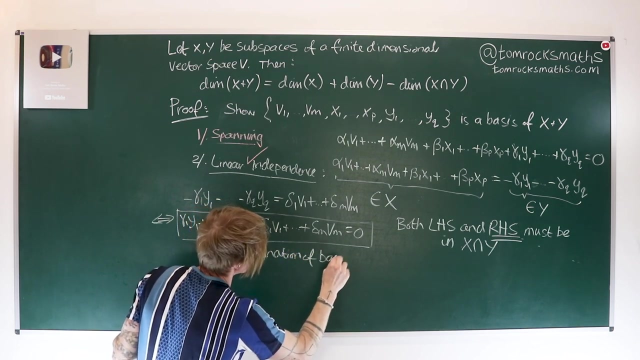 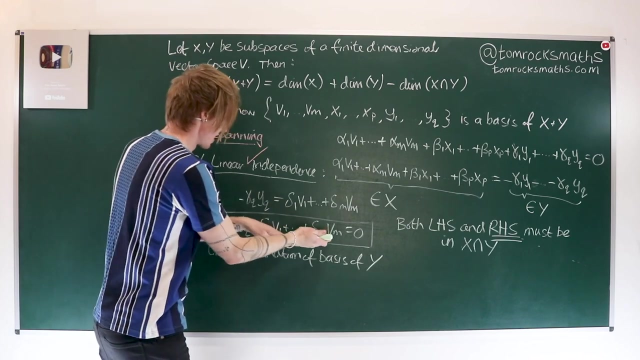 plus delta m, v, m is equal to zero. Now this expression here. this is a linear combination, so let's write this out. This is a linear combination of the basis vectors, of the basis of y. So the basis of our space, y, consisted of the v's. 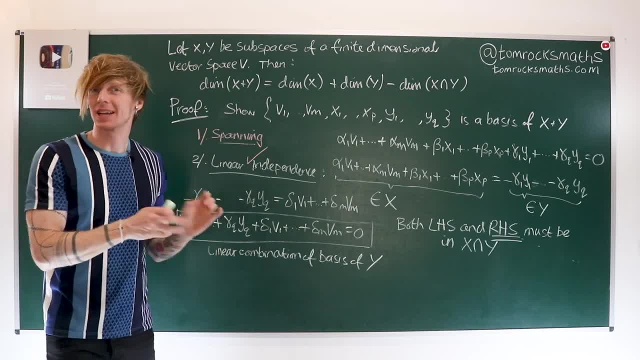 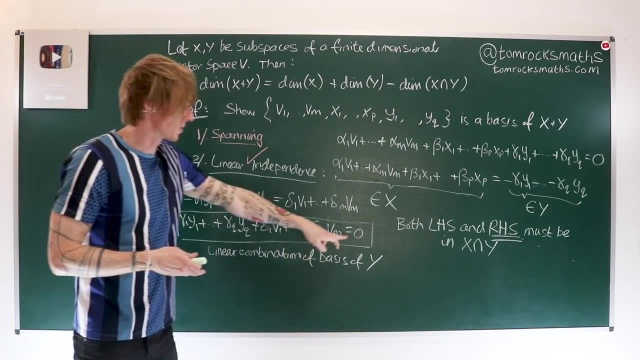 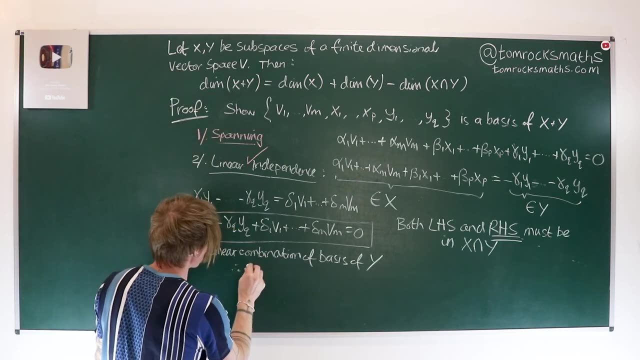 and the y's, And we know that is a basis That is confirmed. So if we have a linear combination of the vectors in the basis of y equal to zero, we know they are linearly independent. So therefore, all of the coefficients. 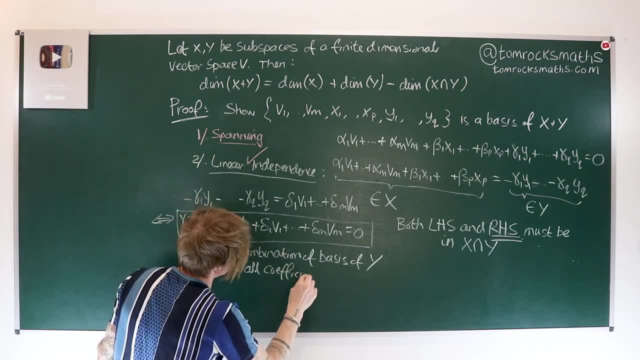 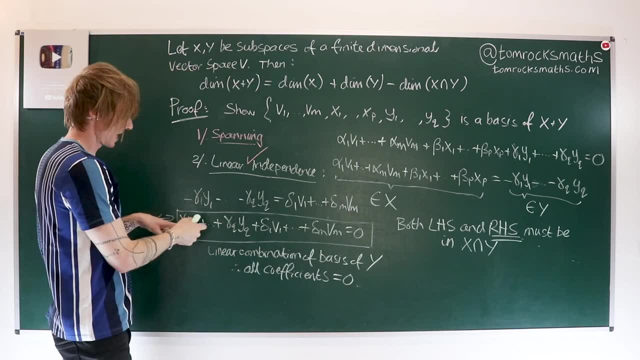 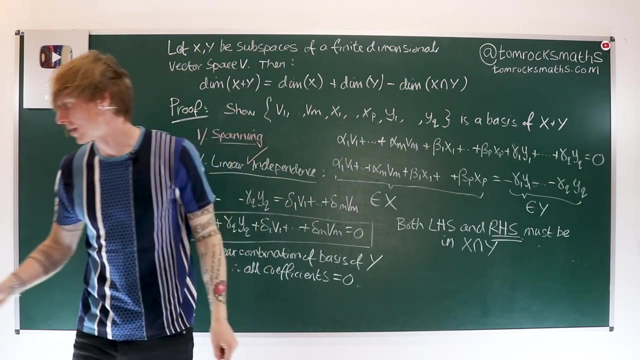 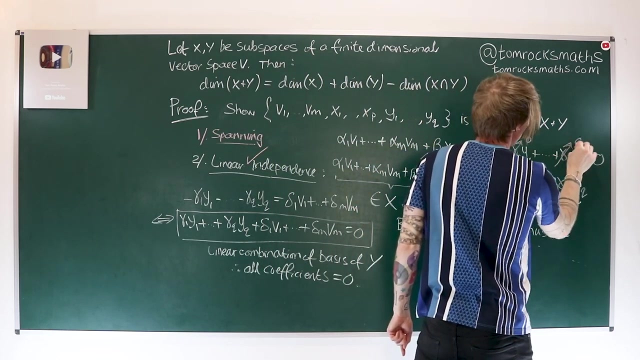 are zero. So, importantly, that tells us our gammas here are in fact zero. So, going back to my original expression up here- and I'll use a different color to express this- we can actually say these are zero. So we've managed. 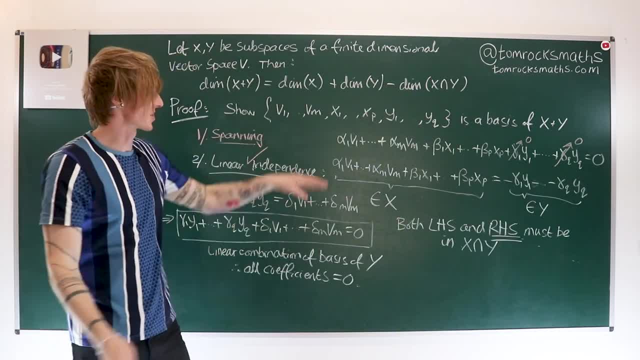 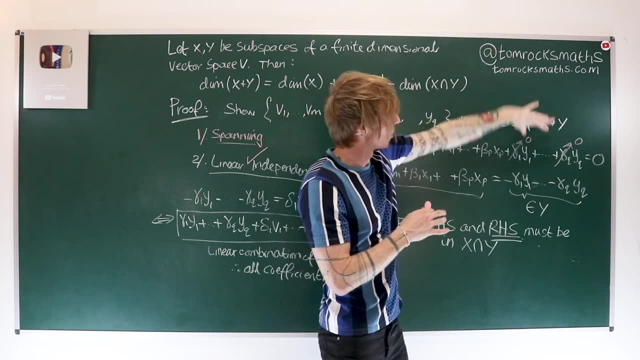 to show one third of the possible coefficients, because we're trying to get all of the alphas to be zero, all of the betas to be zero, and we've just shown successfully, all the gammas are in fact zero. So just to reiterate that one final time. 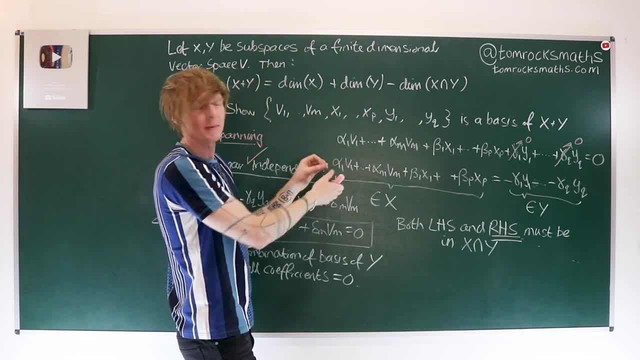 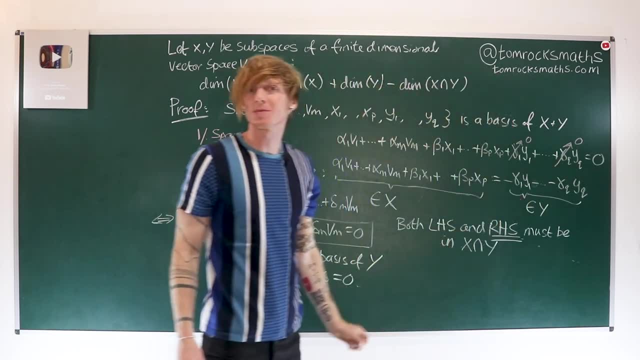 we rearrange this equation to get something on the left that's in x, because it's a combination of the x basis vectors, and something on the right, which definitely belongs to our subspace y. So therefore both sides of the equation belong to the intersection. 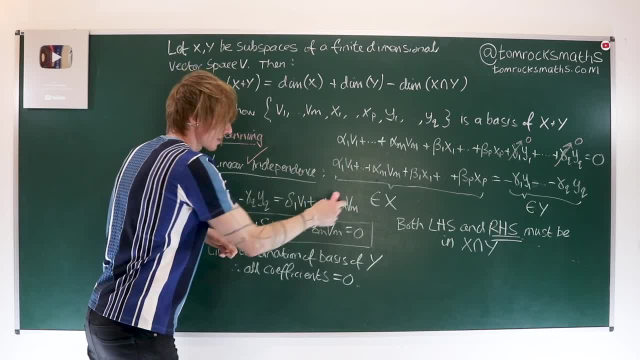 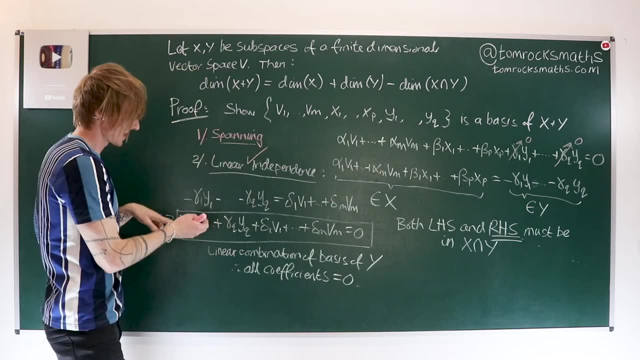 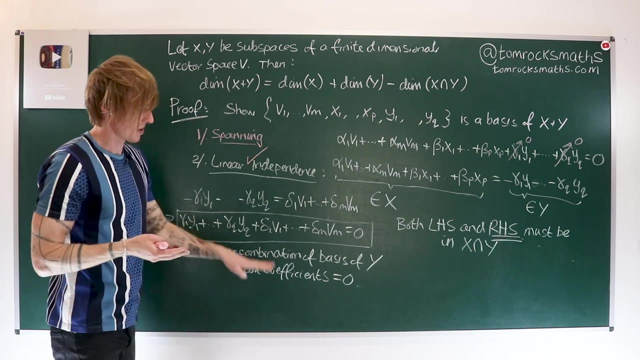 The intersection has a basis given by the v's, so we can rewrite the right hand side in terms of the v's. However, rearranging this gives us exactly the condition of linear independence and therefore, because this is the basis of y, we get all. the coefficients are zero. 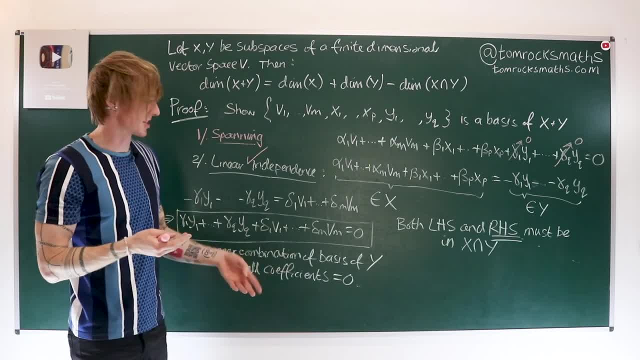 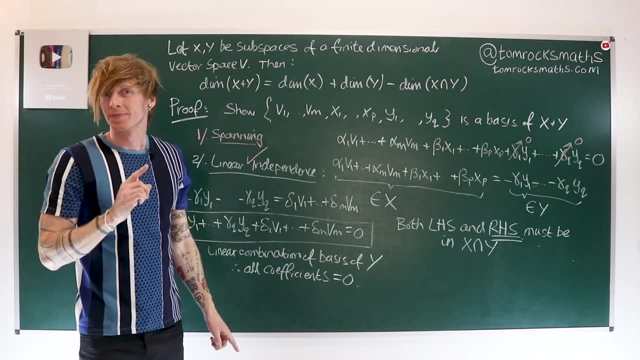 So we also get the deltas are zero. but we don't really care about the deltas, we only introduce them to help us to show that the gammas were zero, which is what we did in fact want. Now all that's left is to show that both alpha and beta 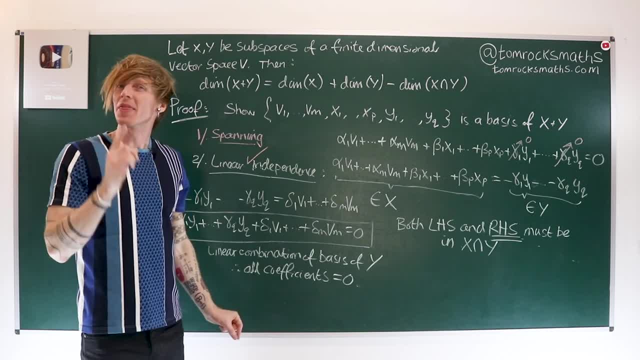 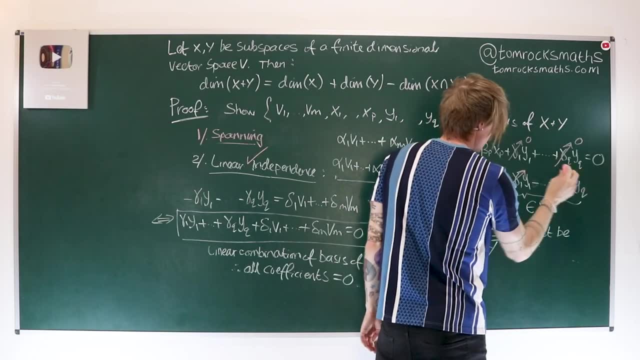 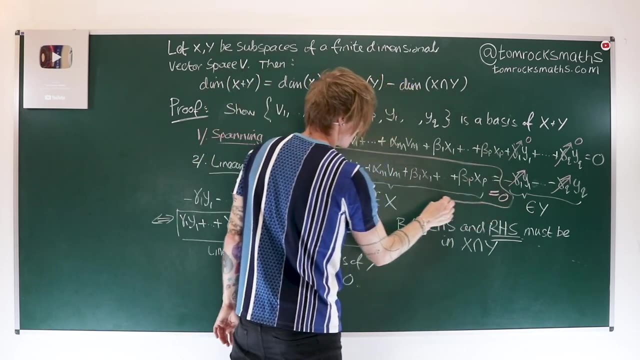 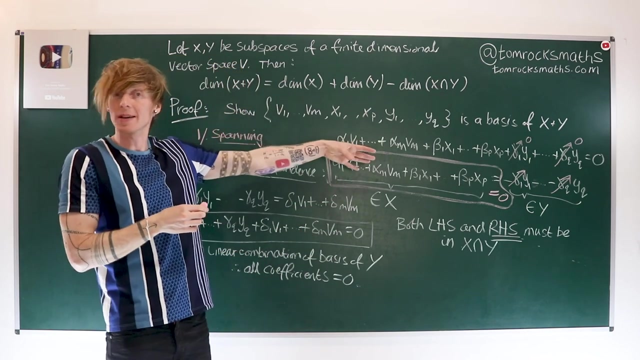 are also zero, But that actually follows quite quickly, because these are zero now here, and so what we've got- and I'll highlight this in red- now this or this whole thing is equal to zero. So the left hand side of our expression from earlier. 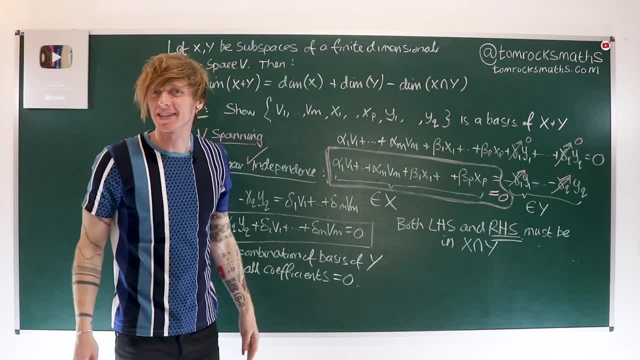 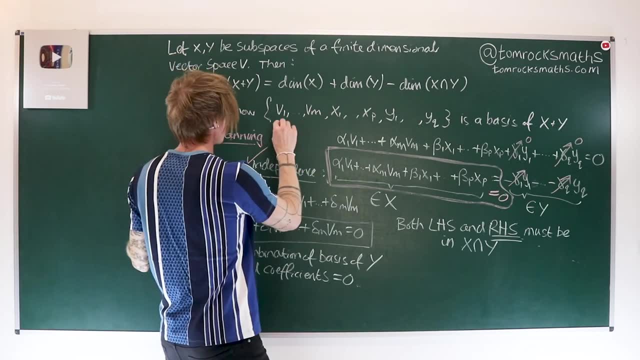 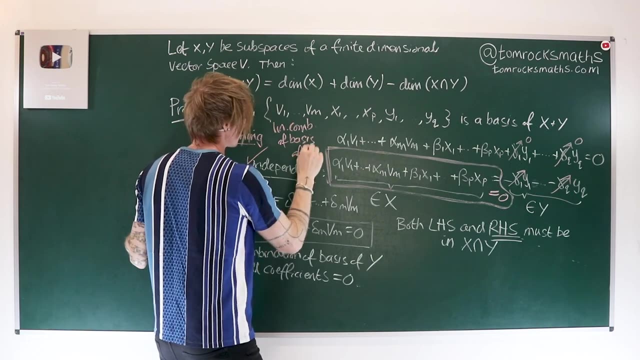 is unchanged. but the right hand side we've now actually shown is in fact zero. But what is the left hand side of our expression? This is exactly a lin combination of the basis of x. The basis of x is made up of the v's. 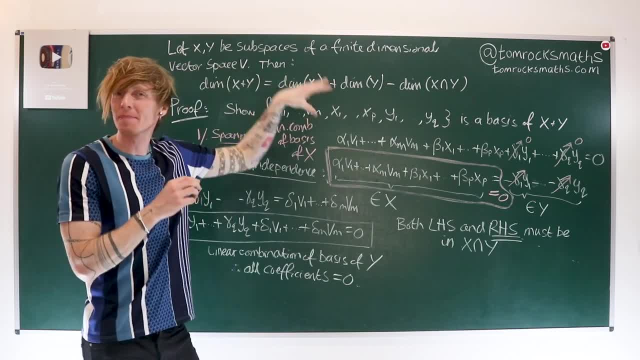 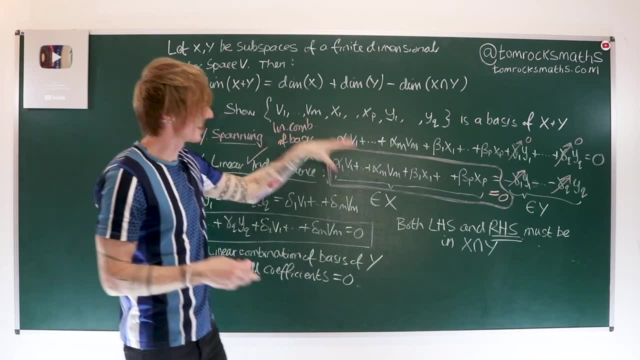 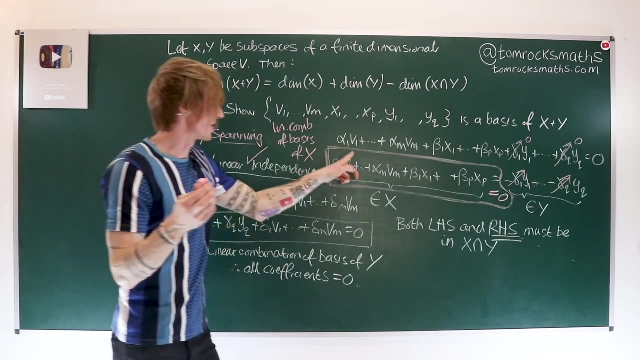 plus the x's. So we have a linear combination of the basis vectors of our space x equal to zero by definition of being a basis. these are linearly independent and therefore all of these coefficients themselves must in fact be zero. So this gives us, therefore, the alpha i equals zero. 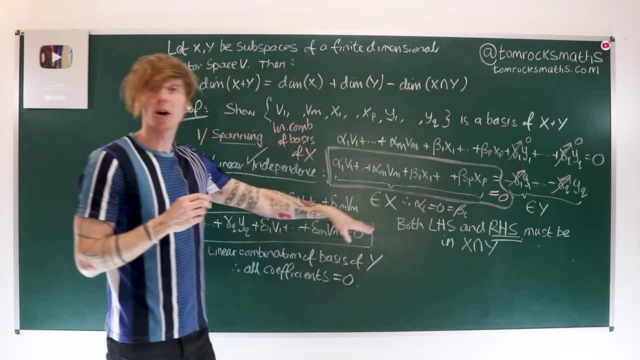 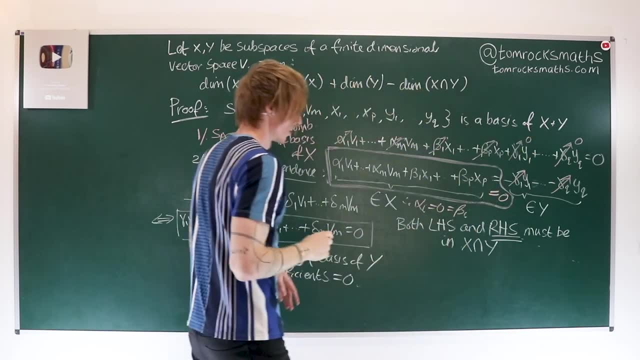 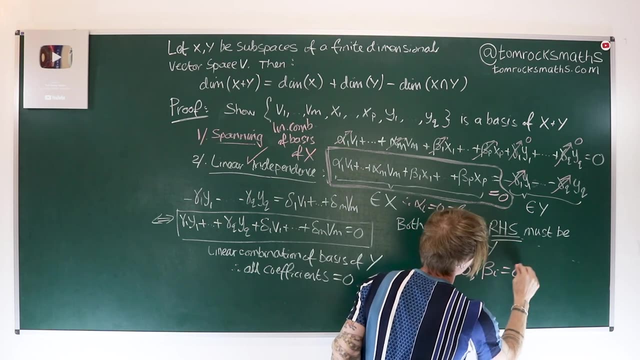 as do the beta i. So we finally have: the beta's are zero, the beta's are zero, and therefore we've got the alpha i equals naught beta i equals naught gamma i equals naught for all. i therefore linear independence, which is what we were trying. 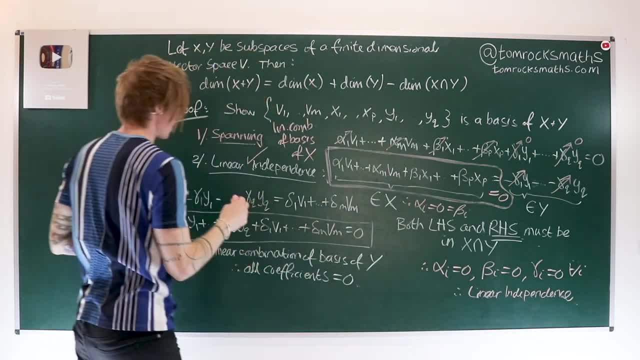 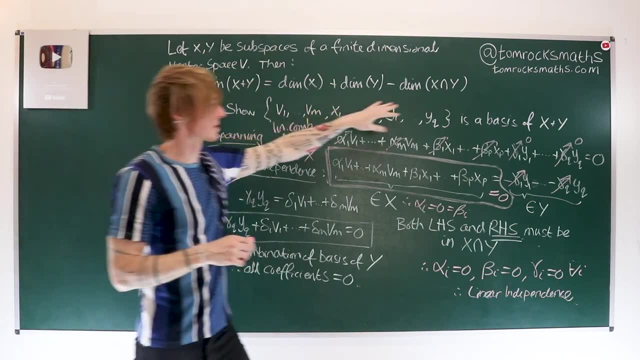 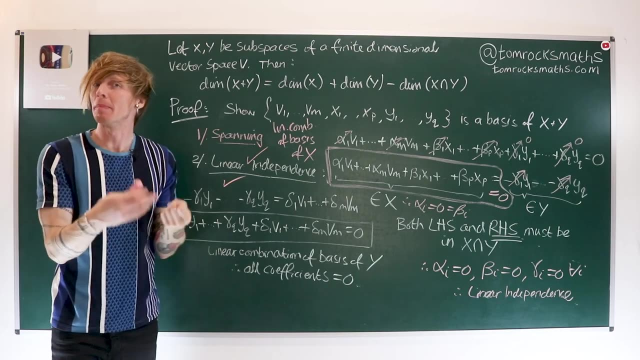 to show So spanning. we've already got linear independence shown, so therefore this set which we wanted to show was a basis of x plus y. we've been able to show is both spanning and linearly independent and therefore, by definition, is indeed a basis, Now that we've shown the claim. 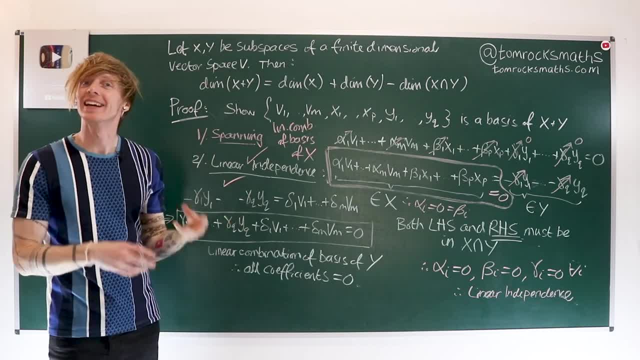 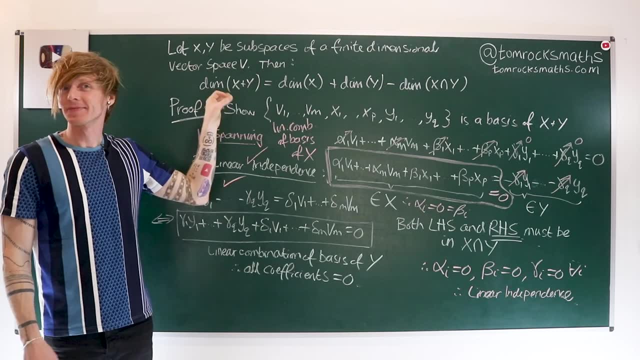 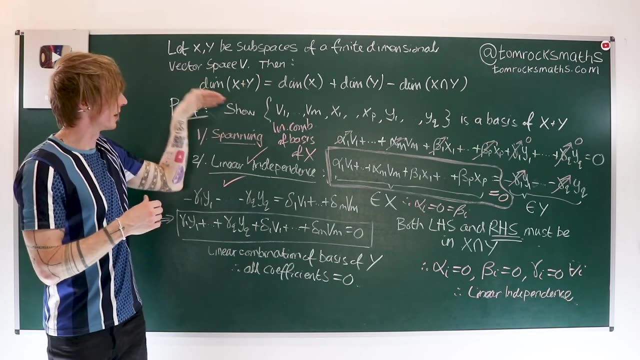 to be true, we can go back to my earlier working and we can indeed conclude that the dimension formula at the top of the board is correct because, remember, earlier on I said this would be true and follows immediately, provided we could show that this collection of vectors of the 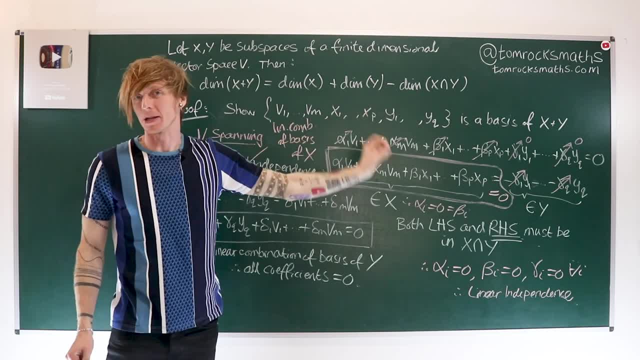 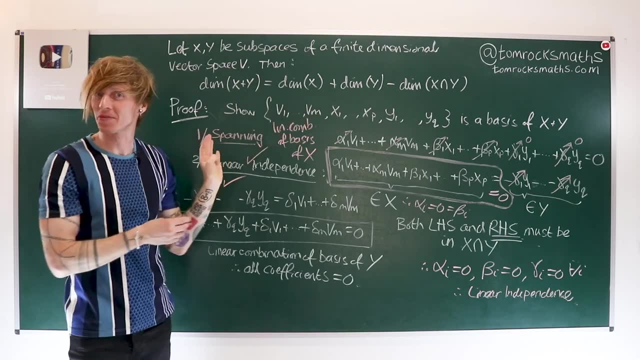 v's, the x's and the y's was a basis of x plus y. So we've just spent a big chunk of time showing that and, as you can see, that is actually the bulk of this entire proof, because once we have this, the formula immediately. 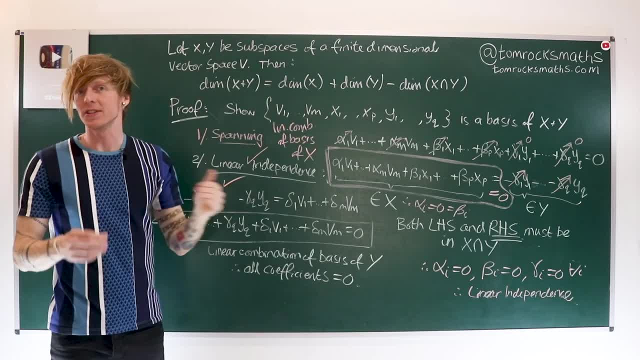 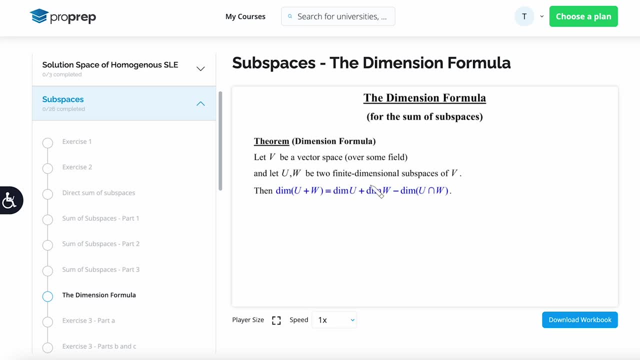 drops out, and that is our proof of the dimension formula. Now that we have our proof, it's time to put the formula into practice by heading over to ProPrep and having a go at some of the exercises on the dimension formula. The first few questions ask you to: 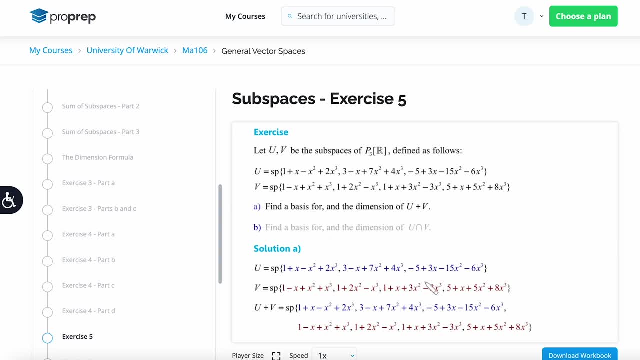 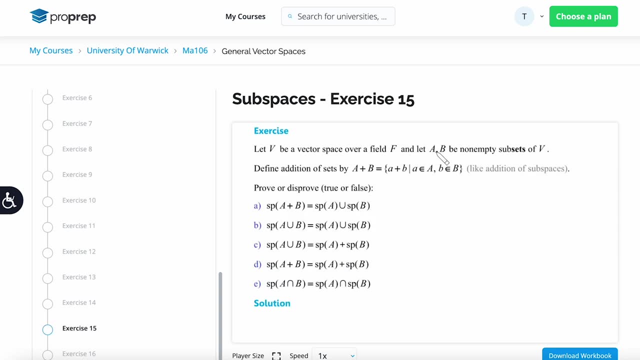 verify the formula for systems of linear equations before moving on to vector spaces of polynomials and even some questions on matrices. And if you really want to test yourself, there are some proof questions later on for more abstract spaces and one where you have to check whether the given statements 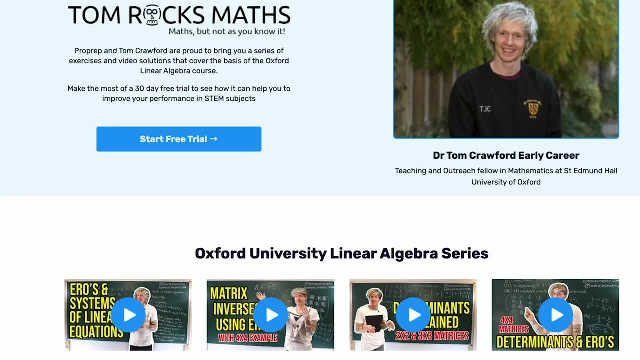 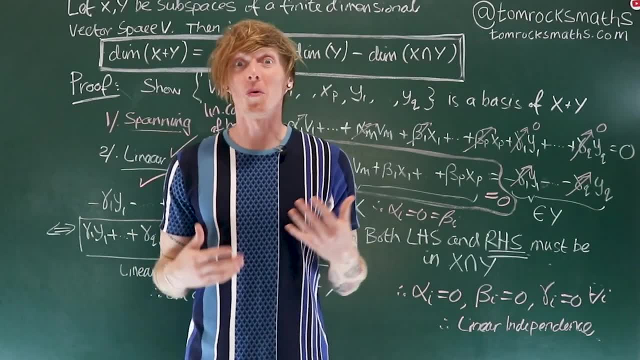 are true or false. Remember to sign up by clicking the link below to get your 30 day free trial of ProPrep, courtesy of Tom Rocks Maths. Thank you everyone for watching. Please do remember to subscribe to the channel if you've enjoyed the video, and I'll see you all. very soon Take care.